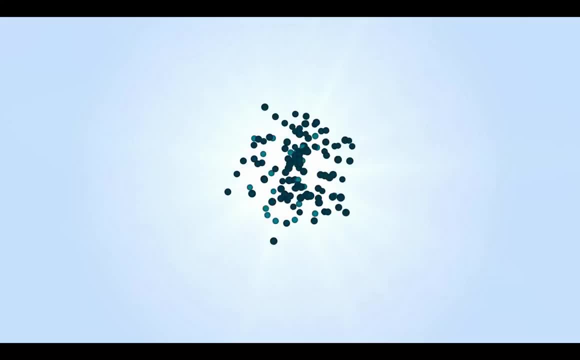 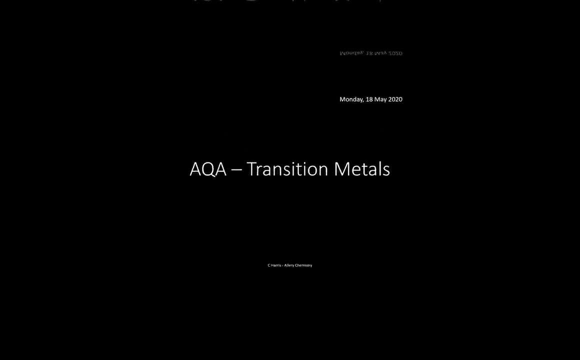 Hello, my name is Chris Harris and I'm from Allery Chemistry, and welcome to this video on transition metals. So this is specifically designed for AQA, so if you're studying AQA chemistry, then this video is absolutely perfect for you. so it has everything that you need to know for AQA and nothing more. In fact, it's. 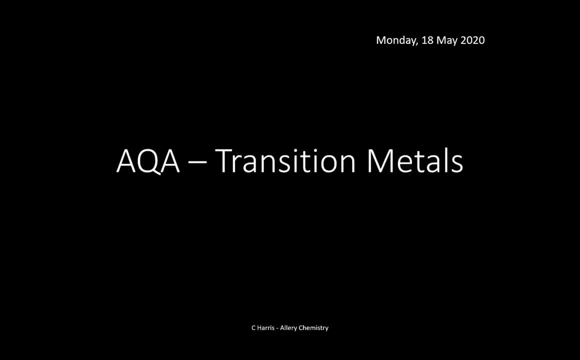 been designed around the specifications so you can have the confidence that actually anything in here is going to be relevant to AQA and that you don't need to worry about if it's in the, if it's in the actual exam paper or if it's on the spec. everything in here is dedicated to AQA. Now we have a full 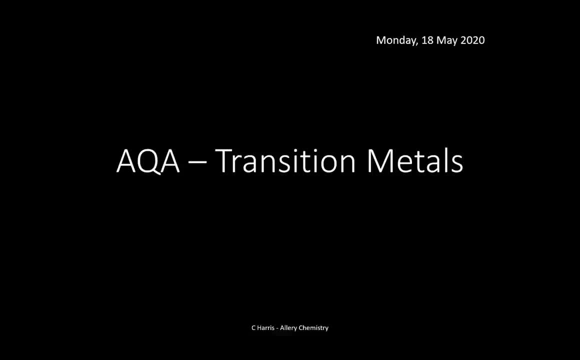 range of AQA videos for year one and year two chemistry on my Allery Chemistry YouTube channel and there's loads of revision videos like this. I've also done whiteboard tutorials as well and which look into specific concepts in chemistry, and I've also done some exam paper past some past paper. 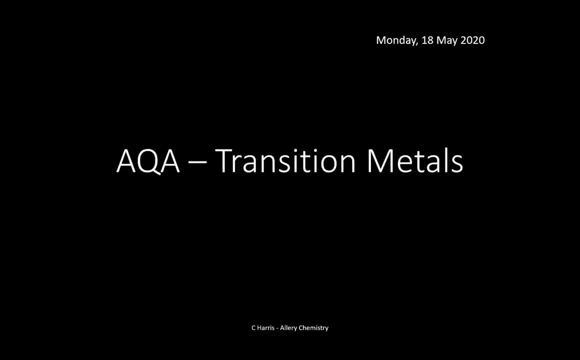 walkthroughs as well, and they're all for free. that all I ask is that you hit the subscribe button, and that would be fantastic Just to show your support for the channel. as long as people keep subscribing and watching, I'll keep making these videos and updating them and refreshing them and coming up with 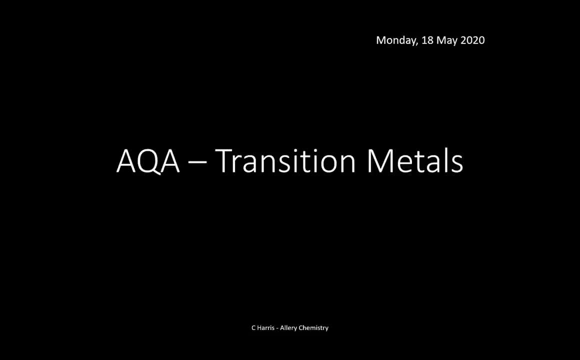 new content, etc. So please hit the subscribe button. That would be, that be great. and if you would like a copy of these, this is, these are powerpoint slides, So if you'd like a copy, there's your money, is yours- copy of these, and then you can purchase them by clicking on the link in the description box below. 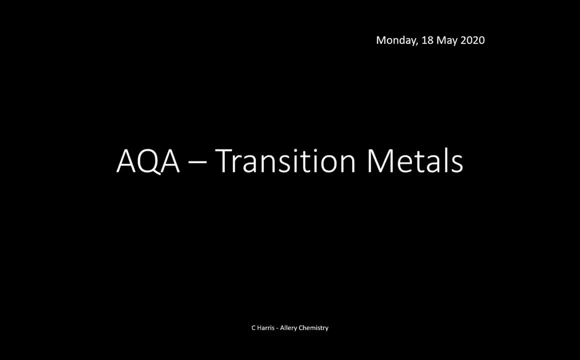 and the great value for money and the full range is there and you can use them on your smartphone, your tablet, use them as and when you require, and also I know people to print them off, for example, and use them as revision notes. so they are, and the full range for AQA is is on there as well. so 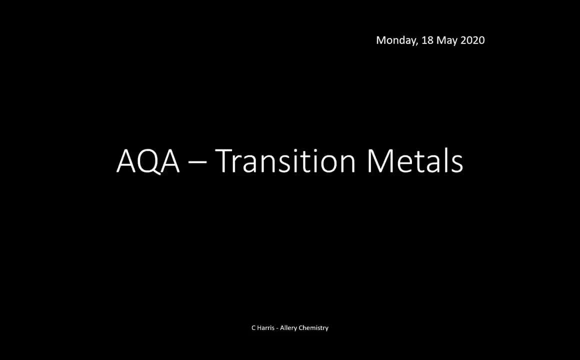 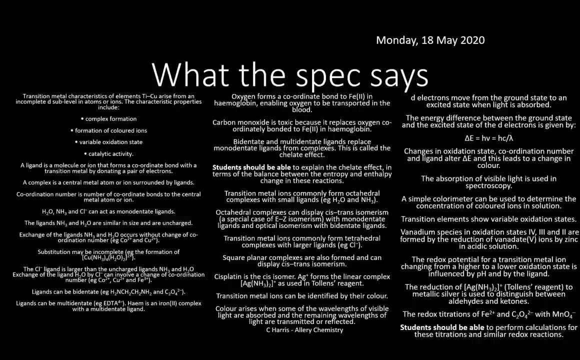 so they are available to purchase. just click on the link below and you can get a hold of them there. okay, so, like I say, this is dedicated to AQA and the specification is listed there. so we're going to look at things basically in this video. we're going to be looking at transition. 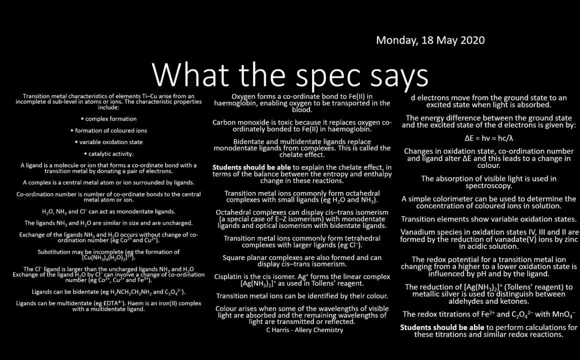 metal complexes and we're going to be looking at ligands. we're going to be looking at EZ isomerism within these complexes. we're going to be looking at hemoglobin- there's a lot in this one. we're going to look at how color is actually derived from these transition metals and look at some. 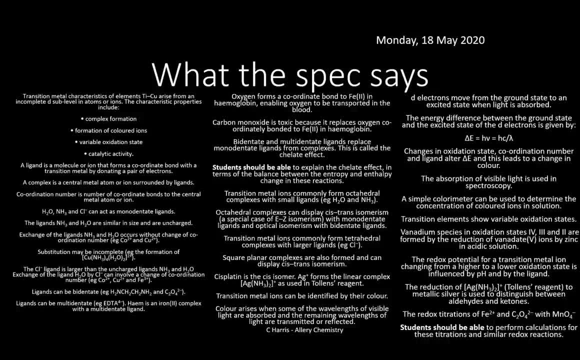 � particular aspect of chemistry including vanadium which is a lovely element of chemistry lovely element well it is an element yeah it's a lovely part of chemistry so we are going to be looking at vanadium as well and also we're going to be looking at catalysts so homogeneous and 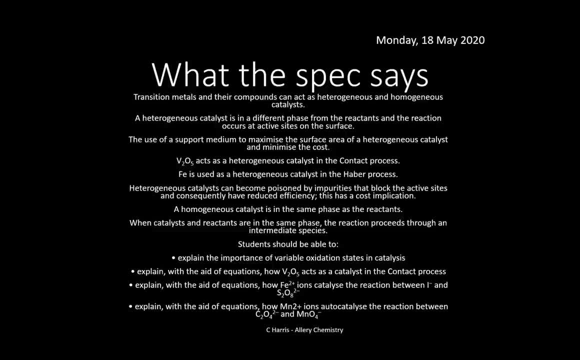 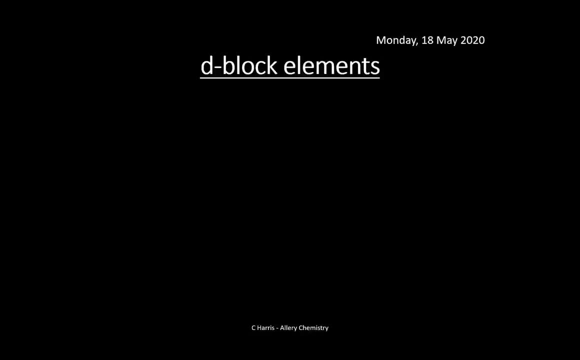 heterogeneous catalysts and autocatalysis, which is the bit at the bottom. so that's the general order of this video. so it does match the specification, okay, so let's have a look and start with d block elements, and we need to know where these d block elements are because let's 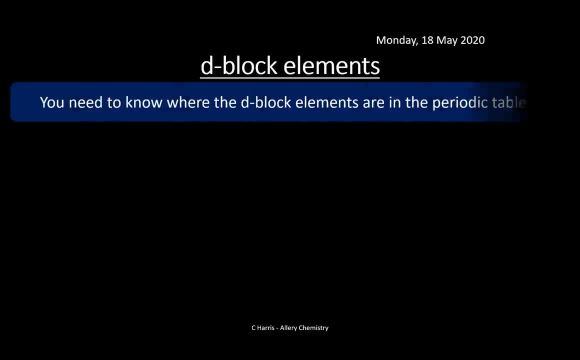 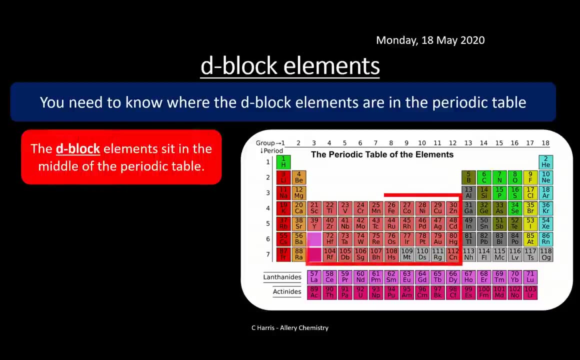 be honest, everything in this video is going to hinge around this, this slide, okay- and these types of elements. so the d block elements of the periodic table are actually the ones that are in the middle there, highlighted in that box. so these are your d block elements and some of these are. 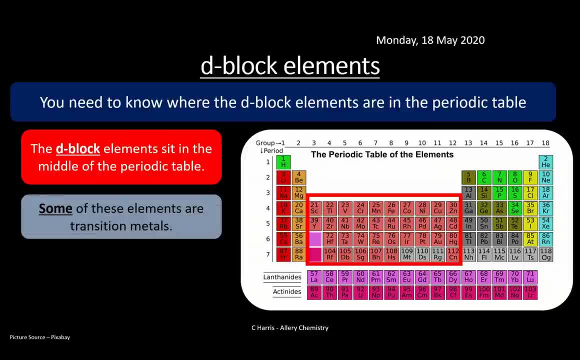 transition metals- not all of them, but some of them are, and the ones that we need to know are the ones on the top row of the transition metal block. there you, so they're the ones from scandium to zinc. you can see on the top row there. so there, it is okay. so 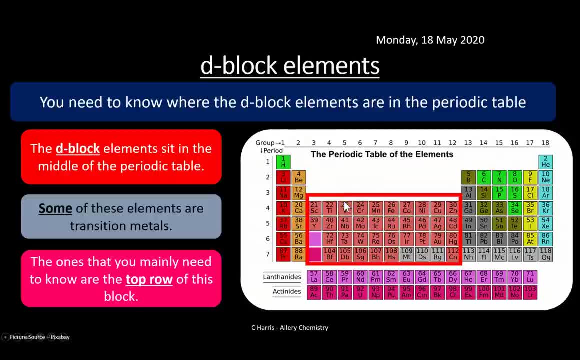 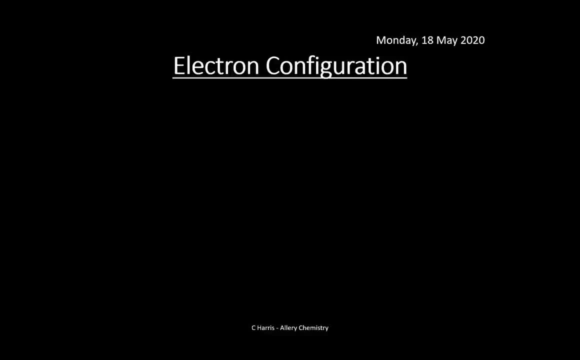 from scandium all the way across to zinc. so these are the ones that you need to know. okay, right, so so let's look at electron configuration, because we're talking about transition metals and so therefore, they have unique. their main properties, or the unique properties of transition metals is: 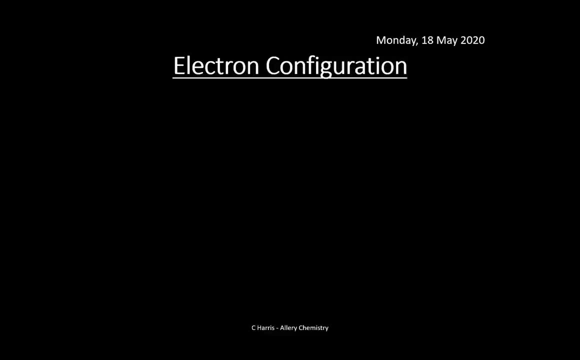 all down to do, or is mainly to do with the electron configuration of these elements, and so, therefore, we need to know, we need to know the way of doing this or we're going to do this. the way that we want to do this is we need to know a lot of information about this. so we're going to start, let's say, by looking at how the electric configuration 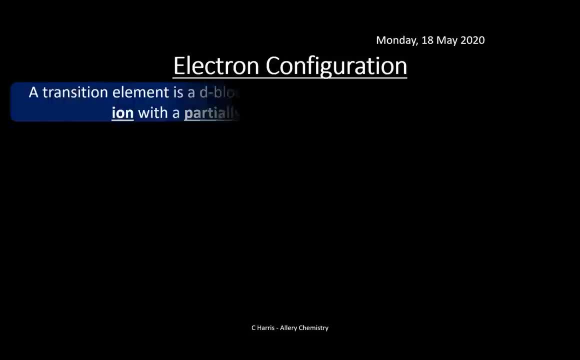 And all of the looking at the electrical configuration of transition metals. so a transition element is a d block, elements that can form at least one stable iron with a partially filled or incomplete d subshell. okay, that's very, very important. so I'm a member of the sub shell and you might have seen this before, but you should have done in your one chemistry when you look to electron. 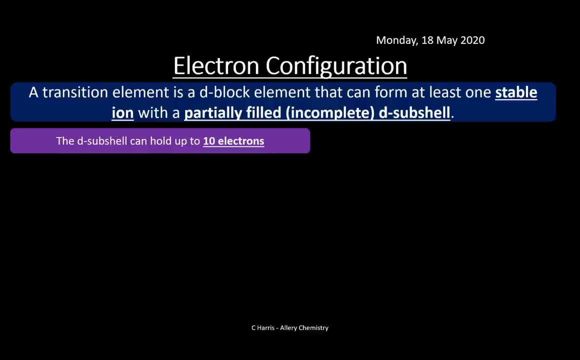 orbitals and that the sub show shell can hold up to 10 electrons in the d sub shell. okay, so remember, for a transition metal, and it must have a stable ion that has a partially filled d sub shell. okay, or what's incomplete. so, um, you can see that for period four d block elements, only eight of these are actually. 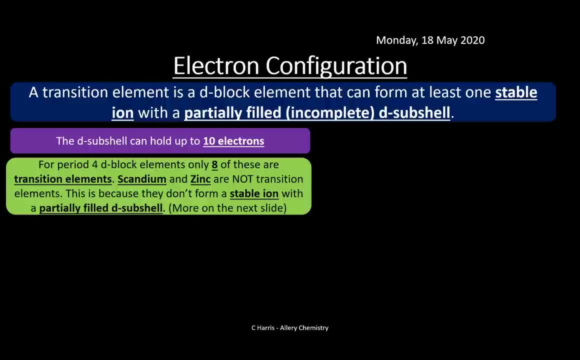 transition elements, so scandium and zinc. so these are the ones that flank the sides of the um, the first row of the transition elements. um, these are not transition elements because they actually don't form a stable ion very important to the stable ion that has a partially filled d sub shell. 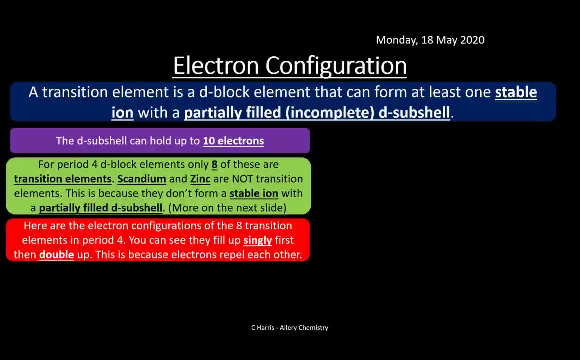 okay, um. so here the electric configurations of um eight transition elements in period four, and what we're going to see is we're going to see them filling up singly first, then they'll double up. now it's like i like to kind of um be using an outlet. well, not analogy, but i suppose. 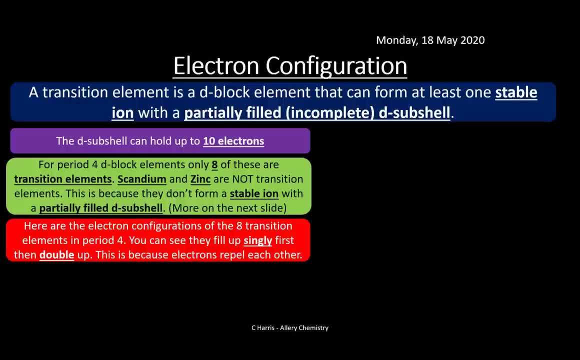 a life experience. i think i'm going to call it um, be using life experience sometimes when you might. you might notice this as well, but when you get on a bus, um, you have seats, obviously you have seats um, and let's imagine you have um, um half the seats are somebody sitting in the seat and half. 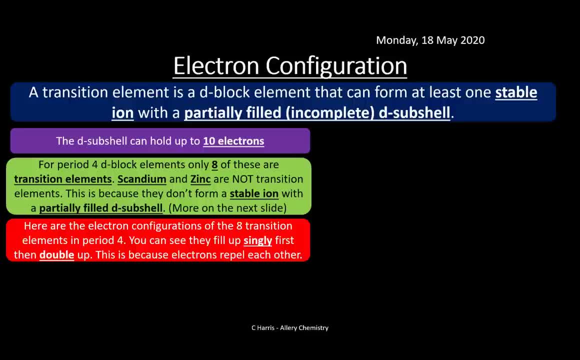 them are not. now. when somebody gets on the bus, they are more likely to go and sit on a seat on their own than go and sit next to somebody else. okay, and that will continue to happen until all actually have have at least one person sitting on them and then, when somebody else comes on, the 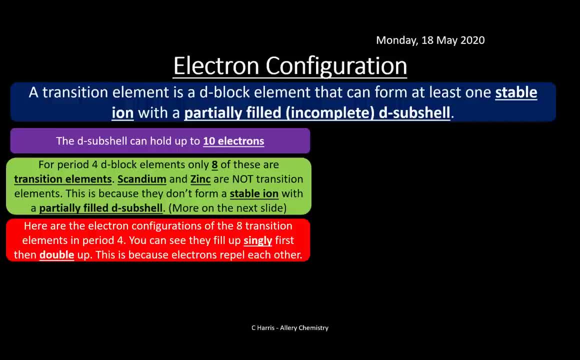 bus afterwards. what you normally find um is: uh, some people just stand um and some people will, but they have to. if they want a seat, they're gonna have to sit next to somebody. but it's just funny because it's this reluctance to sit next to somebody. i suppose it's that you're having your. 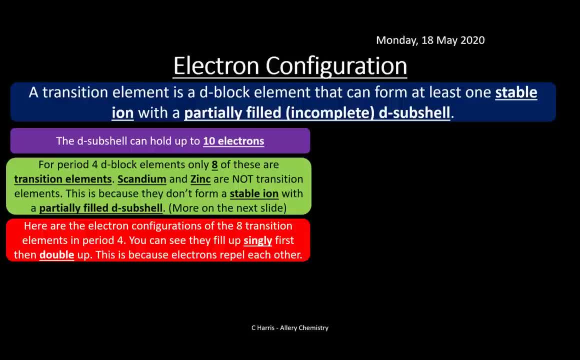 own space, that bit of kind of you know privacy, um, you know so things like that. so but yeah, but electrons are exactly the same actually, you know they, they will only go in an orbital if it's, and only if they absolutely have to will they actually double up, and that means if it's lower. 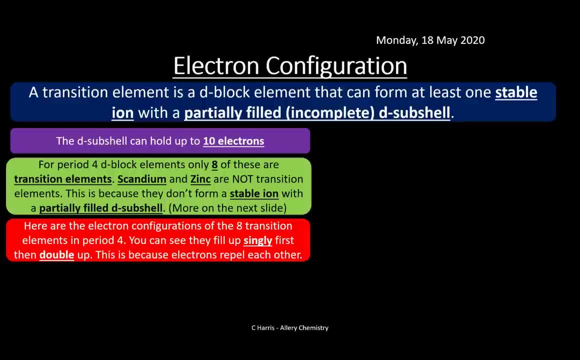 energy generally with with atoms because, as you know, if you've seen my other videos, um you know atoms and ions and electrons and atom um protons, etc. they all want to be in the lowest energy possible. they're incredibly lazy um- and you'll see this already- really lazy and um that they uh. 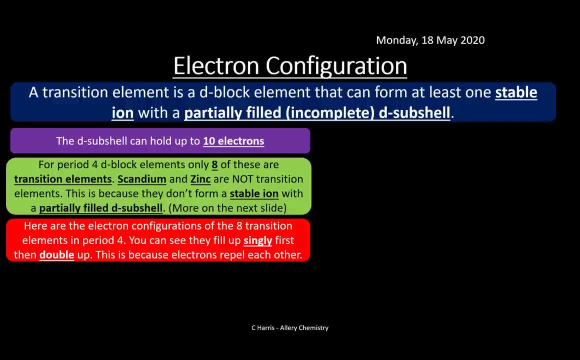 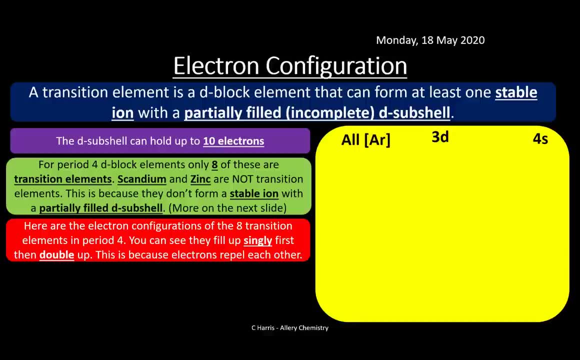 they always want to be in the lowest energy state. so this is kind of where it's, where it stems from. let's have a look at some of these, then let's let's move on to this. so when we're doing electric configurations, you'll notice i'm going to use um, all of the configurations i'm going to give start. 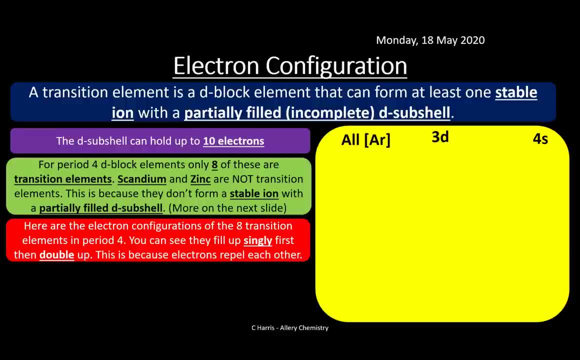 with um, ar in square brackets, and you might have seen this, and all this means is just the electrical configuration of argon, so it stops me from writing out the full electrical configuration for all these transition elements. so, remember, the electrical configuration of argon m is 1s2, 2s2, 2p6. 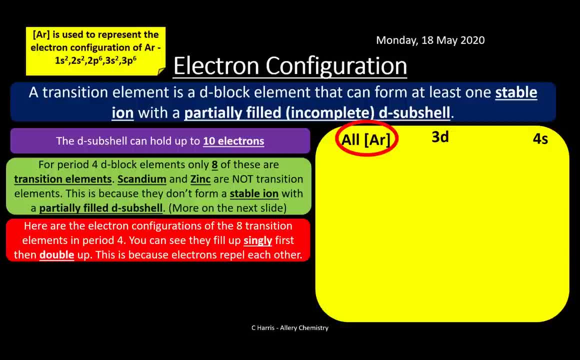 and then the electrical configuration. is that plus what you're going to see on here? so we're going to start looking, going across the transition elements. so we're going to start with titanium first. titanium has um four electrons. this is for the remember, this is for the transition metal. 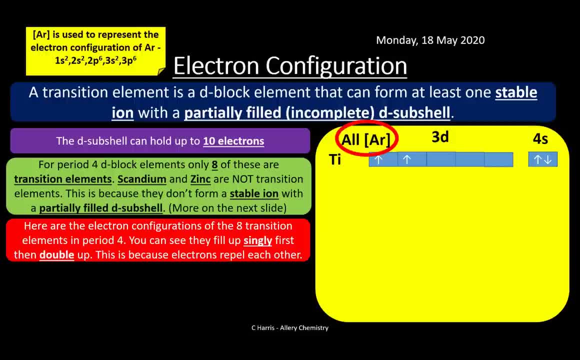 um, elements, not ions. okay, so this is just the elements. so it has two electrons in 3d and two in the forest, so it's got four, four valent electrons effectively. okay, um, and then vanadium has the extra electron in the 3d orbital, so that's fine. 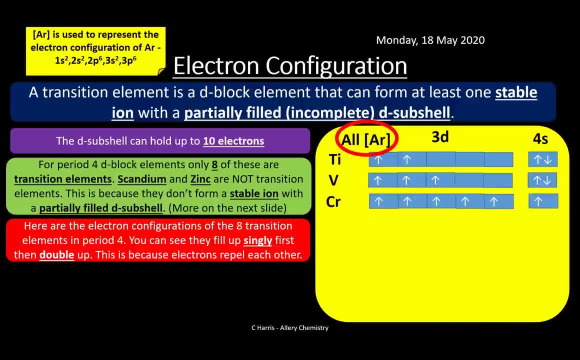 um, and then chromium has something a little bit strange. what happens with chromium is one of the elements, or one of the elements, one of the electrons in the 4s orbital jumps down into the lower orbital here, and the reason why is this half full configuration these. 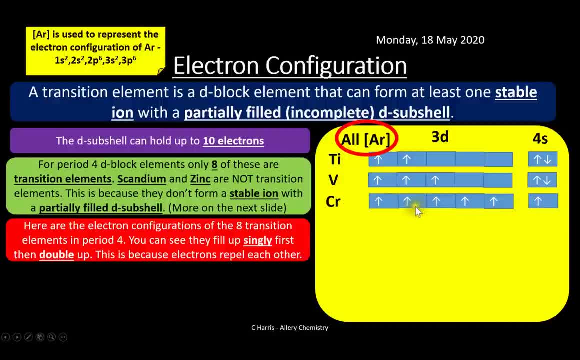 are like seats on the bus. this half full configuration is actually really stable. it's more stable than having the fourth electron and the other electron paired up there. remember, electrons really don't like sitting next to each other. so it will do this, chromium will do this. um, you know what? 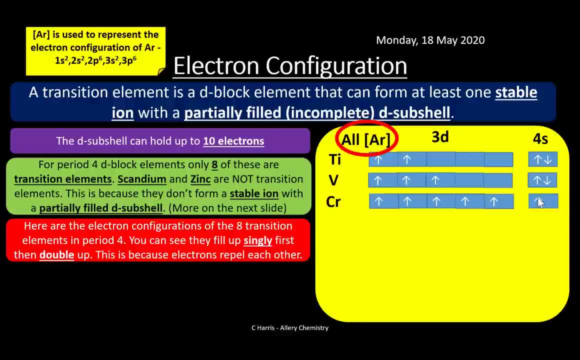 this element. so just be really careful for chromium. there's another one coming up as well, um later. which? um? where's another where it behaves like that as well? so let's have a look at manganese, which is the next one. now the electron for manganese then sits into that, goes into the 4s. 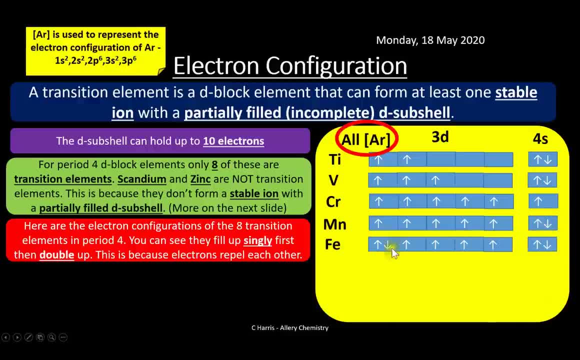 orbital um, and then iron is obviously. that electron goes there for iron, the next one's cobalt, and so cobalt has the extra electron in there, okay, which is absolutely fine. and and then we've got the extra electron goes in there, and then copper is the other dodgy one. so the electron then decides: 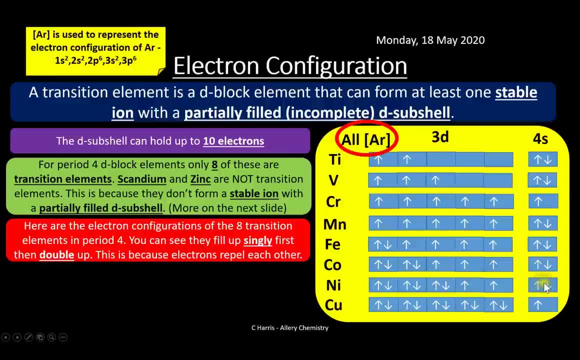 again to jump from here. so the normal electron goes in that orbital, but this electron jumps into this one here again. this is more stable because we have a full 3d subshell here, whereas whereas with this one with manganese it was a part filled d subshell and that is. that's a stable setup there. 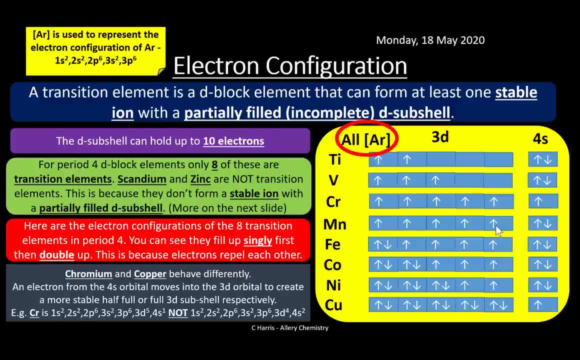 so you can see that chromium and copper, these behave differently. so an electron moves from the elements into the 3d to create a more stable half full or full 3d subshell. so just to make sure that when you're given the electron configuration of um, your transition elements, as you can see on 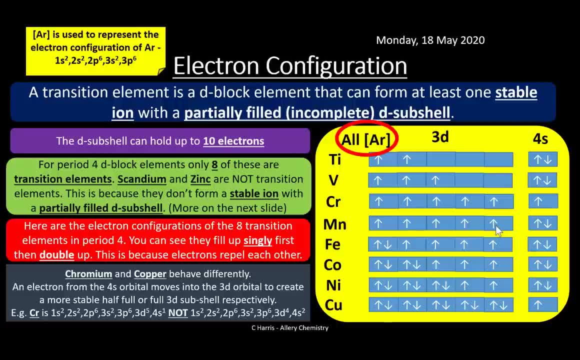 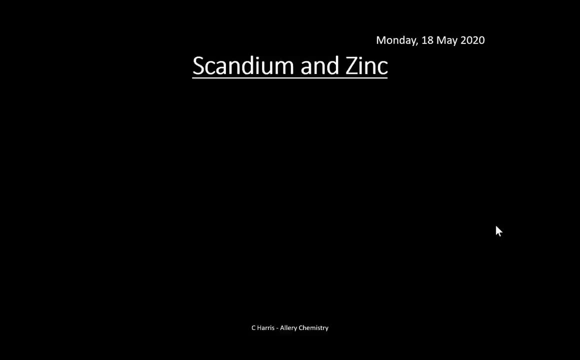 there that they're actually- um, you know that you're actually giving them correctly, particularly for chromium and copper. so don't forget that, because the bottom dollar, the exam board, are going to ask for the electric configuration of them elements, because they're a little bit different. okay, so we're going to look at two, remember two- of the elements here. 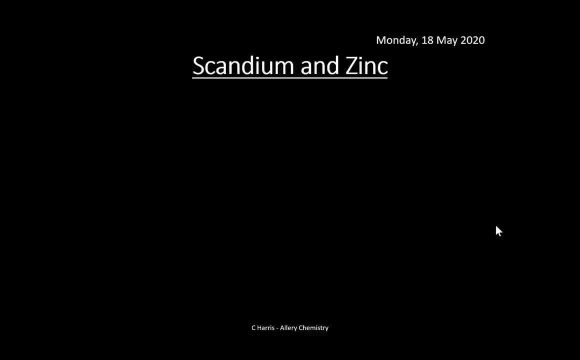 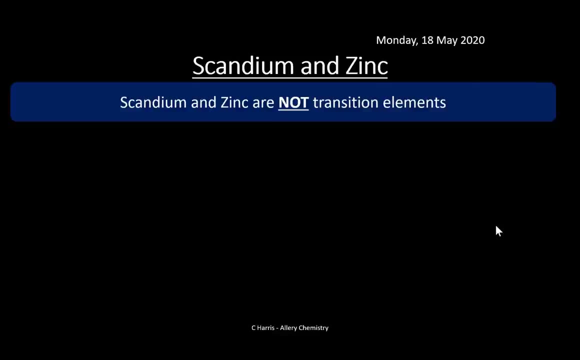 that we've seen before and we said that actually these elements are not transition. uh, these are not uh transition elements, but they are d block elements. so remember um, which is scandium and zinc. so we're going to look at a little bit more information about why these are not transition. 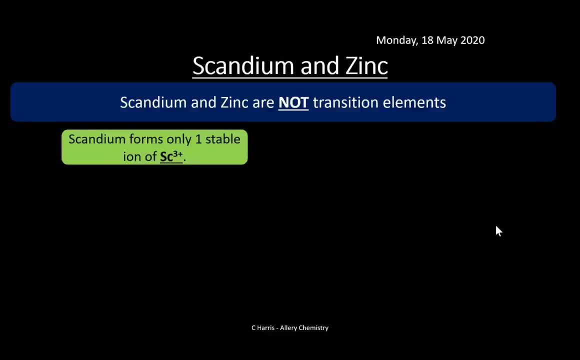 elements. so we start with scandium. scandium only has one stable iron, which is scandium 3 plus. okay, now if we look at the configuration of scandium, it has an empty d subshell, so it's not partially filled d subshell. so it's going to be a partially filled d subshell, and that's because the scandium 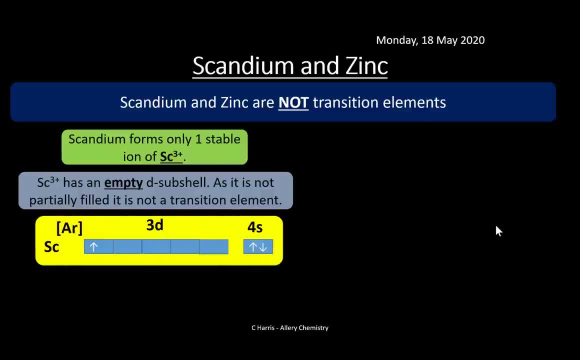 ion has got a partially filled. sorry, it doesn't have a partially filled d subshell. it is not a transition element. so if we have a look here, that's scandium atom. okay, that's you might think. hang on, that's got a partially filled d subshell. but remember the definition: it's the ion, that's. 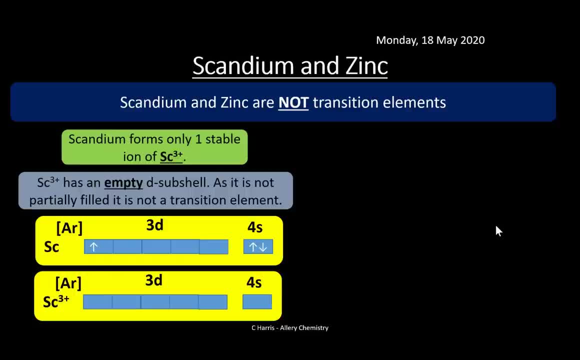 got a partially filled d subshell. so the iron, the only stable iron scandium forms, is scandium 3 plus and you can see there that there is absolutely no um filled. so therefore it isn't a transition element and you'll see a little bit more on that later. 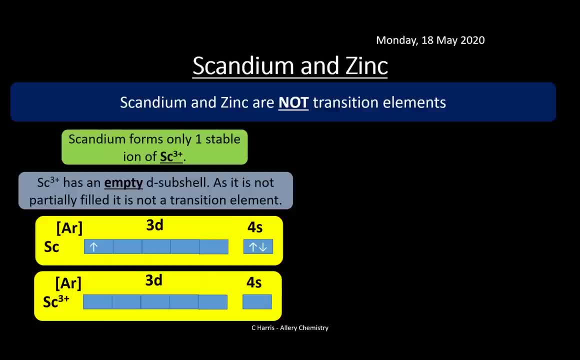 when we look at um, when we look at um color, for example, because transition metals are generally most, vast majority of them are colorful. the ones that aren't um are not colorful. i remember the other one was zinc um. zinc only forms one stable iron, which is zinc two plus um. now zinc two plus. 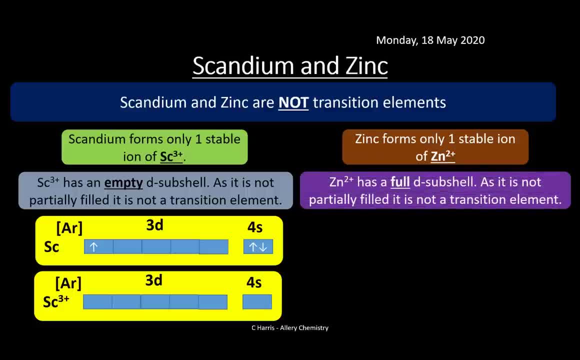 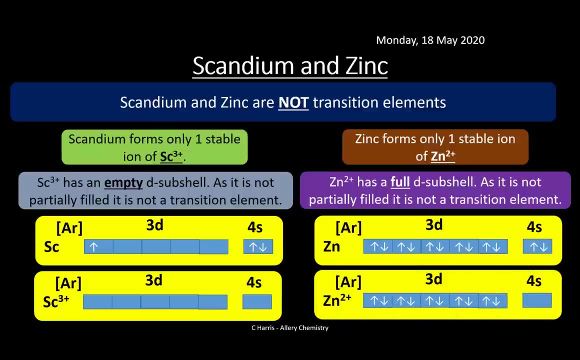 has a full d subshell, um it's not partially filled. so let's have a look at zinc atom first. so zinc atom has a full d subshell, but the ion, which is zinc two plus um- actually you'll see a little bit more on this um later- but the electrons- when we're removing electrons to form an iron. 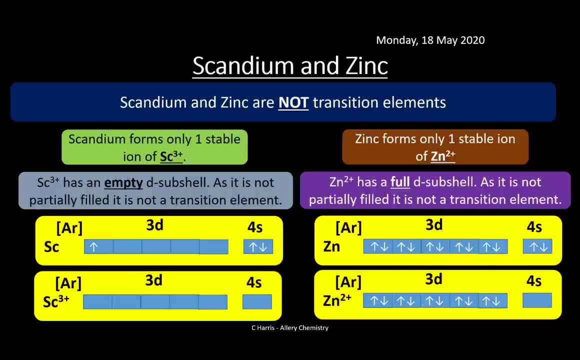 they are removed from the 4s orbital first, then the 3d. so because zinc two plus has lost two electrons, it loses them in the 4s. it still has a full 3d subshell. so therefore is not a transition element. okay, so this is what we're actually going. 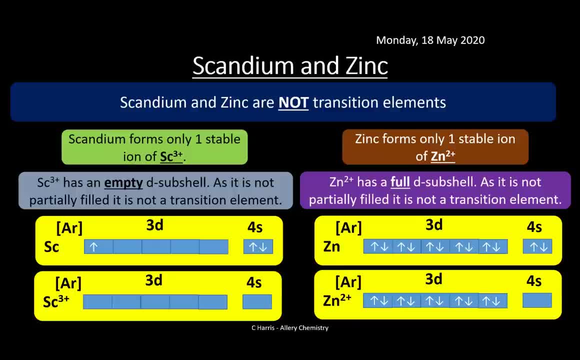 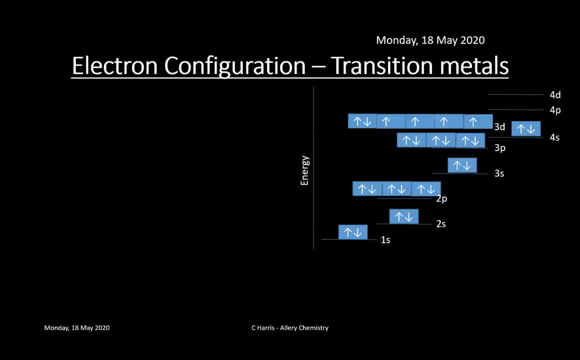 to look at. we've looked at the the 4s. they're losing the electrons of the forest first when we're when we're ionizing a transition element. so we're going to look at that in a little bit more detail by using this electron um electroconfiguration diagram. okay, so we can see. 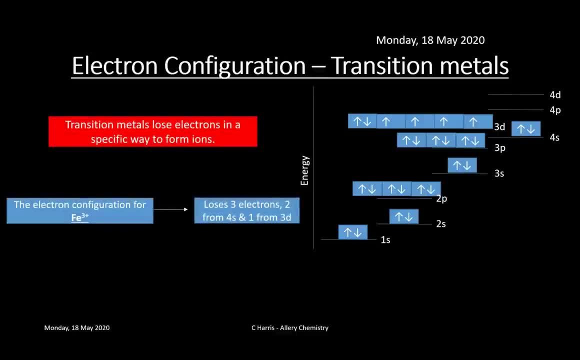 this one. here we're going to be looking at iron. okay, and they lose electrons in the specific ways we've seen before. so looking at iron. so this is the electric configuration of lithium and from iron 3 plus, this loses three electrons to form iron 3 plus. so two from the 4s and one from. 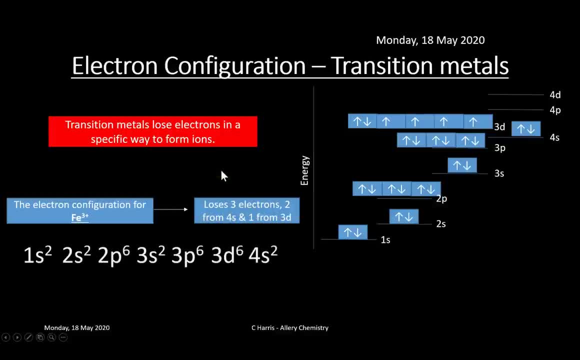 the 3ds, remember it loses from the 4s first. so let's have a look at the configuration. so there's the configuration of iron 1s2, 2s2, 2p6, 3s2, 3p6, 3d6, 4s2. okay, so that's the electric configuration. 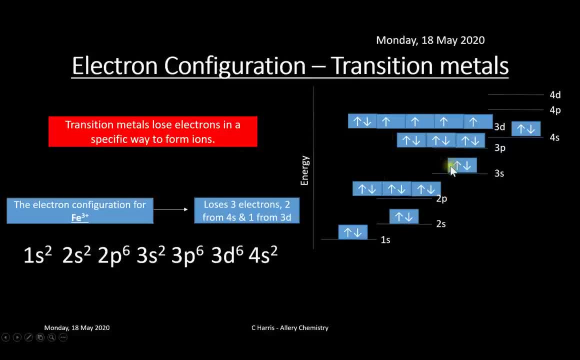 for iron and that is the actual energy diagram, as you can see there. okay, so if we then ionize this, okay, and we turn it into a fe3 plus, then we lose the electrons. if i just go back and you can see it there. so that was the configuration of iron, and iron 3 plus means we 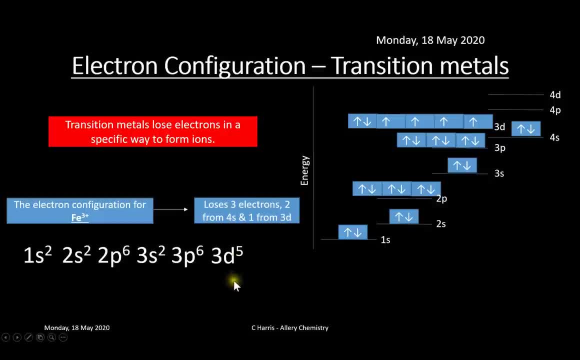 lose them electrons and we end up with a 3d5. okay, so what we should do is always check, check the numbers. so the um, the number of electrons in iron, standard iron metal, is 26. but we're losing the electrons, so we're losing the electrons, so we're losing the electrons, so we're losing. 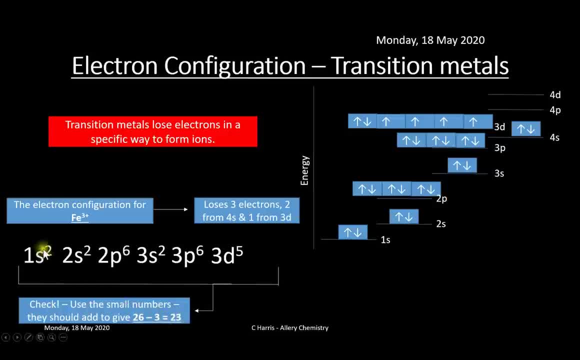 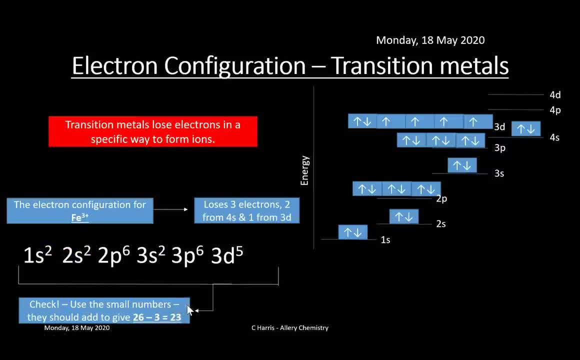 come to 23. okay, so we're then going to apply that into our diagram. so let's have a look here. so we're going to lose to the 4s first and then the 3d. there we are, and then the 3d, and that is the. 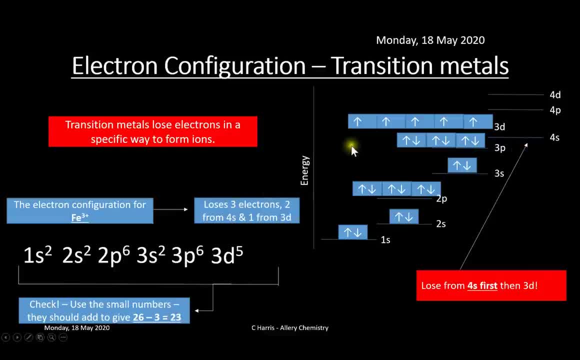 electrical configuration of iron iron 3 plus. so you can see that iron 3 plus does have a partially filled 3d sub shell or d sub shell. so therefore, is a transition metal. okay, so you've got to remember that. you've got to remember um in terms 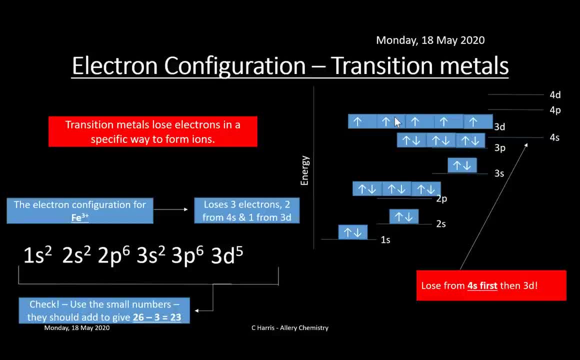 of um the electrical configurations of the elemental, of the, of the elements, the transition elements, but also, how do we then um write the electrical configuration for the irons, because they, you know there is, they are removed in a particular way, as you can see. okay, so we've looked at the kind of the properties in terms of an from an atomic. 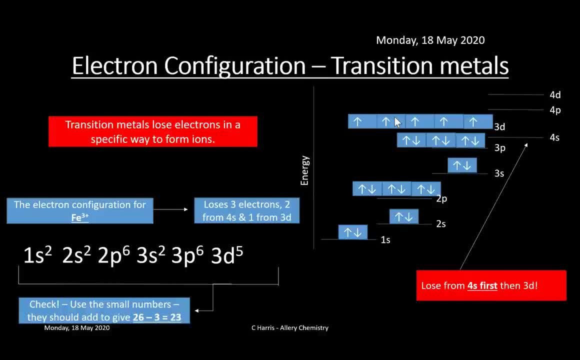 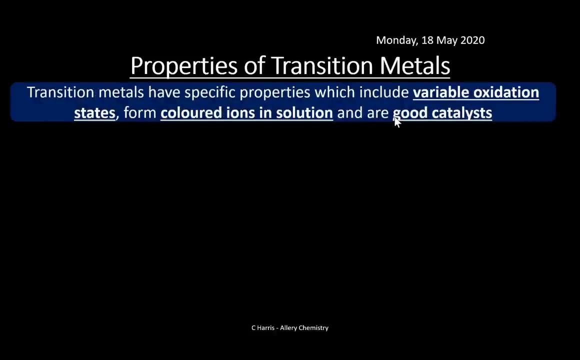 level of transition elements, so the electrical configuration, because it is critical for that. so now we're going to look at their properties, in other words, what can we observe or what can we do with them, practically okay. so properties of transition, uh, properties of transition metals. so transition metals have specific properties and this, this is such as, or these are such as: 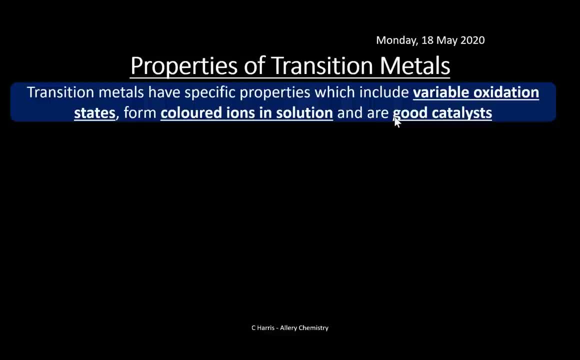 variable oxidation states. they form colored irons and solutions and they're good catalysts and we're going to look at all the way through the video. we're going to look at the various properties of these transition metals. i love this topic. it's really good. it's not easy. it's not an easy topic but, um, i like it because it's all colorful. it's the most. 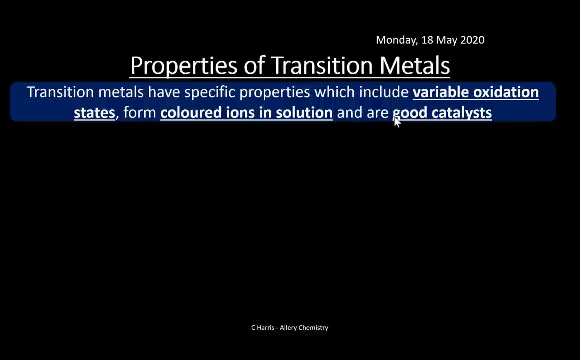 colorful area of chemistry and it's often kind of just thrown to one side because you know you often kind of well, you either look at the physical side, which is the mathematical side- some people love that- or you look at the organic side, um, you know, which is quite a big part of chemistry. so 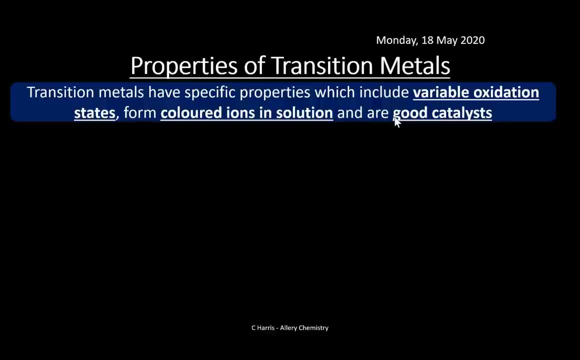 there isn't much on it in organic chemistry in at a level so um. so when it does come around, i i quite enjoy it. so there we are. that's the. that's the bit that i particularly like because of the colors. so transition metals have variable oxidation states and this is because the electrons remember. 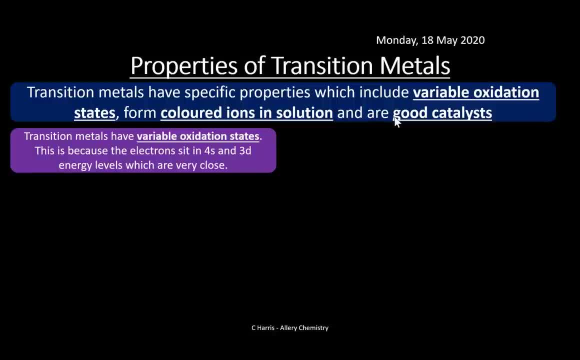 when we looked at a diagram, they sit in the 4s and the 3d um orbitals and these orbitals are actually really really close in energy and it's this closeness and energy of these orbitals that give transition metals the properties that we see um what we see um around us, so, um, as a result, what 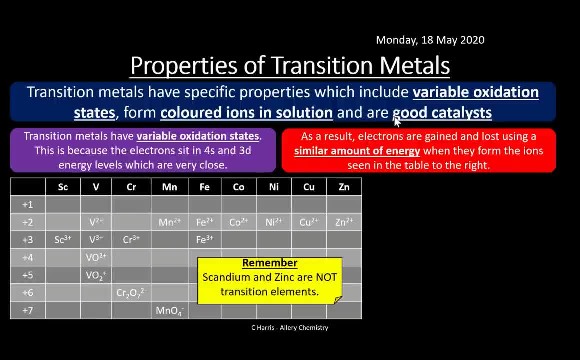 they do, um is they form a variety of different ions. okay, and they um the electrons are gained and used in a similar amount of energy. okay, when, whether we take it from a 3d or 4s, um, as we um, you know, as we remove the electrons from them, and so, therefore, they can form a variety of different. 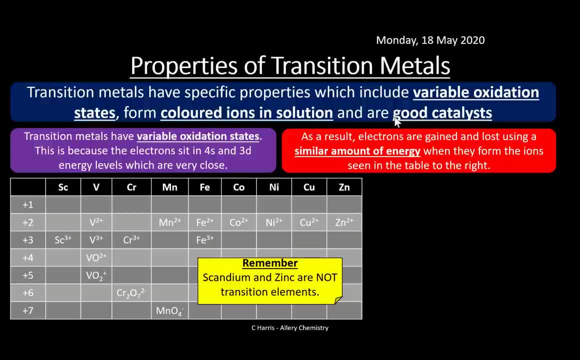 ions. as you can see- and here there are some various different examples here of different ions and unlike, say, group ones and group twos. where group ones will form plus one ions, group twos will form plus twos and that's pretty much it. transition metals form a variety of different. 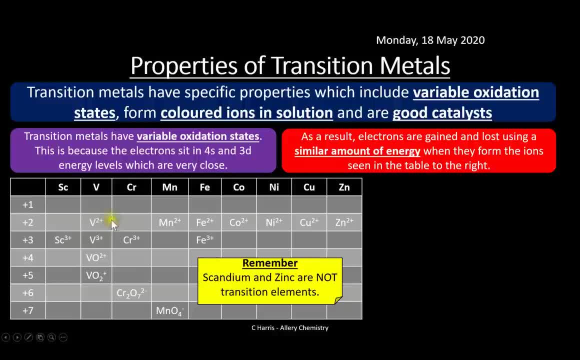 ones, particularly vanadium, and you're going to look at vanadium chemistry later on. but vanadium has loads of different oxidation states, loads of different colors as well. um, chromium, obviously got your chromium compounds, manganese there as well, iron, cobalt, nickel, copper and zinc. so remember zinc and scandium here on the side are not transition. 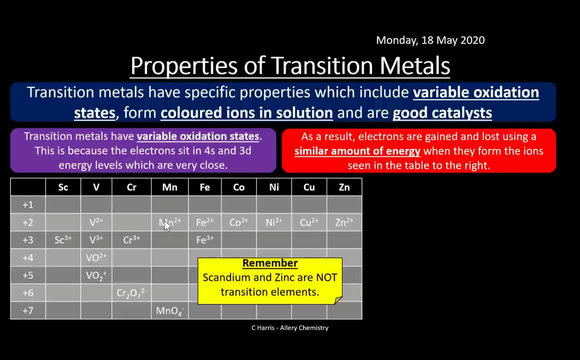 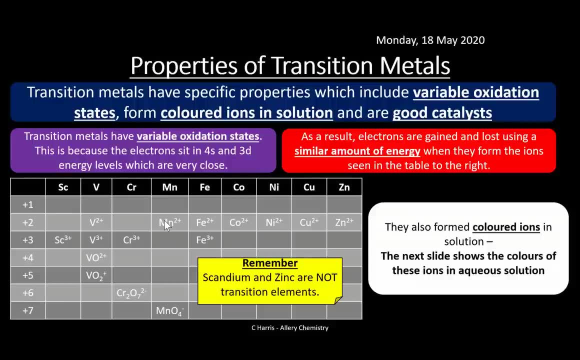 elements. they do, they are d block elements, but they're not transition. they're not actually transition elements. okay, so they also form um colored ions in solution and we're going to look- actually we're not going to look at this- in the next, uh, the, the, the next slide. I suppose you're. 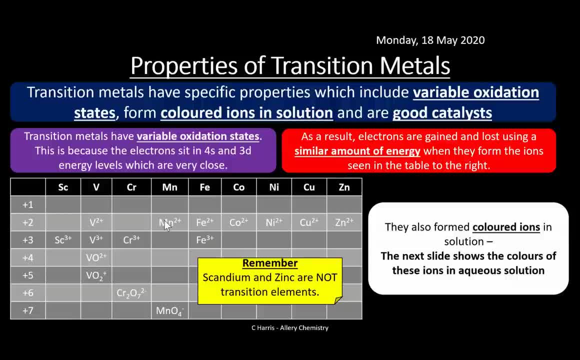 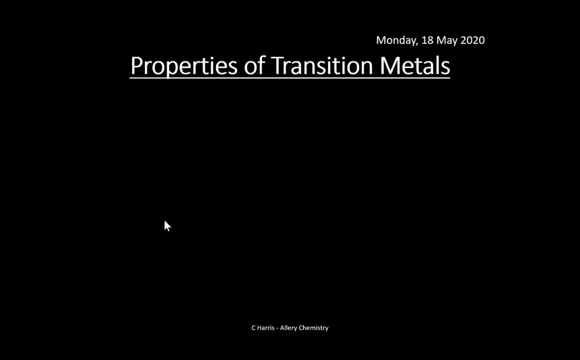 going to look at this in a little bit more detail on the next topic. that's what it should say: okay so, looking at the in aqueous ions, the colors of these, okay so, um, so we are going to look at, um, we are going to look at the, the colors here, but not actually the actual complex, which is which is going. 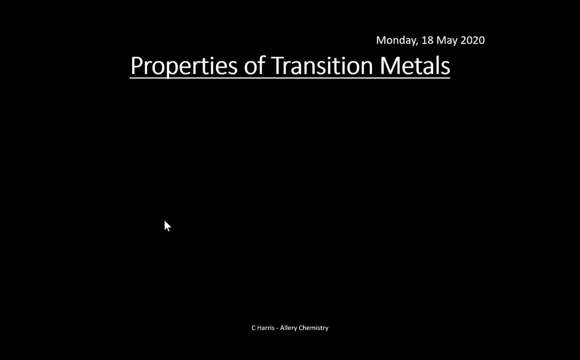 to be in the next topic. that's what I mean, you'll. you'll see what I mean. so we're just going to look at, you know, the reactions with hydroxide pneumonia. we'll look at that in the next topic. you'll see what I mean. I'm going to shut up and just get with it right. so transition metals, they have specific. 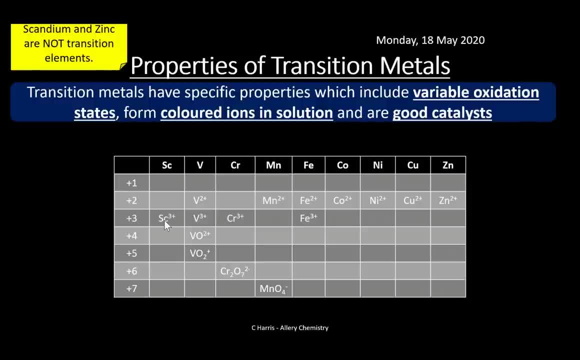 properties. um, like I say, one of them is colored solutions. remember, scandium and zinc are not transition elements and you can see here we've brought our table back up again. so we're going to look at the colors of these and when they are dissolved in water, and just look at the colors. 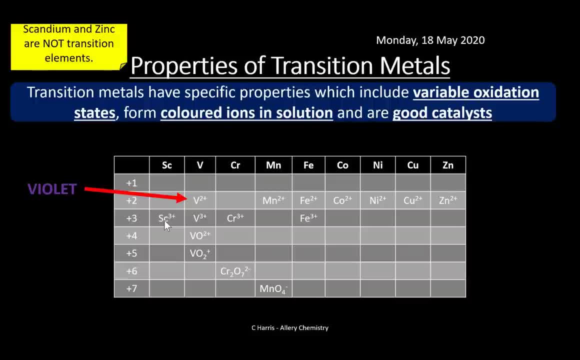 like I say, the actual structure is going to be in the next topic. so, um the vanadium 2 plus is violet, vanadium 3 plus is green, um vo2 plus is blue and vo2 plus is yellow. don't get them too confused. um you know, make sure you're. 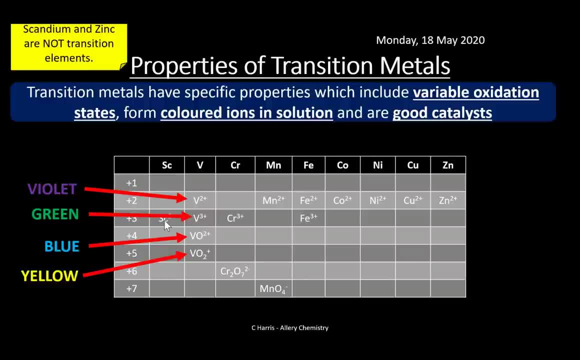 really clear with these, because there is a topic. well, there's a section in this video where we do look at vanadium chemistry. it is a requirement and for aqa. so it's really important that you differentiate between vo2 plus and vo2 plus um. okay, so your um. next one is chromium 3 plus now. 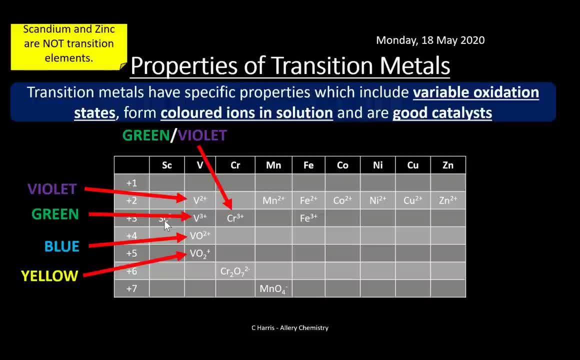 this one is greeny, a greeny violet. um, the reason why is actually it's violet when it's surrounded by six waters, um, but they're normally substituted with other things, so actually usually looks green, so it's a bit of a funny one. um, it's chromium 3 plus a dichromate is a lovely orange color, so that's nice. uh, your manganate 2. 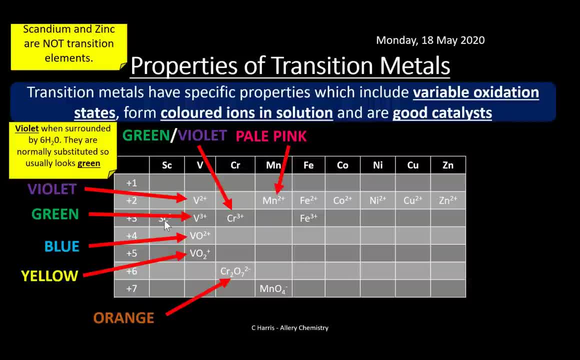 plus is a is a like a pink color, okay, um, and then your manganate. you would have seen this MNO4 minus pale green. it's a light green color, and iron 3 plus is rust, so that's an orangey, orangey, yellowy. 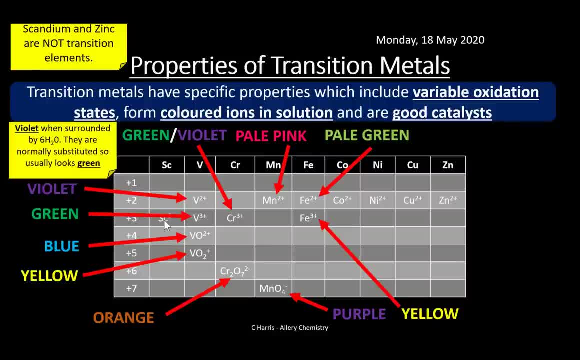 color um is is fe3 plus uh. cobalt 2 plus is pink. it's nice fuchsia, like a bright fuchsia pink. and nickel 2 plus forms green solutions. so nickel, nickel based solutions. and then copper 2 plus is blue, it's a nice pale blue and you might. you might have seen um, particularly if you made copper. 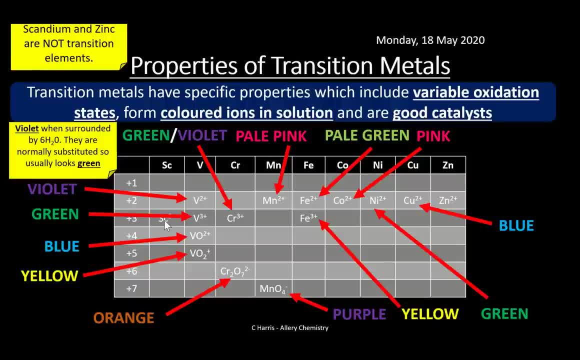 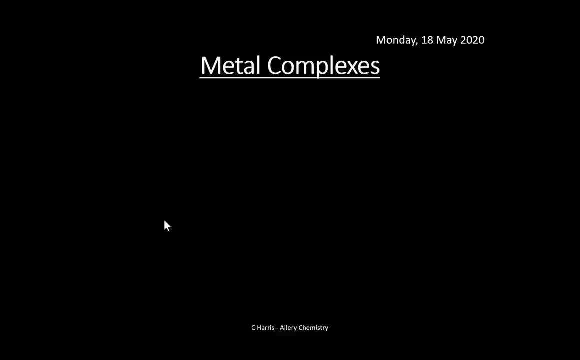 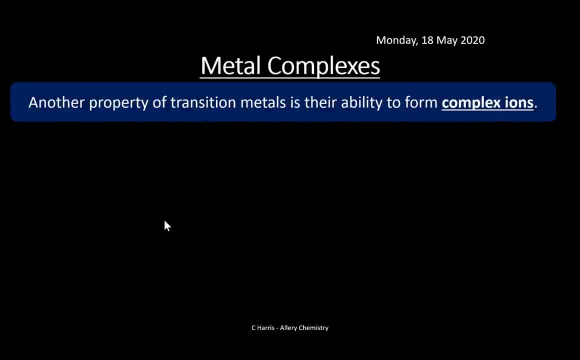 sulfate crystals. you get nice crystals there- um, so that's um. that's obviously quite, uh, quite important, okay. so looking at um some metal metal complexes here, so another property of transition Metals is their ability to form complex irons. okay, that's really really important. so what it does is it actually forms um. so when we have a transition metal in the middle and actually 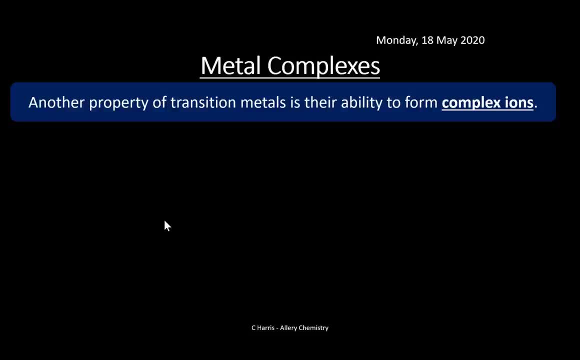 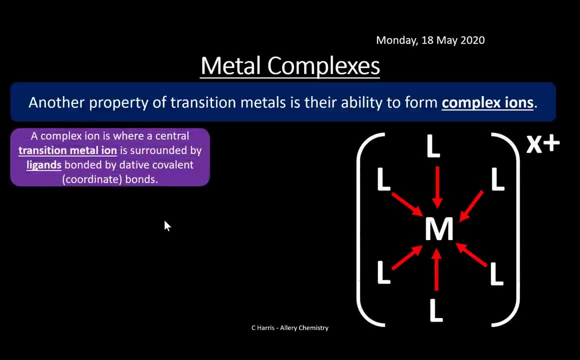 forms a big, large structure with loads of ligands surrounding that and that's obviously bonded, right, Mr, middle of the metal ion. okay, so a complex ion is where you've got a central transition metal ion is surrounded by ligands and it's bonded by dative, covalent or coordinate bonds. so you can see here: 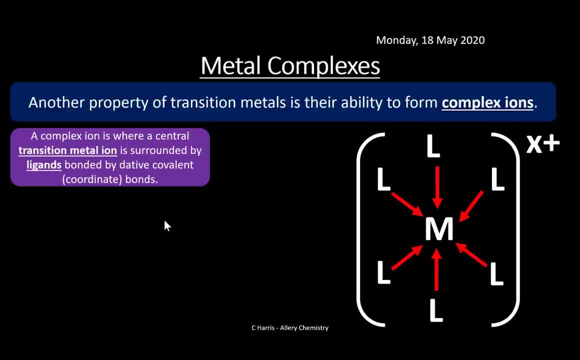 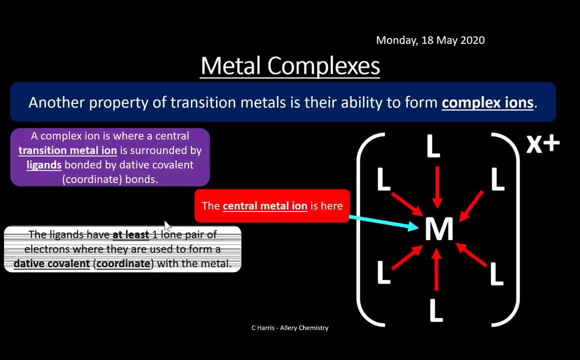 that we've got our complex- an example of a complex here- and the basic structure of it is that you have your central metal ion in the middle, so that's right in the middle there, and then we have some ligands, and so the ligands have at least one lone pair of electrons where they're used to form. 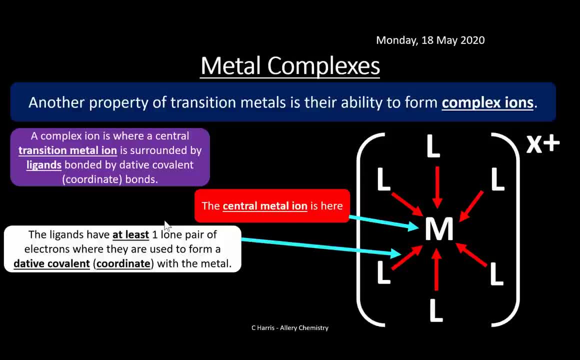 this dative covalent bond- remember, a coordinate bond- is illustrated by an arrow. so that red arrow there is showing the direction of the electrons. so the lone pair of electrons on the ligands are bonded to the central metal ion in the middle there. okay, so then obviously we have a square. 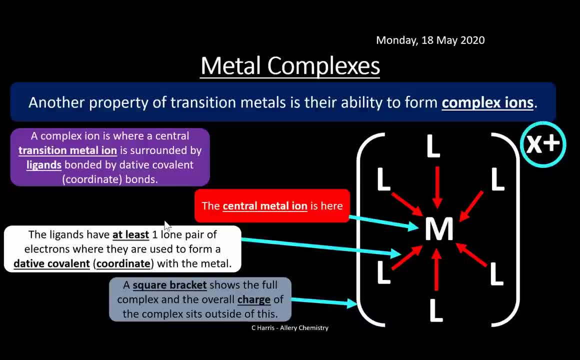 bracket as well, and the square bracket basically surrounds it, basically partitions off our complex, and then we have a charge, uh, on the outside as well. the charge is just the um, so the charge of the complex. so it's a in this case that obviously metals are positively. 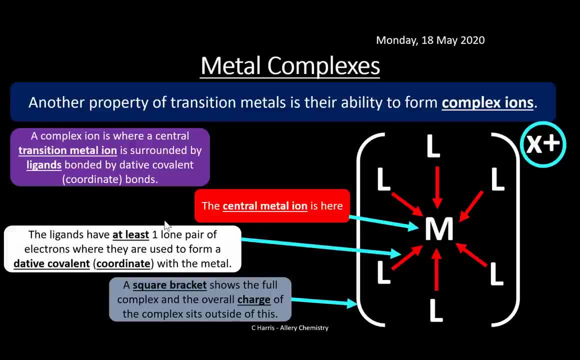 the metal ion is positively charged, but you can get complexes which are negatively charged as well. so that shows the overall charge of the of the complex. okay, and obviously the metal ion, the charge and the metal ion in the middle has an impact on that, and so does the, so does the ligands. 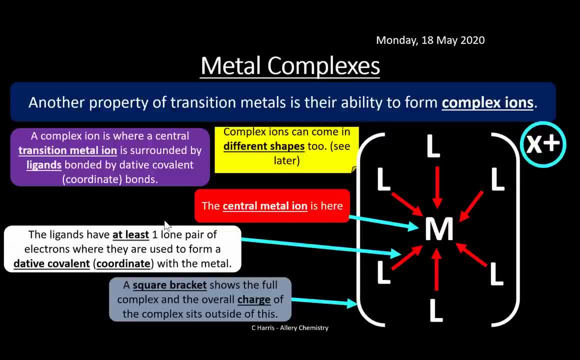 okay, so, um, complex ions come into different shapes as well, so this is an octahedral shape. and you would have seen this in year one chemistry when you looked at the shape of shape of molecules. so this is an octahedral shape, but we'll look at that later. okay, um, right, so. 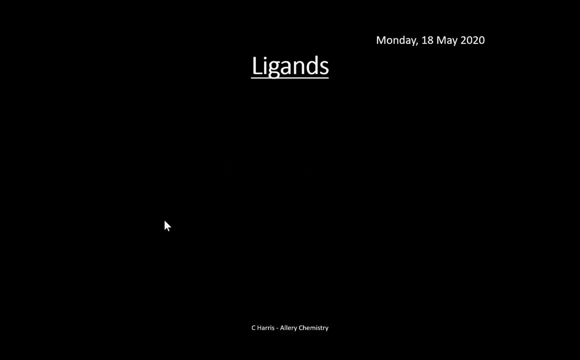 let's look at um. let's look at ligands. okay, um, ligands, remember were them things which surrounded the metal ion in the middle there. so these are the molecules. um, and remember, ligand is an atom that must have at least one lone pair of electrons. 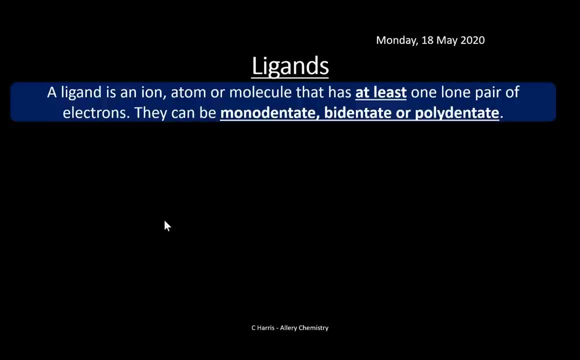 and if they don't, they're not a ligand. so that was a. that is an absolute fundamental criteria for ligands, and they can come in three different types. you can get monodentate, bidentate or polydentate ligands. okay, so let's look at the monodentate ligands first. they're 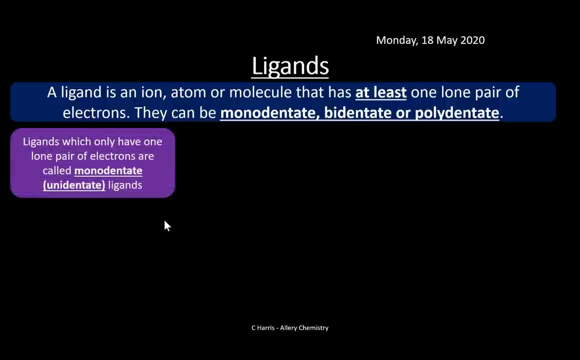 also known as unidentate ligands. so these only have one lone pair of electrons that they can donate to the metal ion, and there's three specific examples that you need to know for aqa, and that is water ammonia, which is nh3 and cl, minus your chloride ion. so you need to know them as well. so they're the ligands that you'll. 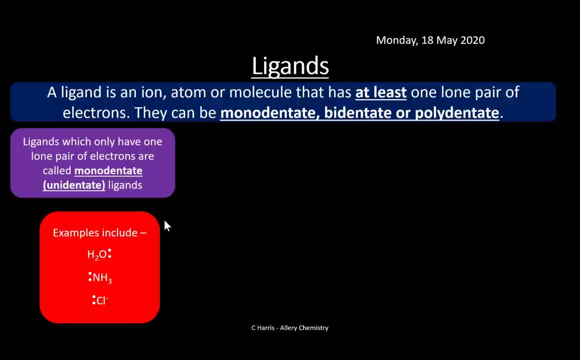 see them all the way through, particularly in the next topic, and when you look at aqueous ion, transition metals and aqueous ions, um, you know they're really going to come into their own in that topic, um. and then we've got our bidentate ligands. so these are ligands which have two lone 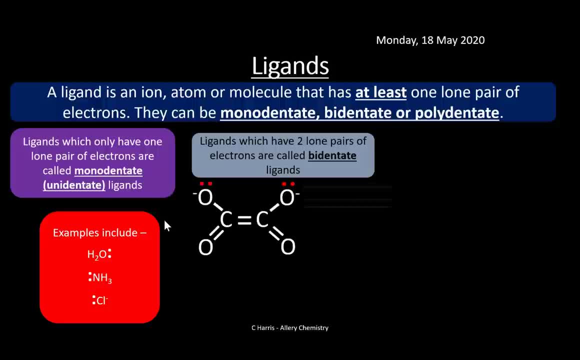 pairs of electrons. so specific examples that you need to know for this are ethane diuret, which is basically a dark di carboxylic acid, as you can see there. so we've got our carboxylate ions there, and the other one is ethane one two diamine, and you can see here that we've got two amine molecules. 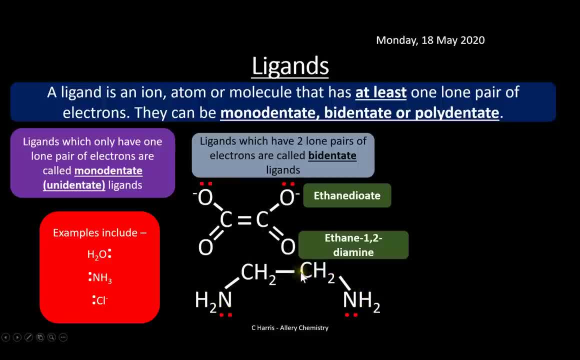 here, attached obviously to an ethane, which is your two carbons. so it's ethane one, two diamine. okay, so ligands which have more than one coordinate bond are called multi-dentate ligands. okay, so multi meaning many or lots of so specific example here. there's two examples: you 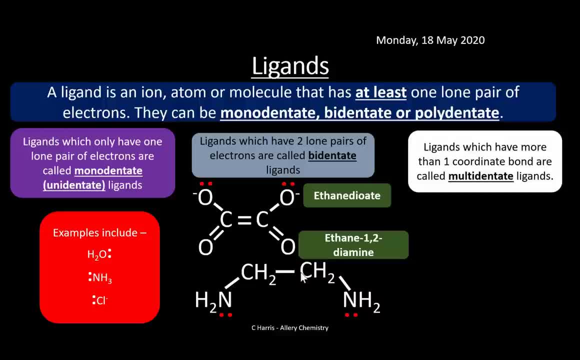 need to know. so one is heme, which we'll look at later when we look at hemoglobin, and the other one, or edta four minus, and this is multi-dentate because it forms six coordinate bonds with the central metal line. so it is a colossal ligand and it literally takes up, uh, all of the space. okay, 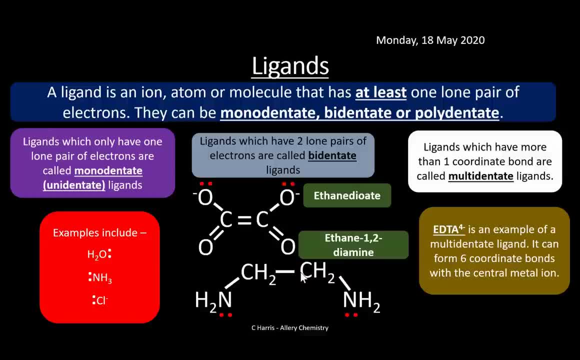 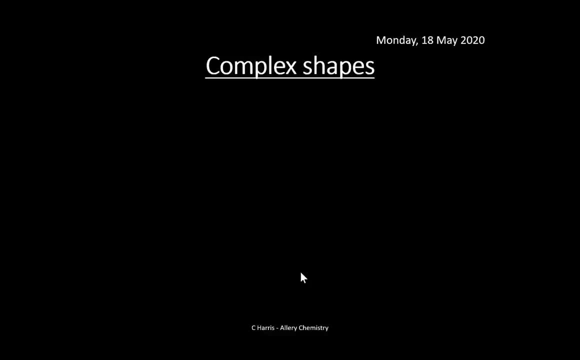 so, talking of space, um, we're going to look at something called complex shapes now. um, obviously we've got our ligands, we know what the ligands are, so we now need to know, you know, how do these ligands actually, um, you know, affect the shape of a, of a complex, and it's actually the size. 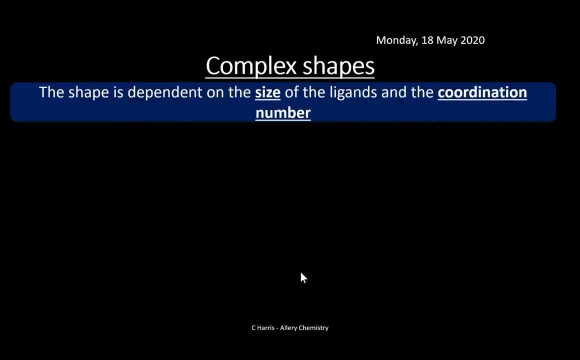 of the ligand. that actually, um determines the shape of the ligand. so we're going to look at shape of it, um, and the coordination number as well, and i'll um. we'll look at coordination number now, but you've got to be careful not to get the two confused. so a coordination number is the number. 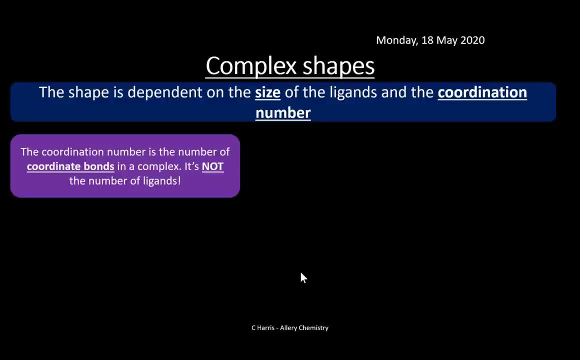 of coordinate bonds in the complex, it's not the number of ligands. so you might have, for example, um six ligands around there. they will have six coordinate bonds. but you may also have only three ligands surrounding a metal line and but you have still have six coordinate bonds in the middle. so 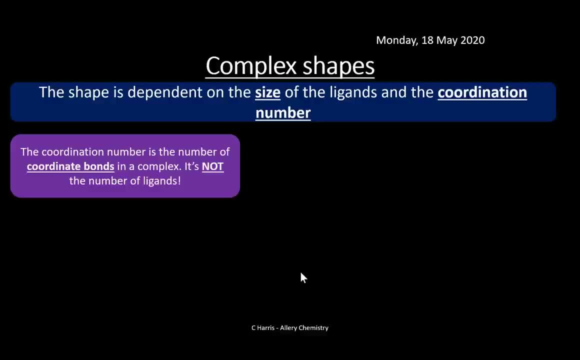 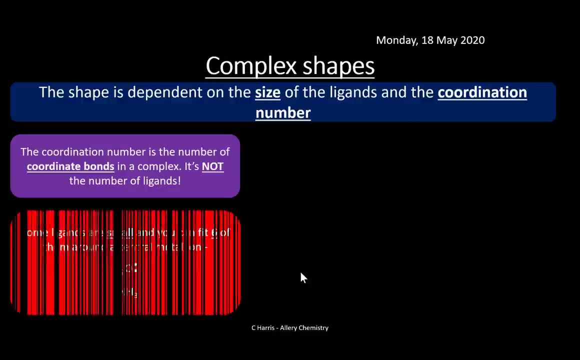 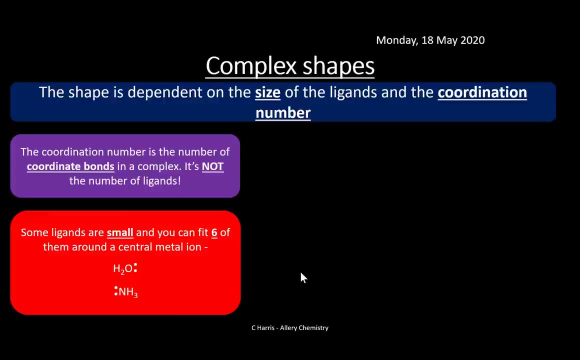 there's a stark difference. so the coordination number is the number of coordinate bonds, not ligands. okay, so ligands can be split into different sizes. so we've got, um, some ligands are small. so these are, uh, things like water, molecules, like water and ammonia. uh, because they're small, you can fit six of these around the central meth line. 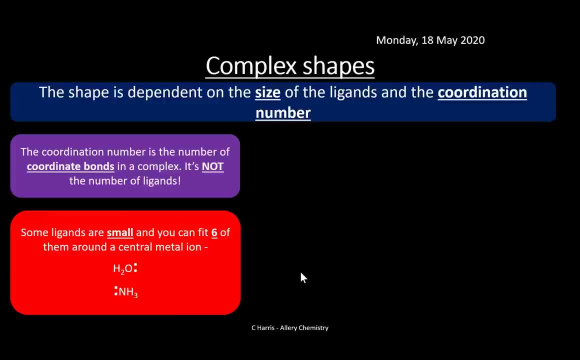 so i like to see this kind of, as um say, like pigs around a trough. so imagine your met line in the middle is the trough and you've got all the food in the trough there, okay, and then you've got the pigs. the pigs are like the molecules. 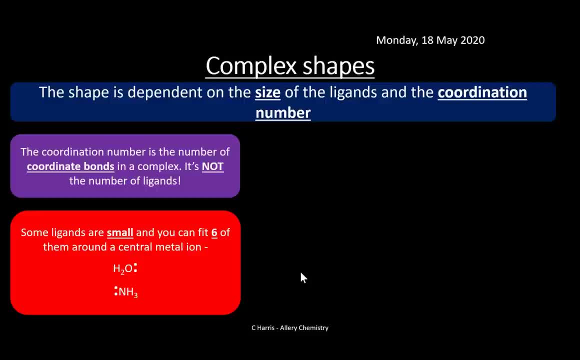 around the side. so imagine if you've got low late little pigs- um so piglets, let's say, and you can fit six of them around there because there's enough space to fit six of them out. but let's say you've got fatter pigs, and fatter pigs, for example, are well, they're bigger and we can get. 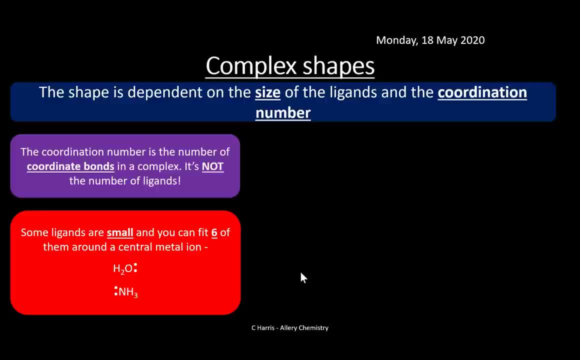 bigger ligands we'll look at in a moment. um but um, fatter pigs, you can't fit as many of them around the trough. okay, so ligands are the same. so if you've got a bigger ligand, you can't fit as many of them around that meth line. they're just quite. there's simply not enough space around the trough. 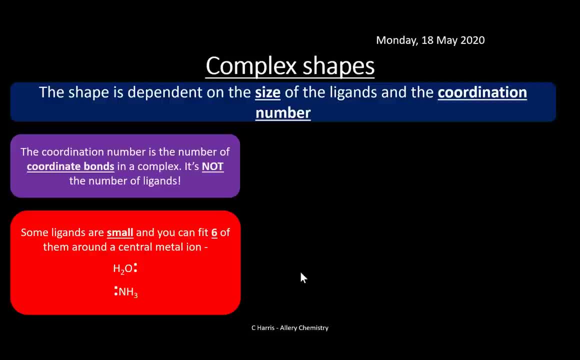 there. so obviously these ligands here, the water and ammonia- these ones are small so you can fit six of them around. but an example of a larger ligand is a chloride ligand and you can only fit four of these around a central metal line because it's a lot bigger than water and ammonia and you 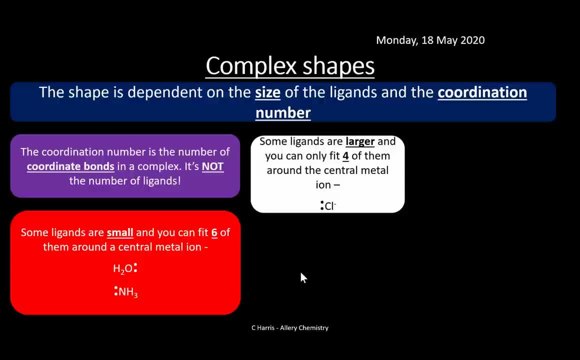 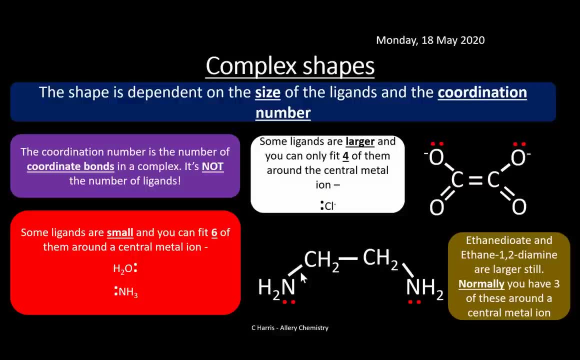 just physically can't fit any more around than um than the four, and bigger still are your bi-dentate ligands. so things like ethane dioate and ethane 1- 2 diamine are larger again and normally we only have the same size with the other ligands, but there's a lot more space around in your met line. so because 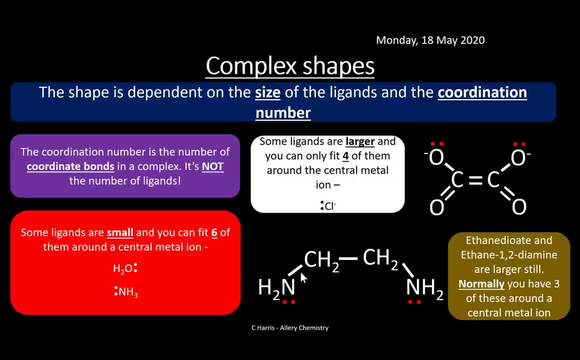 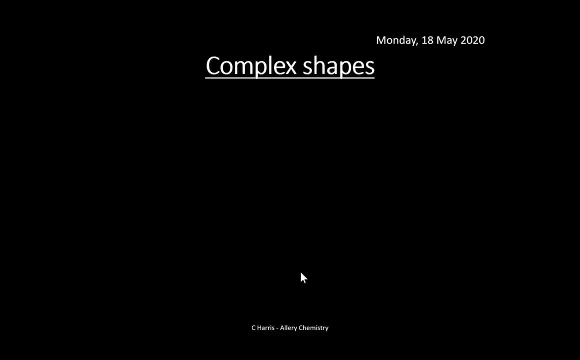 they take up even more space than the chloride ligand or the water and ammonia ligand. okay, so these are different, obviously different ligands and the size of them. so you can see that the size of the ligand does have a significant impact. so let's look at what shapes they actually form. so 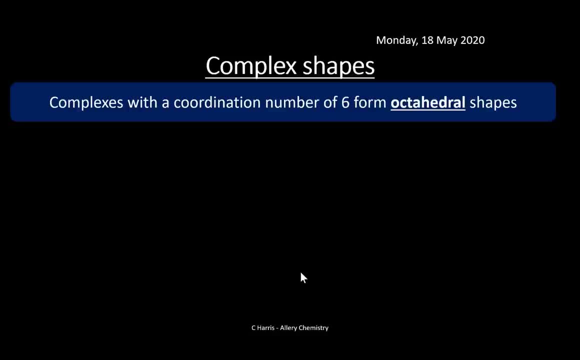 complexes with a coordination number of six. these form octahedral complexes. so you can see here that water ligands surrounding the cobalt meth line in the middle. there the overall charge is 2 plus and it can also be written as that: so cobalt, and we put 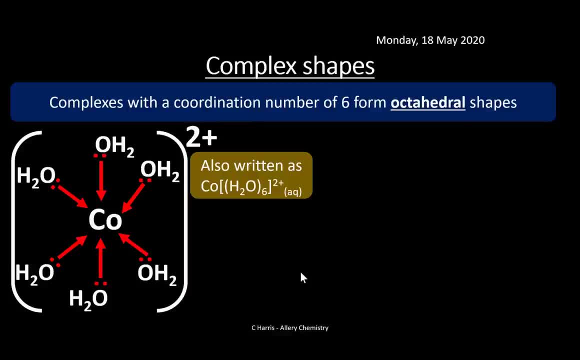 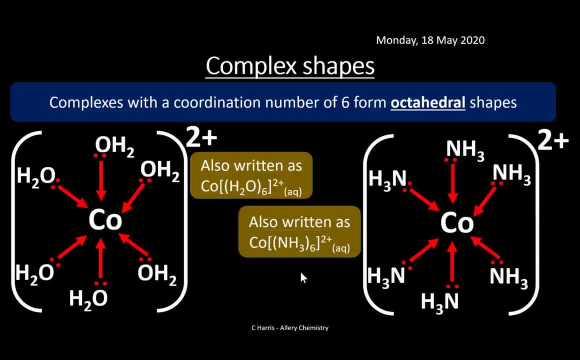 the square bracket around the six waters, as you can see on there, and that's actually with the 2 plus charge, so we can also write it as that. remember, ammonia is also a smaller ligand and that can be written as that. so you can see there's various different ways in which we can draw this. obviously the lone. 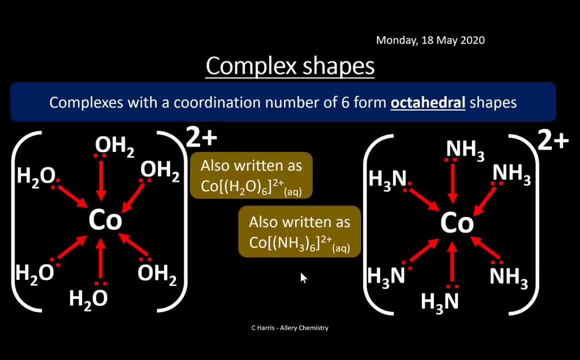 pairs, and the ligand is really, really important here, and it's about trying to write the the formula correctly as well. okay, so all bond angles in octahedral shapes are 90 degrees. okay, so 90 degrees in all of them. remember that from year one, chemistry, and we looked at the shapes of molecules, they're all 90 degree. 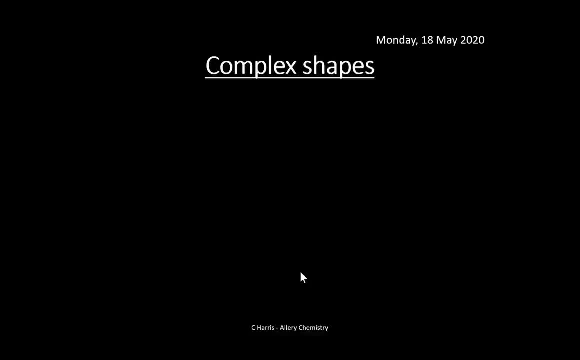 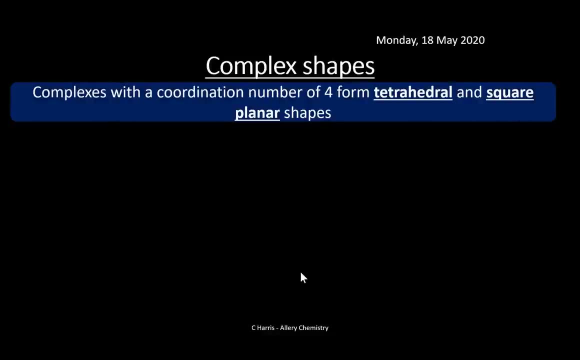 or 90 degree shapes, okay. so let's look at the next type of shape, which are tetrahedral shapes. so you're with four ligands around there now. they can come in tetrahedral or they can come as a square planar shapes as well. so let's look at the tetrahedral one first. so you 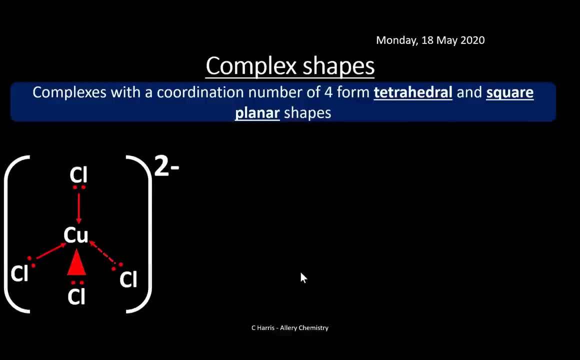 can see here they've got a copper in the middle and we've got four chlorine ligands surrounding the copper there and that this has an overall charge of two minus. but we'll look at that later, look at that in a bit more detail later and obviously you can say it's also written as CuCl4 in the square brackets and 2. 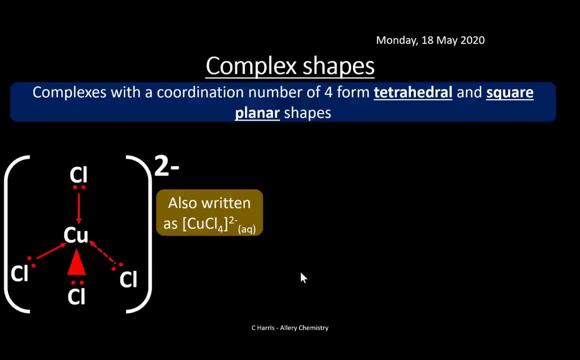 minus. now can you remember what the bond angle is for a tetrahedral shape? well, the bond angle is 1.9nic planar there, as you can see, that it's got. your still got four ligands, but it's flat. now you don't need to worry about differentiating between these. 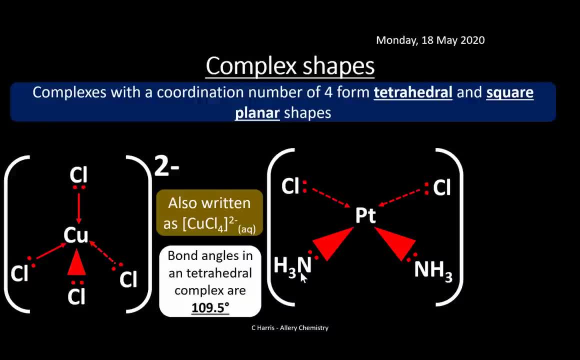 two much because the specific example that you need to know is square planar, and that's specific example is cisplatin, as you can see, there you go. so you need to know, and the only square planar is in a much larger volume than all regular meters of chemistry. so that is square. 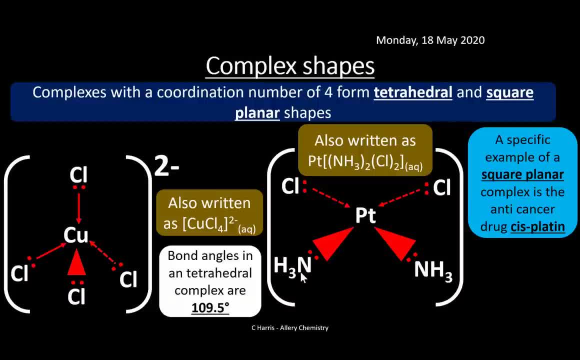 planar, and let me show you the square planar. square planar, one that you need to remember is cisplatin, um. so any other ones they'll have to tell you. the exam board will tell you about them, um. so what do you think the um bond angle is with? 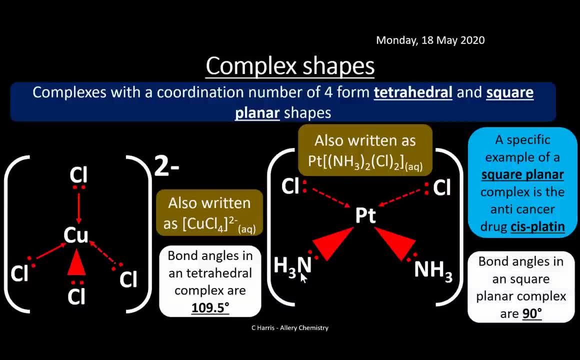 this with square planar. well, the bond angle is 90 degrees. so, remember, all of this stuff is stuff that you've done in year one: chemistry, um, so when you've done, obviously, um, shapes or bond angles etc. so, um, in there, i think it's in the bonding topic. i believe, uh, structure and bonding okay. 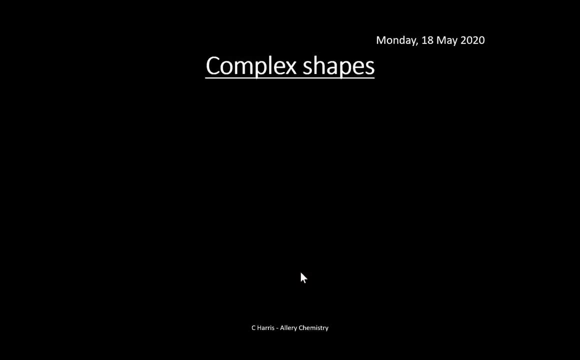 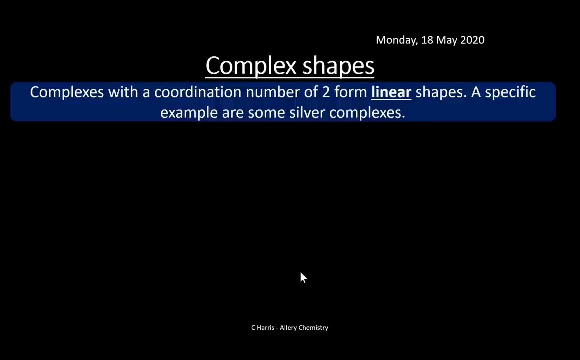 so, um, let's have a look at some um, another complex shape. so we've looked at octahedral, tetrahedral and square planar. the other one, um, is, uh, has a coordination of two, and these are called linear shapes. um, and you again, just like with the cisplatin, with the square planar complex. 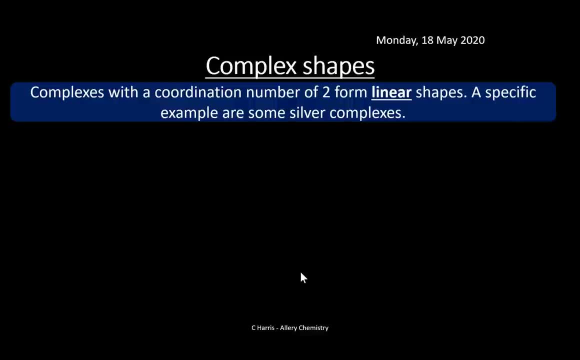 there's a specific example that you do need to know um that are that are linear, and that is this example here, so it's also written as that. okay, so so it's um your diammonia, silver complex. as you can see here, bond angle linear is 180 degrees of. 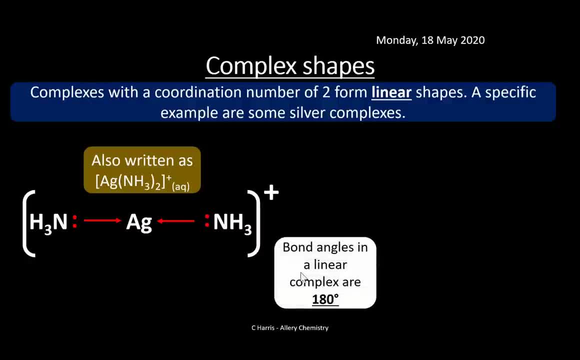 course, that's fairly straightforward. it's just angles on a straight line. um, now, you might recognize this possibly. um, so this is actually tollens reagent. um, so this is actually what you used to test for or to distinguish between aldehydes and ketones, remember? uh, right, okay. 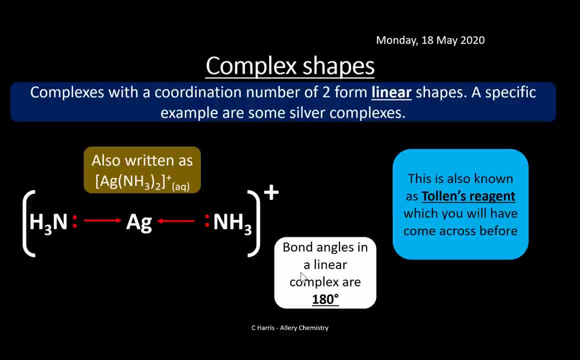 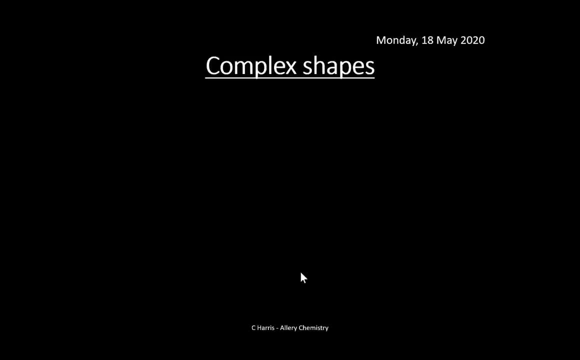 so tollens is the silver mirror, so if you, you probably might remember that, okay. so, um, looking at these shapes, okay, so we now they're all the shapes that you need to know. so you've got your octahedral, tetrahedral, square planar and linear. now what we need to do is then: 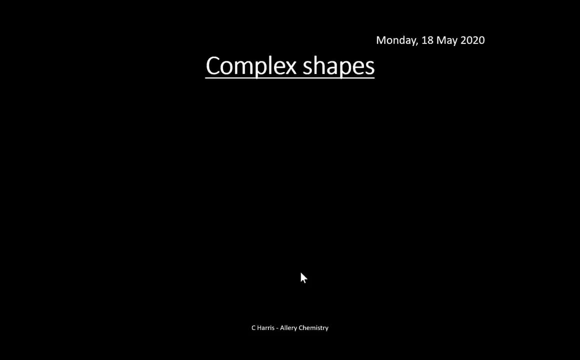 say: right, okay, using them shapes. you're seeing the, the little charges on the outside of the, of the um cases that we've seen there, um, so we need to be able to um, work out the oxidation state of the transition metal in the middle of them, uh, of the of the complex, and that is determined. 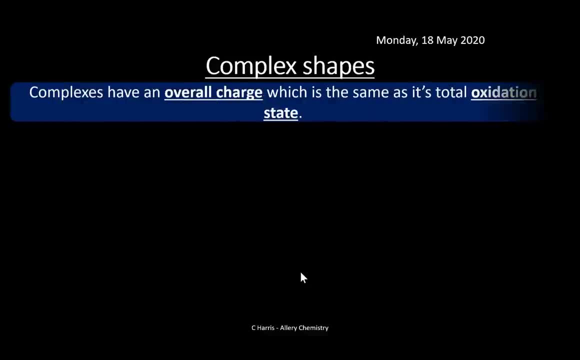 ligand and the number of ligands that surrounds the metal ion. So let's have a look. So it's the same. The complexes have an overall charge which is the same as its total oxidation state. So how we work out the total oxidation state of the metal, the transition metal in the middle is 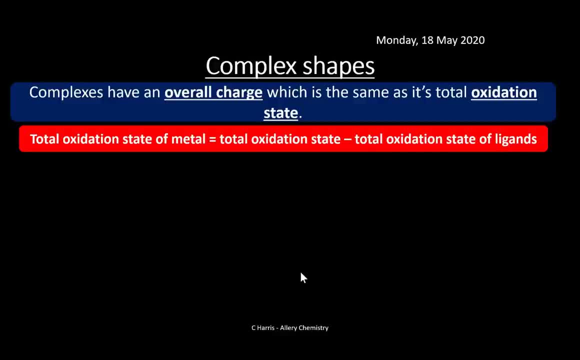 basically the total oxidation state of the complex minus the total oxidation state of the ligands, so the individual ligands. So let's bring up an example here. So this is one of the tetrahedral examples we'd seen here. See, at zero it has a two minus charge, so the overall charge is minus two. 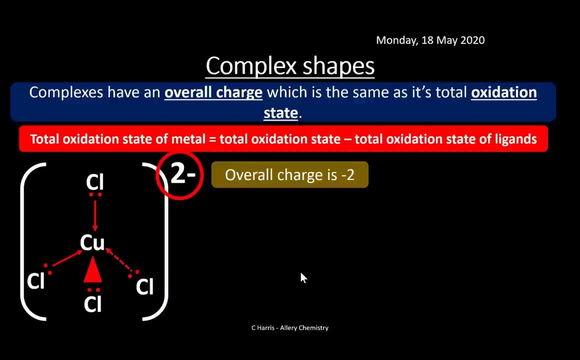 with this complex. So that's the total oxidation state. Then we need to subtract that away from the total oxidation state of the ligands. You can see here that we've got four ligands, four chloride ligands. Each has got a charge of minus one because it's a Cl minus. So that's. 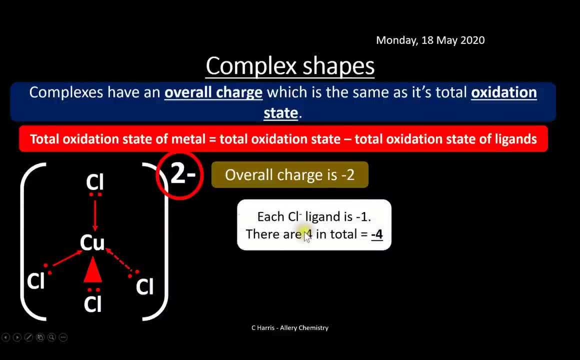 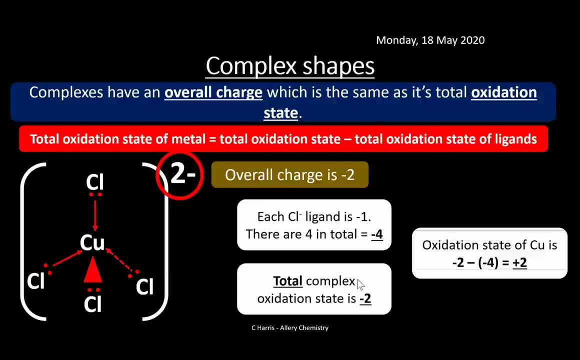 effectively going to give us a total charge of minus four. Now if we put these numbers in here, it's minus two Minus minus four. we're going to get a total complex. oxidation state is minus two. Sorry, that's the overall charge, the total complex, And then if you put them figures in there, 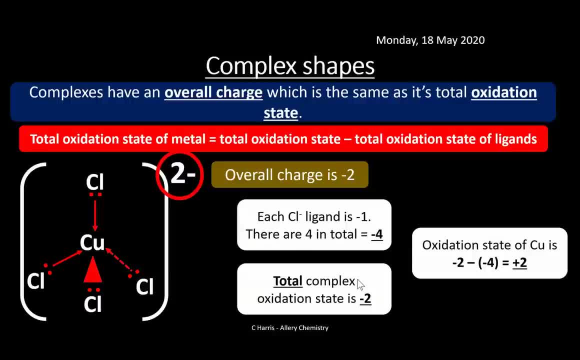 then we get the oxidation state of copper going to be plus two in this case. So you'd see, it's fairly straightforward, but you are expected to be able to identify the oxidation state of the transition metal in the middle, And this is how you do it from the complex. 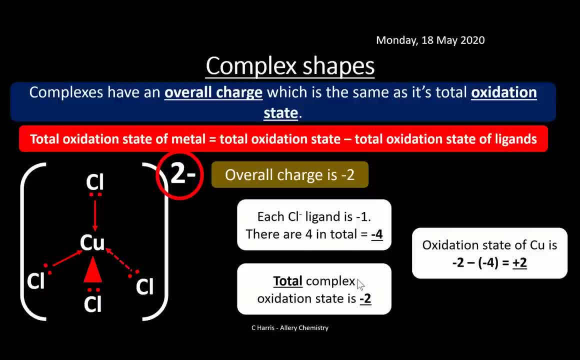 Right. so now we're going to look at a very specific type. So, remember, we looked at the different types of complexes. So we looked at, for example, your monodentate or unidentate ligands, such as water, ammonia and chloride, And then we looked at our bidentate and then our 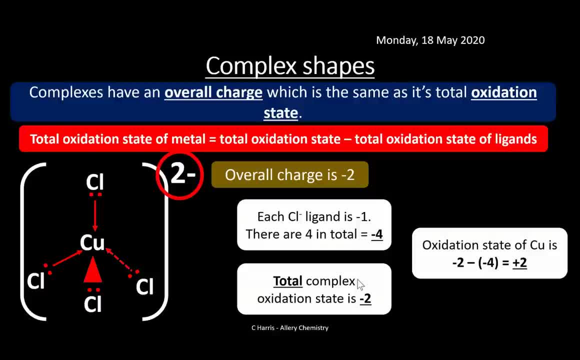 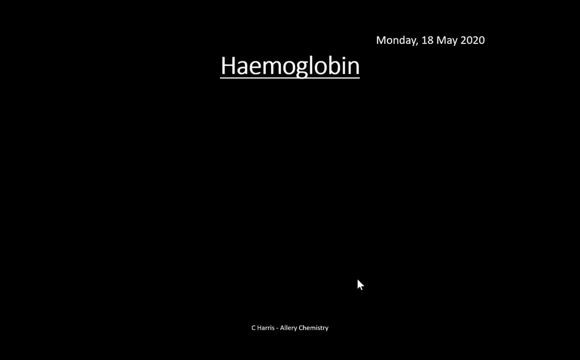 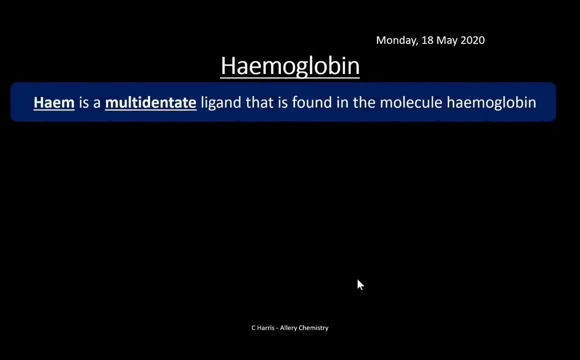 multidentate ligand, And an example was EDTA. Well, this example here is another example of a multidentate ligand, and this is actually hemoglobin, And so hemoglobin is the substance that transports oxygen around the body, but heme is the actual ligand and it's a multidentate ligand. 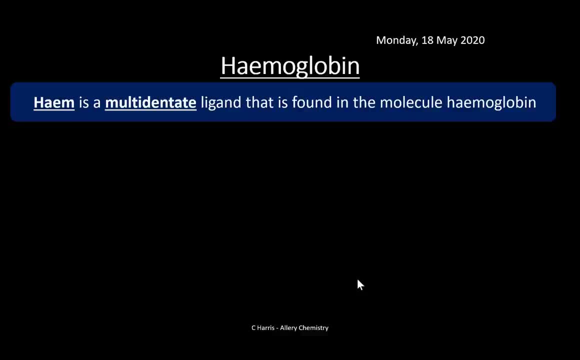 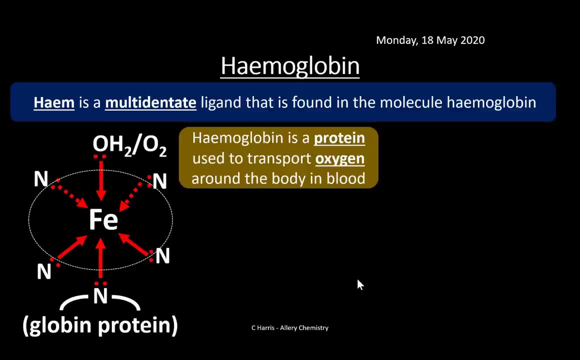 that's found in hemoglobin, So let's have a look and see what it looks like. So remember, hemoglobin is in your red blood cells and it's iron in the red blood cells And it's the iron which is very important here, because the iron actually is a transition metal, as we know, and we have ligands. 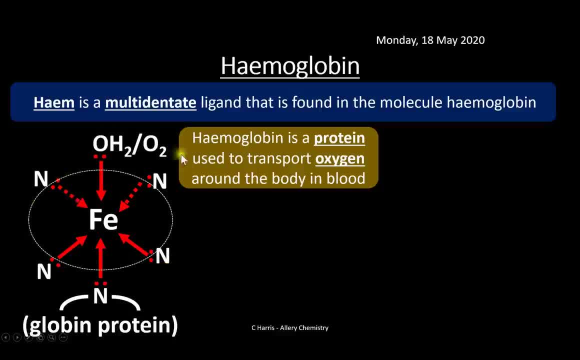 surrounding that iron there. So you can see here that hemoglobin is a protein- this is the full thing- and it's used to transport oxygen around the body. So you can see that it is an octahedral shape. so that's it there And the circle here of the nitrogens, basically the circle. 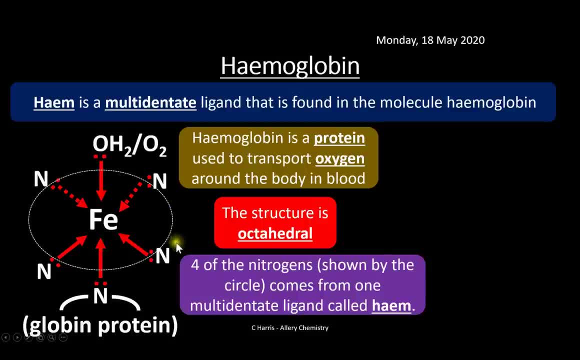 is representing heme. This is the ligand here, so this bonds four times heme. So it's not quite as big as EDTA, but it's still quite a big ligand in terms of the number of coordinate bonds it can form. So there's four lone pairs and effectively these are the ones that are the most important. 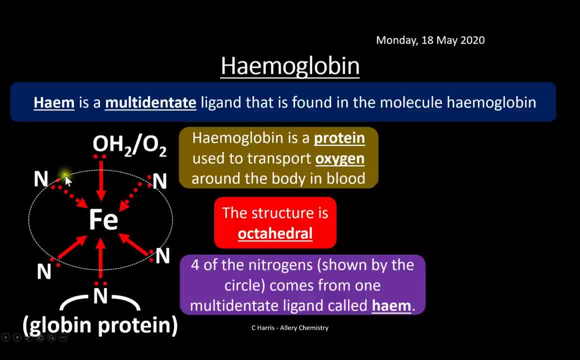 These are all connected by. there's a lot more atoms around the side here, of course, but to simplify, we've just shown as a dotted line. So this is from the ligand heme. Now, one of the coordinate bonds you can see there comes from a large protein called globin. So globin is the one. 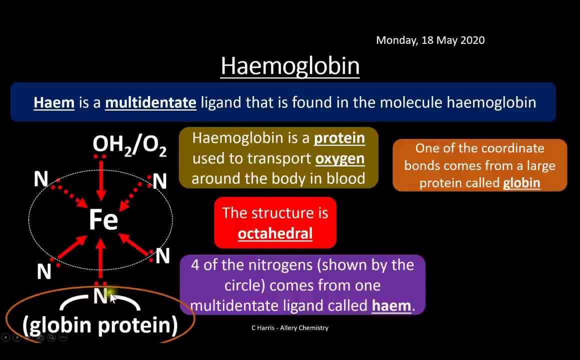 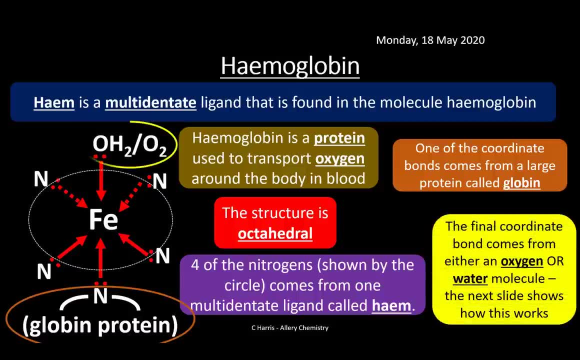 at the bottom. there That's your globin protein, and one of the nitrogens obviously comes from that protein at the bottom. Now the other one, the final coordinate bond at the top there, actually comes from a nitrogen or a water molecule, And so, depending on the state and where the hemoglobin is, 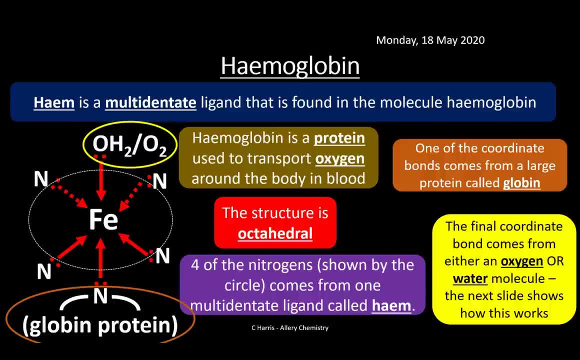 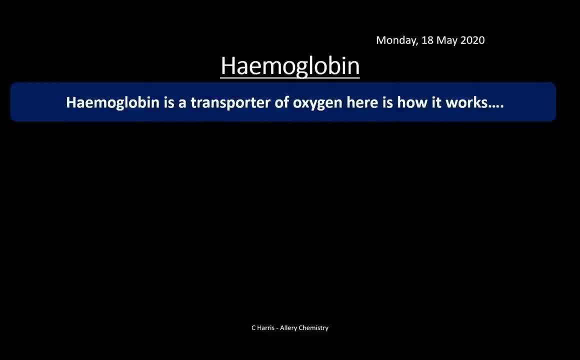 at the time will depend on if it's carrying oxygen or if it has a water molecule on there. Okay, so hemoglobin is a transporter of oxygen, okay, as we know, and we're going to look at the mechanics of that. So how does it actually transport oxygen? How does it actually work? 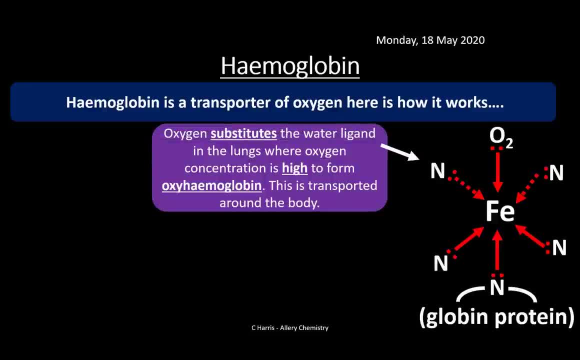 in our body. So you can see, here's our complex. So we've got iron and this one's got oxygen attached to it. So we've got iron and this one's got oxygen attached to it. So we've got iron and this one's got oxygen attached to it. 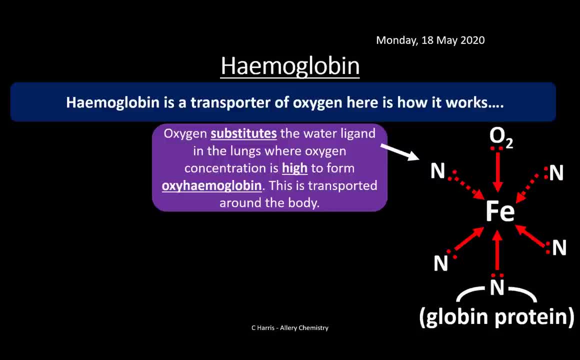 Okay, so this is our hemoglobin. So what happens is oxygen substitutes the water ligand in the lungs. So remember you've got loads of oxygen When you breathe in, you've got a good supply of oxygen in the lungs there and hemoglobin is in the blood supply. And obviously that if you do biology. 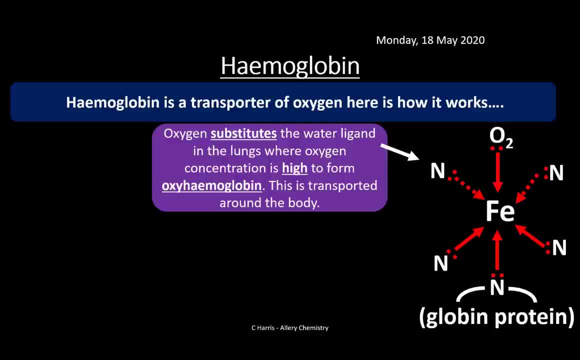 you'll know this: The blood supply. you've got tiny, tiny capillaries that come quite close to the alveoli in your lungs and you get gas exchange. So you get the molecules here picking up oxygen from the lungs and effectively depositing water. because this 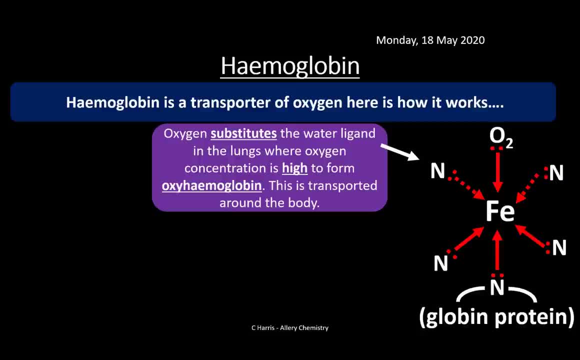 would have carried water beforehand, but we'll look at that ligand in a moment, So this would have carried water from that. So the water is then expelled from the body. So that's why, when you breathe out like this, okay, as if you need an example, but when you breathe out like that, 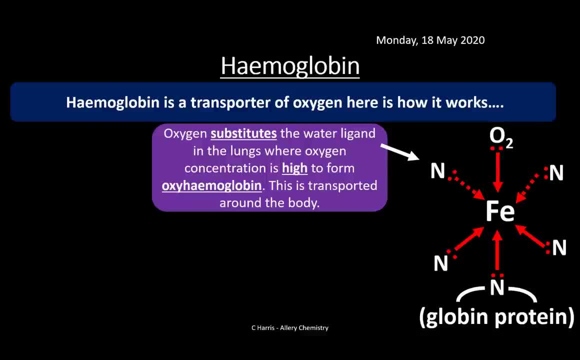 obviously you breathe out water, water vapor, and that's obviously come from that was attached to hemoglobin, So it uses up the oxygen and that's why it's so important to have oxygen in your lungs. Okay, so we've got our oxygen and we've got oxygen in the lungs, and we've got oxygen in the lungs. 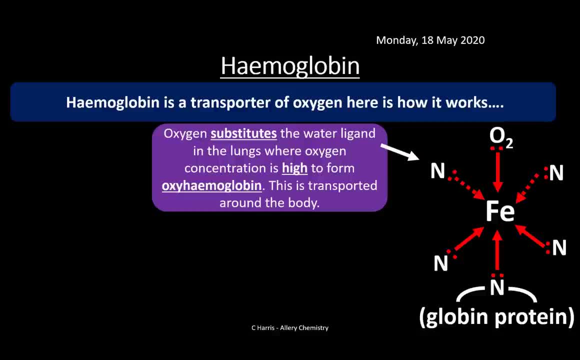 Okay, so it picks it up from the lungs, It then goes to the you know the place where it's required- It could be a muscle, for example- and then it deposits the oxygen in the muscle. and then what it does is it picks up water from the muscle. because, remember again, if you do biology, you 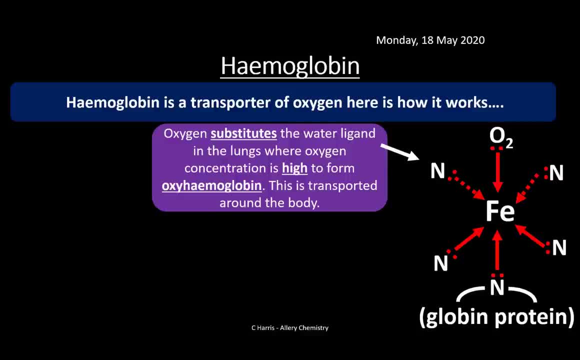 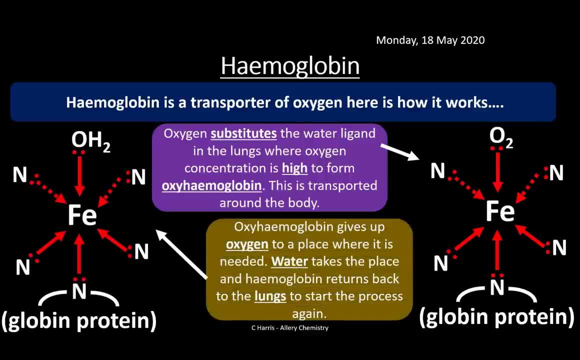 get respiration in cells, and so one of the products of respiration is water, and obviously that's picked up there. So oxyhemoglobin, like I say, gives up the oxygen to where it's needed. Water takes the place, And then what happens to that is it returns back to the lungs. to get rid of the water out of the lungs. 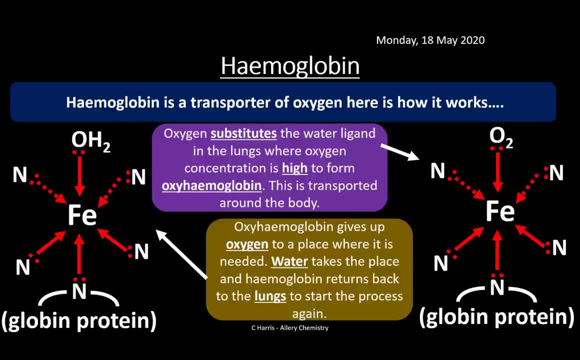 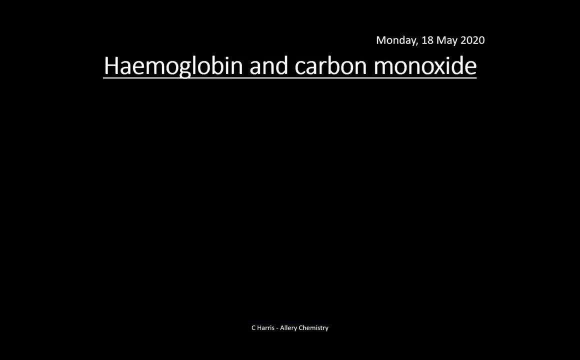 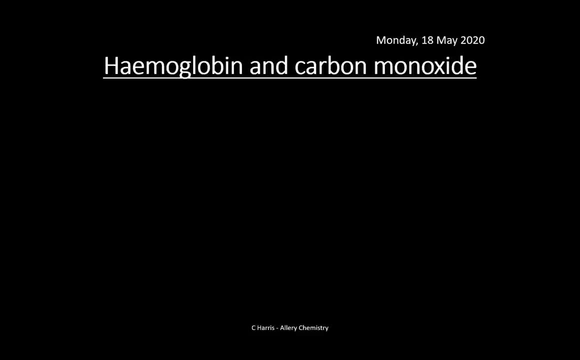 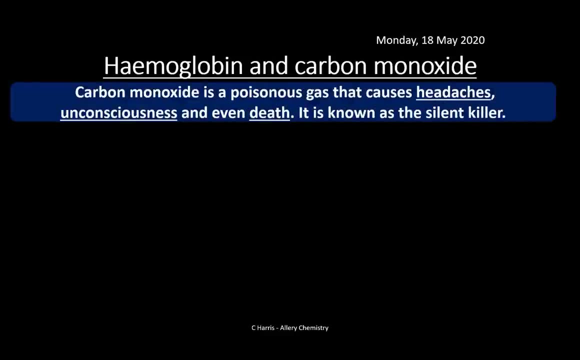 you can't smell it, you can't see it, and when you breathe it in, you start to become nauseous, you get headaches and it's really difficult to know exactly. you know, is it carbon monoxide that actually causes this? 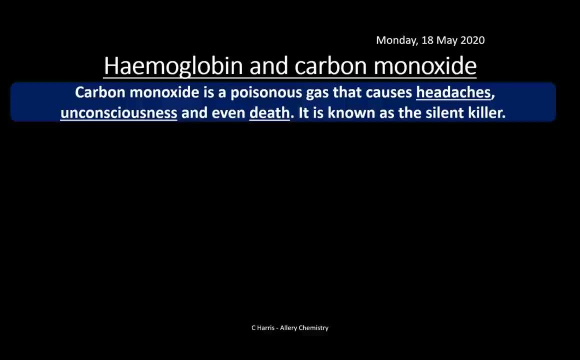 But it does cause headaches and it's known as a silent killer. So, for example, if you have, if you have a boiler, for example, in your bedroom, or you have a boiler in a living space, you must have a carbon monoxide alarm near the boiler. Some older houses in particular, 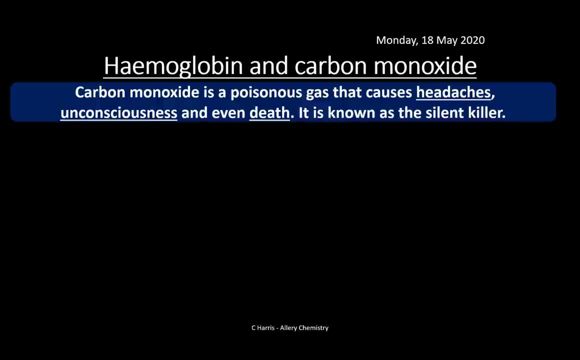 might have boilers in the cupboard in the bedroom. You've got to make sure you have a carbon monoxide alarm because if the boiler's burning incompletely or it's faltering or it's malfunctioning for whatever reason, boilers are designed to regulate gas flow to try and reduce, you know, the amount. 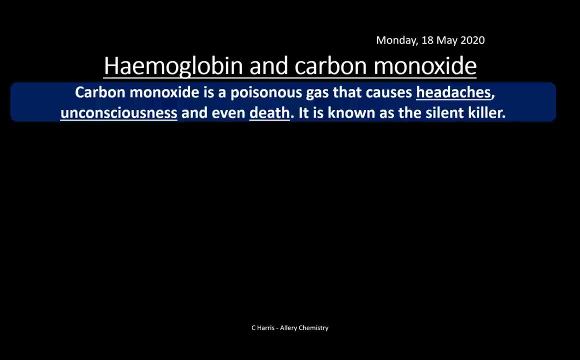 of incomplete combustion, But sometimes they can fault, of course. and if that carbon monoxide leaks out in your bedroom and somebody's sleeping in that bedroom, they won't wake up. It's as simple as that. It's a. it's a really, really lethal gas, So a carbon monoxide alarm is designed. 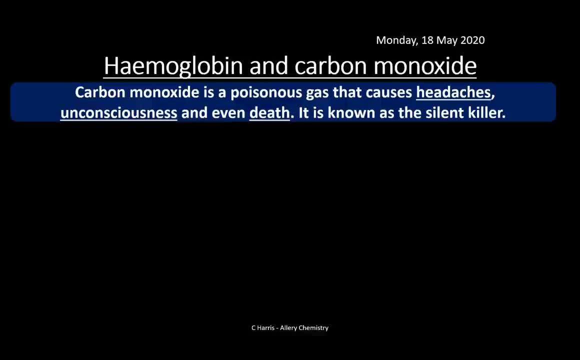 obviously to clearly go off when there's carbon monoxide around, alerts the person in the room to get out of the room. You know a lot of boilers- obviously nowadays are- well, I assume I'm not a builder or a plumber and all that- but you know these boilers, especially new builds, like newer. 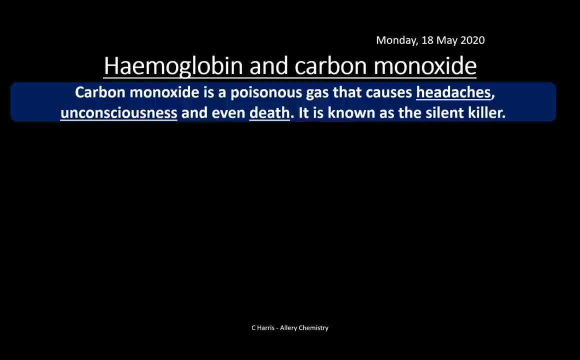 houses they are. they're not put in bedrooms, You know, they're put in a garage, where people- you know people- don't live in the garage or it's well ventilated, Okay, so let's have a look and 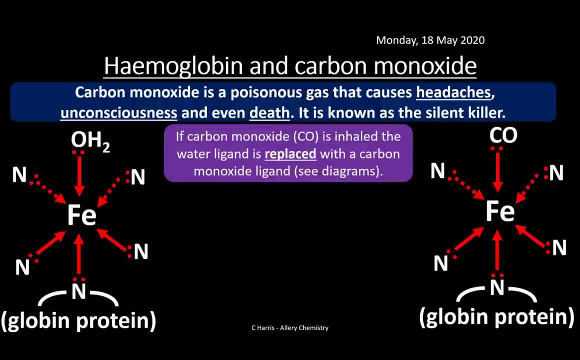 see how this actually works in terms of you know, how does it actually kill us, How does it affect us? So carbon monoxide's inhaled into the, into the lungs, okay, and the water ligand that was attached to that hemoglobin was is replaced with carbon monoxide, and you can see there, Okay. so 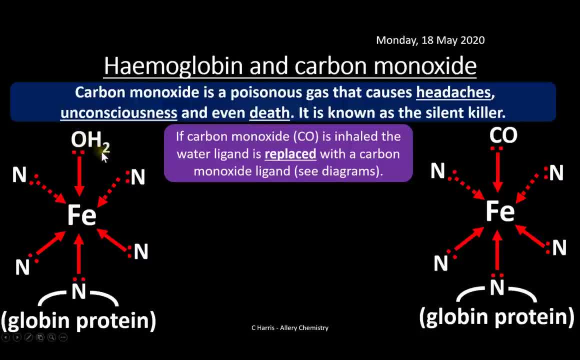 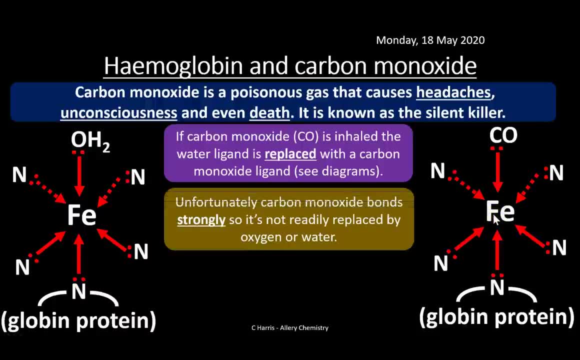 you had your water on the side. there there's your water ligand, Remember. that gives up the water in the lungs and then it picks up carbon monoxide, which is here, and that bonds to the iron. Now the problem is it bonds too well and it bonds really strongly, and so therefore, it's not. 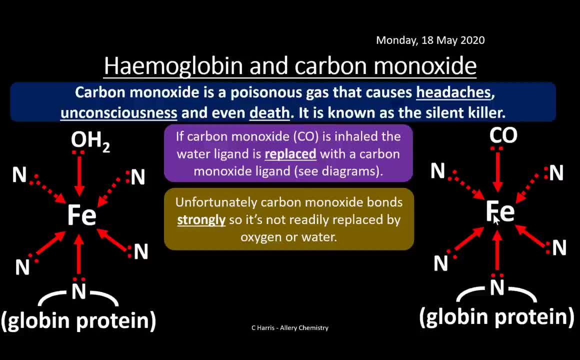 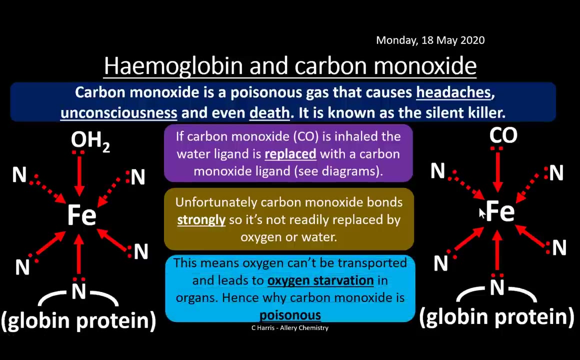 actually readily replaced by oxygen. It's not actually readily replaced by oxygen or water and therefore it just sticks. it sticks to the molecule and it's really difficult to levy this off. So, as you can see, you have a finite, a number of these molecules and if all of them- or good majority of them are- have carbon monoxide as one of the ligands, you're going to be really struggling to get oxygen around your body, because where's the oxygen? how is the oxygen going to be carried if there's no space for it? So effectively carbon monoxide all it does is it's a. it bonds better to the iron in the middle. 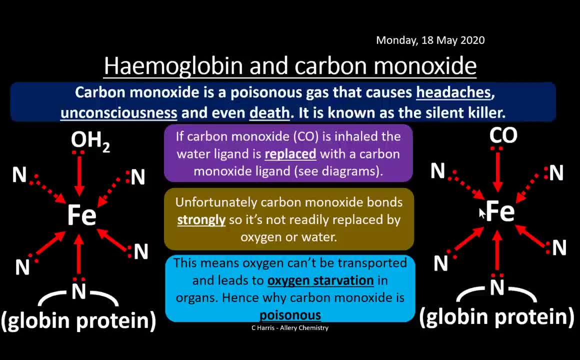 It has a stronger bond, It's not easily displaced by another gas and so therefore, effectively, you you're starved of oxygen, The body's starved of oxygen, which is why you feel sick, because a lot of oxygen to the stomach and also mainly it's the brain. You get a lack of oxygen to the brain, you feel lightheaded and you go unconscious. So, really, really important, you know, but you didn't think you were going to get some kind of safety lesson here, but it's important that you need to know this. obviously, how how carbon monoxide is. you know why it is poisonous and toxic. 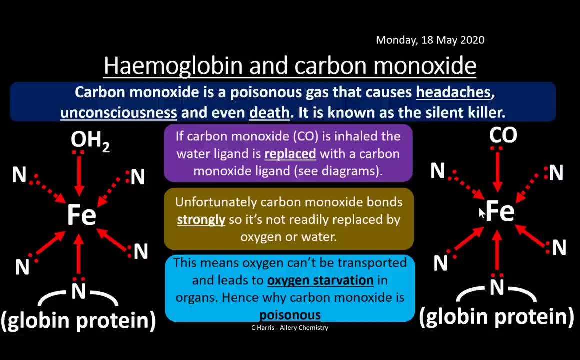 But also about, you know, safety with any anything that burns a fossil fuel. you know, like hydrocarbon, like that. you know it's really important that if it's not burning completely, you know you've got to be able to identify the gases that come from it. 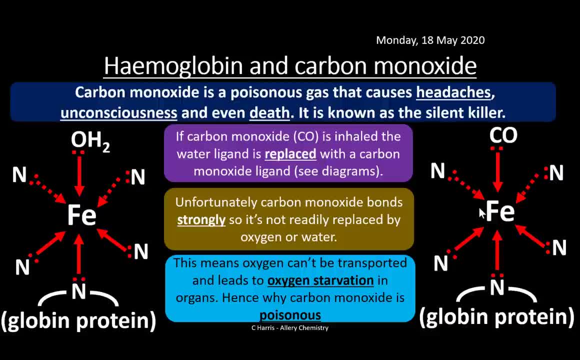 Okay, so we've now looked at that. So now we're going to move away a little bit from you know, you know the ligands and the types of ligands etc. and we're going to focus a little bit more on the complex shape here. 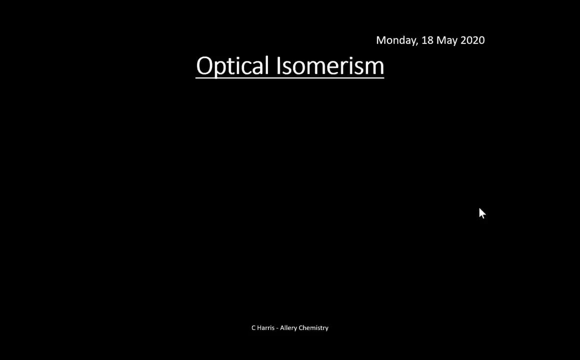 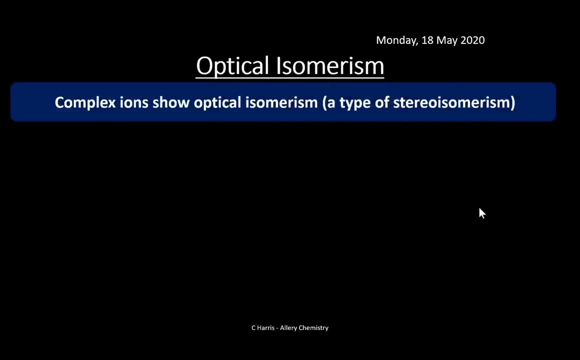 So these transition metal complexes? actually they form optical isomers. Okay, so complex ion show optical isomers. This is a type of stereo isomerism. Okay, so you may have seen this already, depending on the order in which you're learning this. 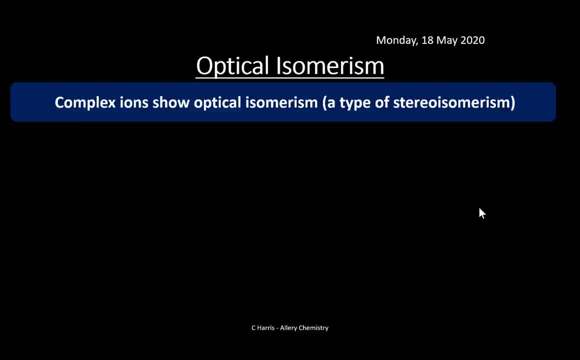 So you need to be aware of you know what. what an optical isomer is? Remember, it's something that's a mirror image, and these are molecules which are mirror images of each other, but they're non-superimposable. 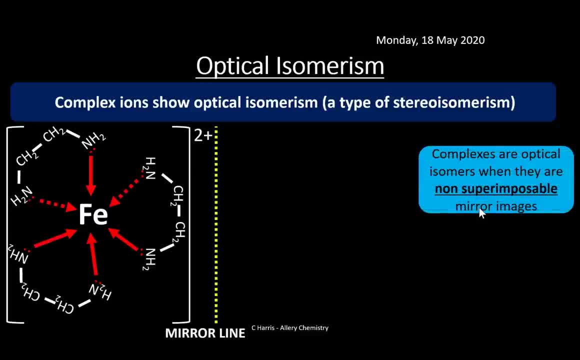 So you can see here that we've got an example where we've got two complexes. So these complexes- you can see the mirror line down the bottom there where we have these are enantiomers. So these are mirror images of each other, mirror line down there, and you can see that these are non-superimposable. 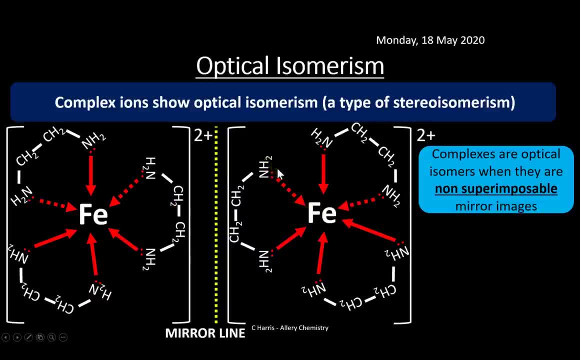 So I can move these across each other and spin it around as many times as I want, and they're not going to actually completely superimpose over each other. So that is that's really really important. Okay now octahedral complexes. 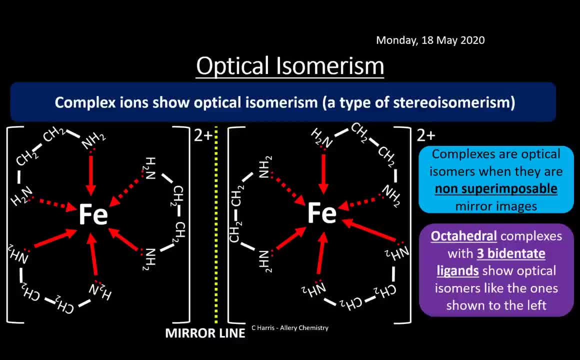 So three bidentate ligands. So this particular example here: these show optical isomers like the ones that we've seen on the left. So that's the criteria. we're looking for: Octahedral complexes with three bidentate ligands. 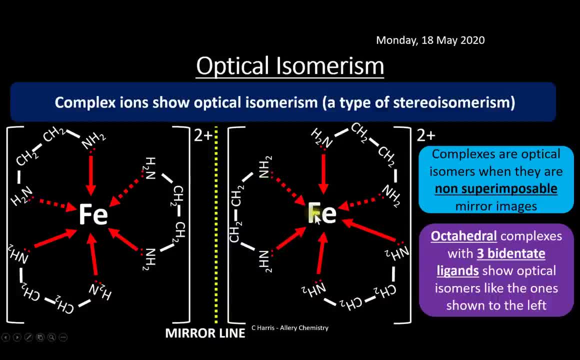 Remember, bidentate means they have two places where they can bond to the metal ion, So the two pairs of electrons obviously on the, on the ligands there. Okay, we can also get something called cis-trans isomerism, and this is complex, which show this: 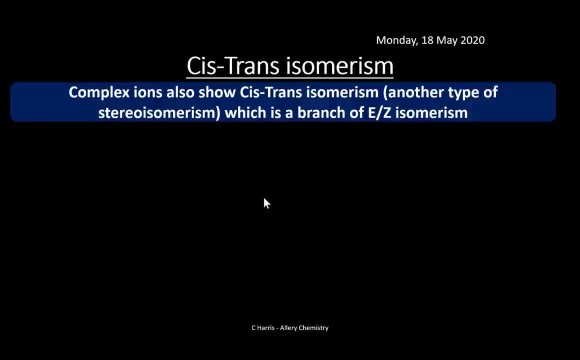 Um is is is. this is just another type of um? uh stereoisomerism. It's a branch of EZ isomerism, but molecules that show this um have a different arrangement of atoms in space. 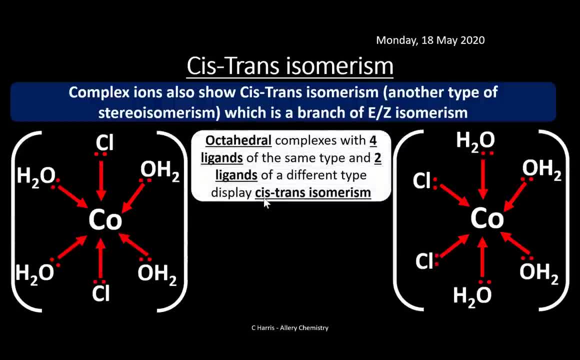 So octahedral complexes. So what we're looking for here, the criteria for this one, is still an octahedral complex, but it's just where four of the ligands are the same and two ligands are different, And these ones, these, any ligands with that type of arrangement, will display cis-trans isomerism. 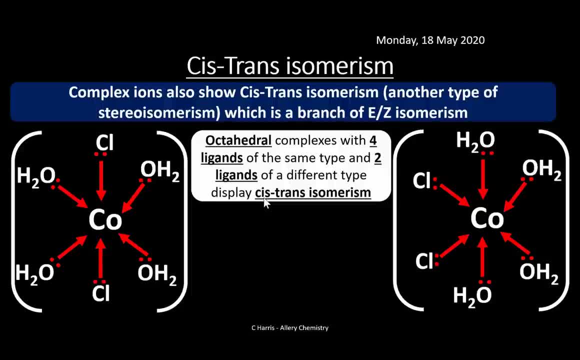 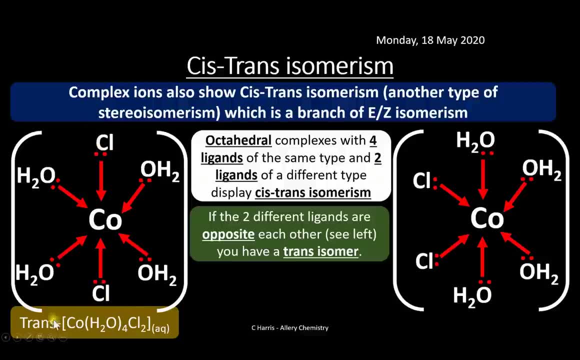 So, for example, if we look at the one on the left there, um, you can see that we've got two different ligands are opposite each other. So there they are. So this one here and one here. because they're opposite, we call this a trans ligand. 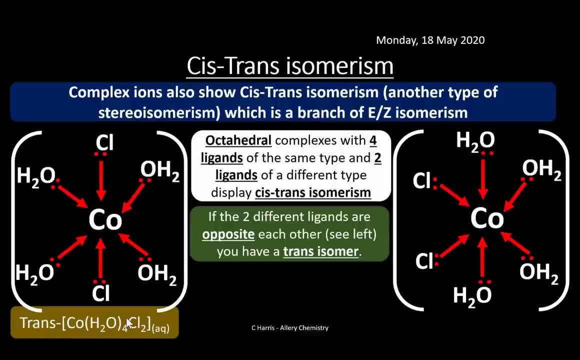 Just like, for example, you've got transatlantic flights, So trans means opposite, Okay, so we've got uh opposite, uh opposite the cobalt there, And then with this one you can see we've got the two ligands that are on the same side. 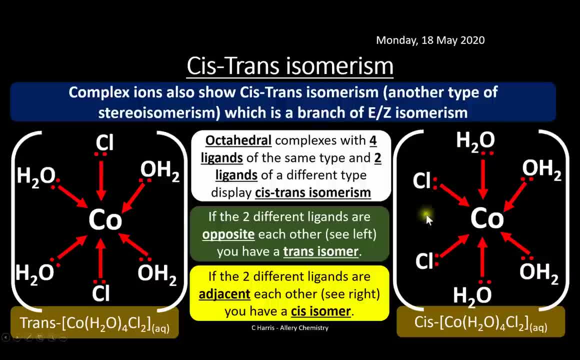 So these are called cis. Okay, So these are adjacent to each other, So we call this a cis isomer. Both of these have the same formula. You can see there. The only difference is that actually this one is a cis and this one's a trans. 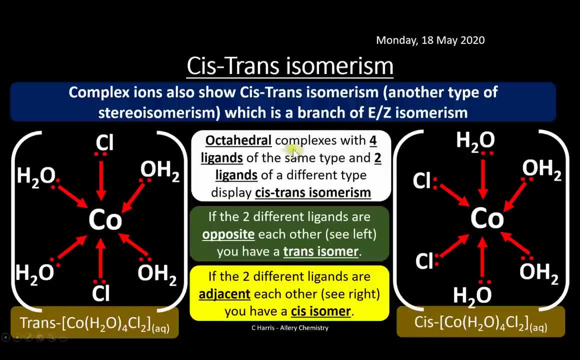 So just make sure you put the name of this in front If it meets this criteria. just get in the habit of being specific with what type of isomer it is- cis and trans Okay, because you may lose a mark if you don't put that in front. 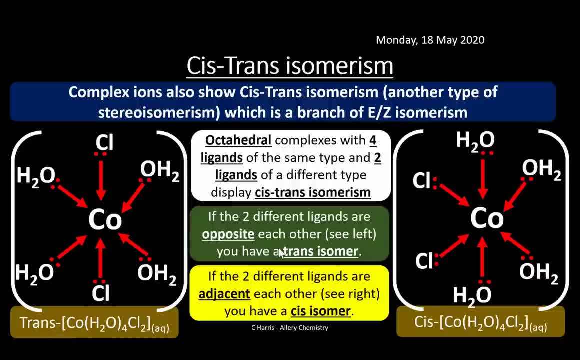 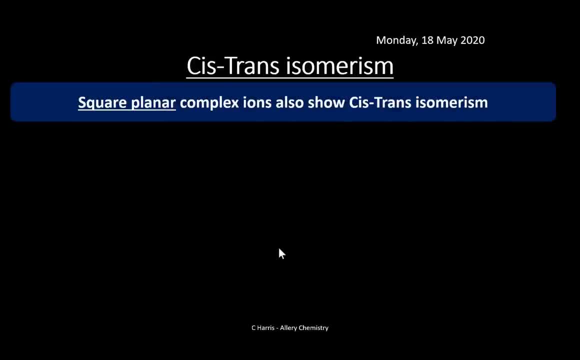 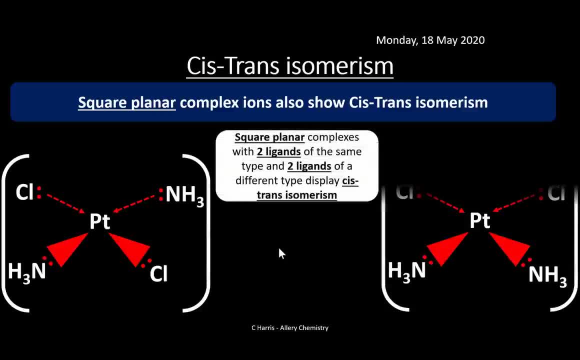 and we've seen some of this already, actually when we looked at cisplatin. So you can see here that we've got some square, plainer complexes with two of the ligands that are the same and two ligands which is different, and these displays cis trans isomerism. 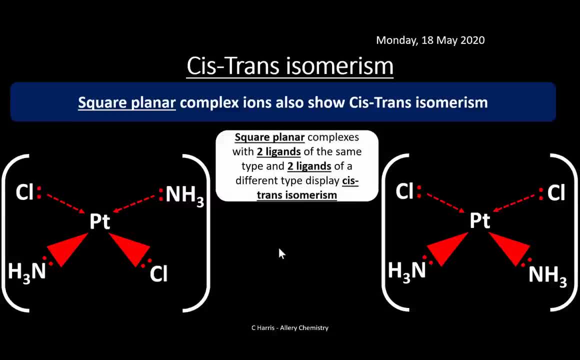 So we've got two types of square, plainer complexes here. So the 1st on the left is a trans trans complex. So you can see If the 2, ligands are opposite each other. so you can see you've got chlorine and chlorine that opposite. 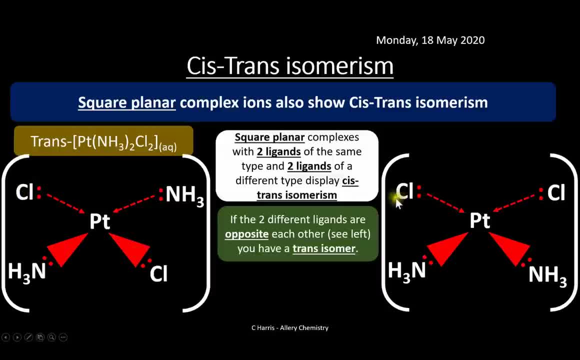 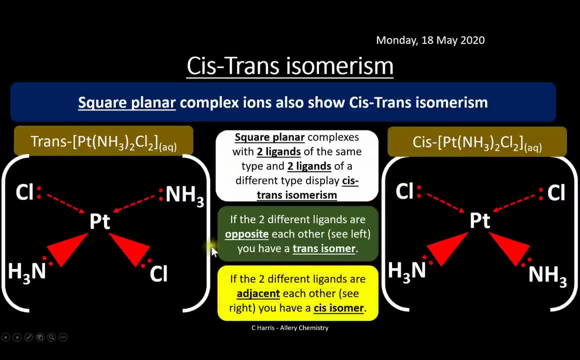 the platinum, okay. then we have a trans isomer and of course, if they are on the same side, as you can see there, then these are a cis isomer. so the ligands here on the same side, the ligands here opposite, okay. so trans and cis, okay. so this one cures cancer, this one doesn't. so the, you know the. 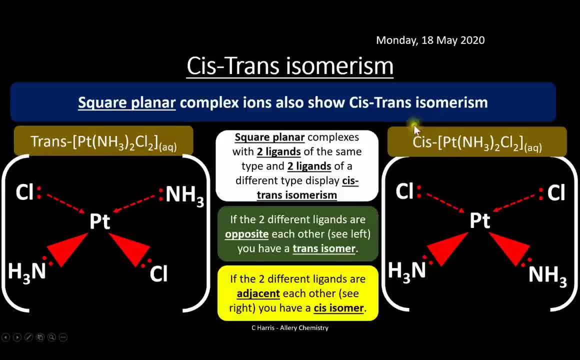 isomerism is critical, particularly in medicine. you know, the isomerism of the molecule really does impact, um, you know, for not all the time, but you know, for things like this. um, you know, your cis platinum does have an impact because one does cure cancer, the other one, the other one won't. 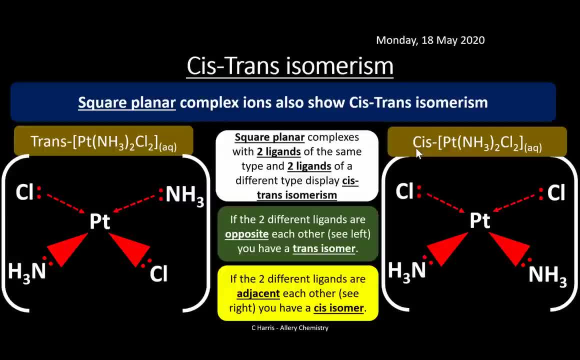 okay. so we've looked at a lot of the complexes here. we're now going to delve into a little bit of physics and we're going to look at some d orbital splitting. okay, so d orbital splitting is is effectively, as the title suggests, it's, where we take a d orbital and we split it. 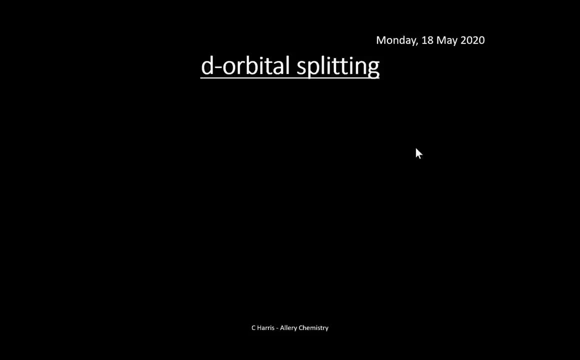 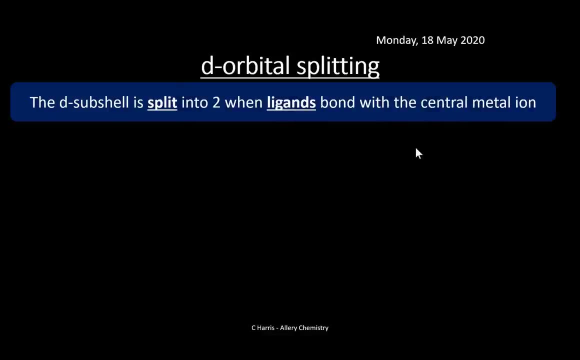 and these are split when, um, you know the ligands, sorry, the d orbital, the split when um ligands are bonded to it. okay, then what happens? you get something a bit peculiar where the ligands, instead of as you've seen, sorry as you've seen the d orbitals, in a line before it actually splits into two halves. so you can see. 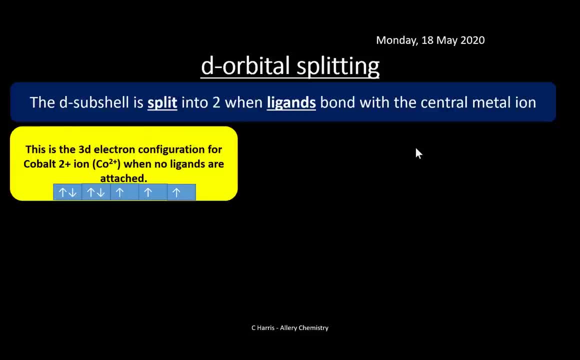 here's an example here. so we've got a 3d electron configuration for cobalt, two plus ions to co2 plus, and this is when there's no ligands attached. so you can see, all of the electrons are in orbitals, same energy level, okay. but something weird happens the moment you add ligand onto this. 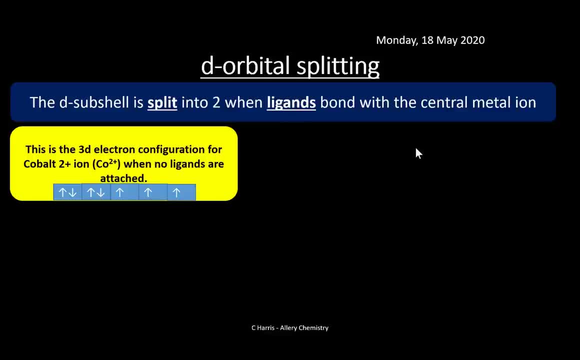 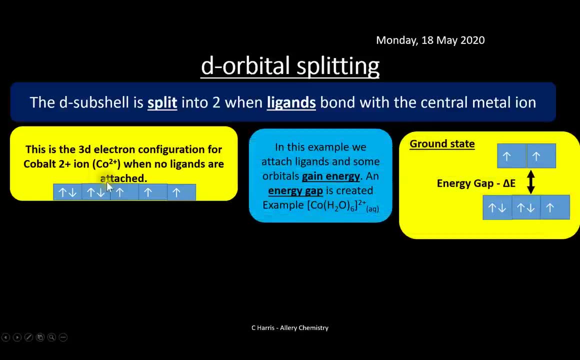 the d orbital then splits, uh, and we get two different energy levels. so you can see um. if we bond um six water ligands to this cobalt iron, we then end up with a, with a d orbital that's split into three on the bottom and two on the top, and we have an energy gap in between. this is delta e. 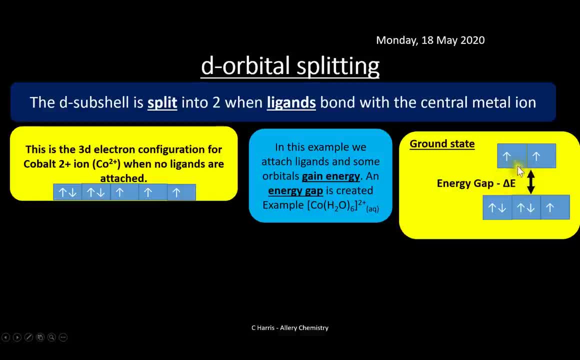 okay, um, and so basically, um, orbitals gain energy when we, when we add uh ligands to it, and so it splits in this way. okay, and so when electrons absorb light energy, some of them move from the lowest energy state- this is the ground state, as you can see here- and some of them move to a higher energy level. 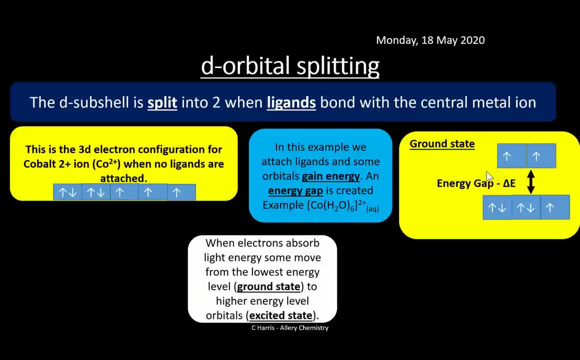 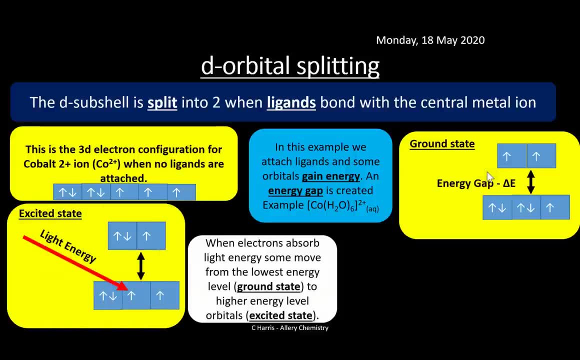 orbitals, which is called an excited state. so let's have a look and see how that looks. so there it is. so excited state is effectively where, if we have an external energy supply that could be visible light, for example, so light energy- and this energy is then used to. 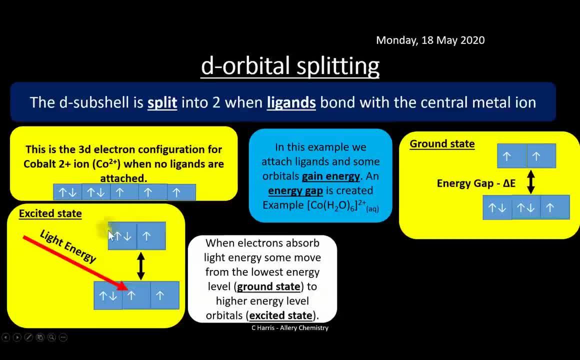 excite an electron in the lower orbital and a one up into the top here. okay, and this actually explains why. if you didn't have, so you look at is a scandium and zinc that we looked at before. they weren't transition elements because they don't have a partially filled d subshell you need. 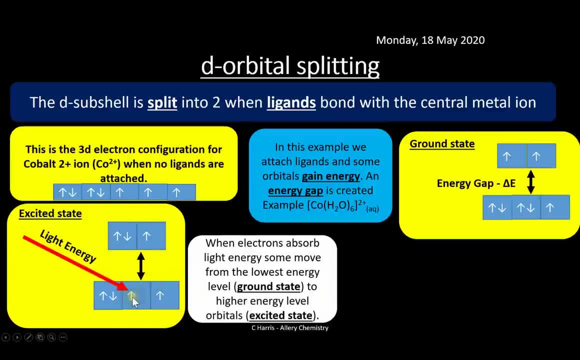 a partially filled d subshell for this to occur, for an electron to effectively transist from one orbital to the other, okay, and if it doesn't, if there's no electrons at all, obviously you can't do that. but if it's full um, like zinc is um, if it's a full uh electron shell, then obviously you. 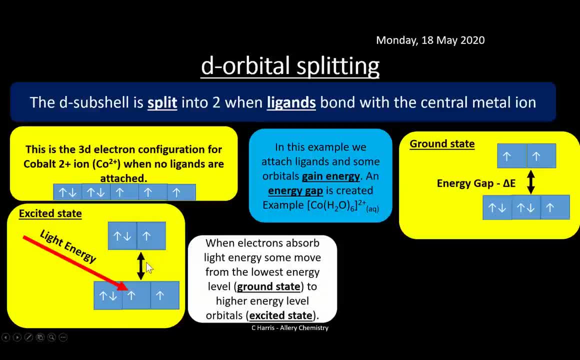 can't. if these are full at the top here you can't move any up or down, so that's why they're not transition. well, so it all stems down to this. so in order, like, say, for order for an electron to be migrated up into the higher energy level, then um the uh, the energy must. 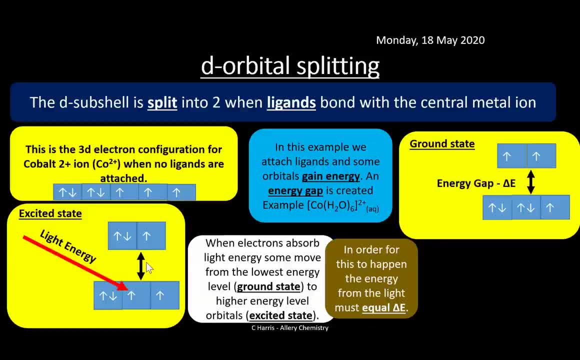 the energy of the light must equal delta e. okay, very important. so the size of delta e is dependent on. so that how big that gap is is dependent on the central uh metal ion and its oxidation state. so depending on what the metal ion is, that will depend on the size of that and the type of ligand. 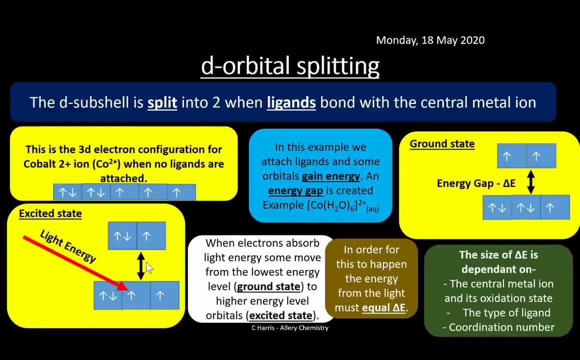 that's bonded on there, whether it's a water ligand, it might be ammonia ligand, a hydroxide ligand or which minus, and also the coordination number. so remember that's the shape of the molecule, so the number of coordinate bonds around the central metal ion. so whether that's octahedral, tetrahedral, 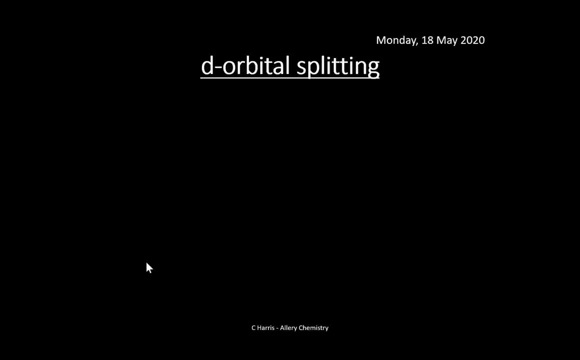 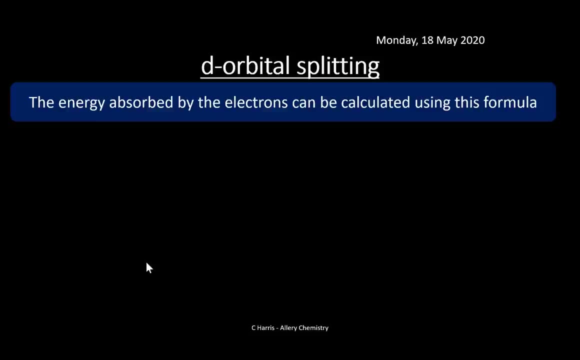 square planar, etc. okay, so the energy absorbed by the electrons can be calculated using this formula. so here's the physics bit. so if you do physics, um, you will have seen this formula before, but if you haven't, i'm going to break it down. i'm going to tell you what each bit means. 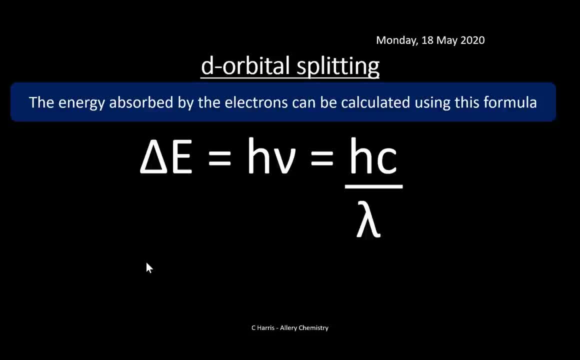 so this is it here, okay. so it's got um, it's broken down, it's equated into different steps. so e, delta, e is the change in energy in joules, uh, h is planck's constant, which is 6.63 times over 10 to the minus 34.. you don't need to remember that number. you will be given that in. 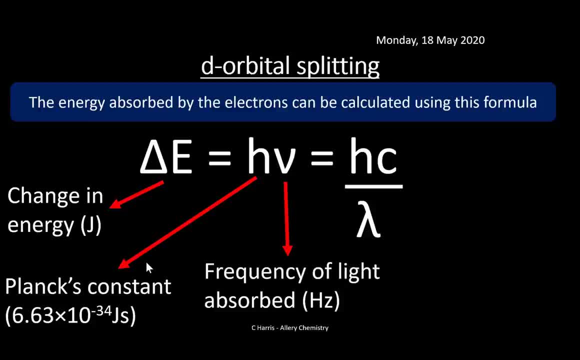 the exam um. mu is the frequency of light, um which is measured in hertz, uh, and obviously lambda is the wavelength of light that's been absorbed in in meters um and then, and the speed of light is three times ten to the eight meters per second. so that's c okay. so what we're going to do is we're going to use this to try and work out um. 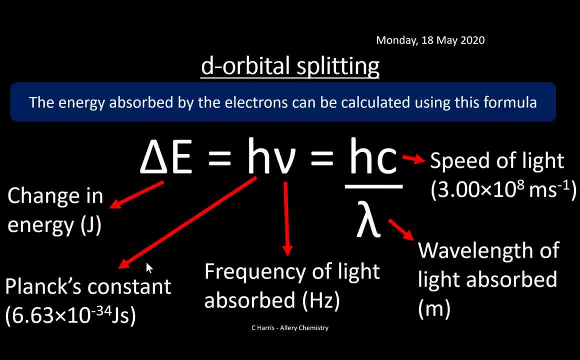 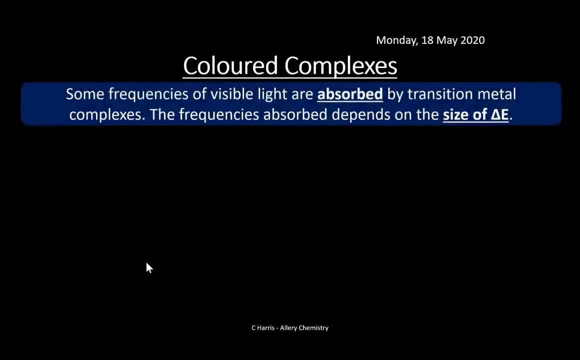 well, you will be required to um, you know, to use this formula to work out, say you know, wave length or speed. it won't be speed of light, but or it could be energy, for example energy change. so you will be expected to do this, okay, so so some frequencies of visible light are absorbed by 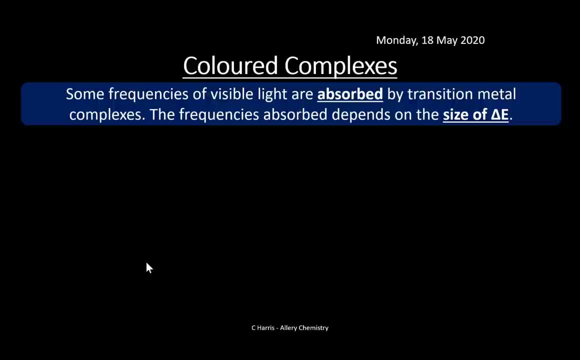 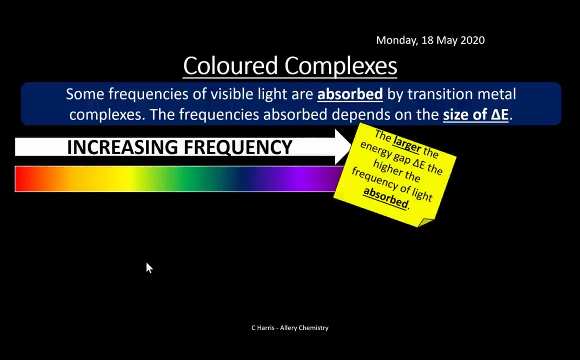 the transition metal complexes, and so the frequencies absorbed depends on the size of the delta e. okay, that's your change in energy member between the the split d orbitals. so what's important is to equate a frequency and energy together. okay, so you can see here that as we go um from, you might have seen this as well. 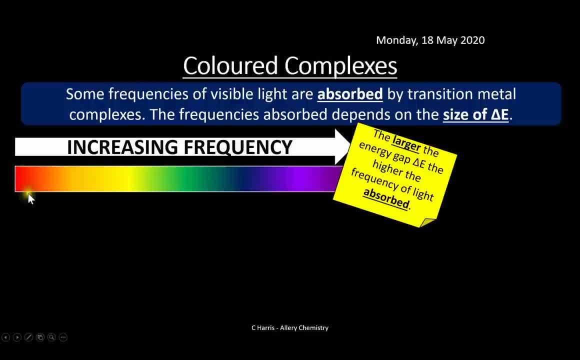 from um. you know a cannon from physics. red um has the lowest frequency, which is the red color here, whereas the violet and purple colors at the top there have a lower frequency. so we can talk about a higher frequency now. the larger the energy gap, that's delta e, the higher the frequency of light. 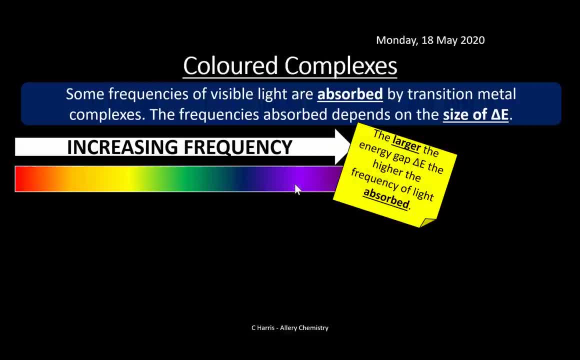 that is absorbed. okay, so we have um the. obviously we've got white light that comes through through the window, let's say um one of these frequencies of white light, so one of them is absorbed by the complex that we're looking at. okay, so bear with me here. okay, so if you study physics, this might. 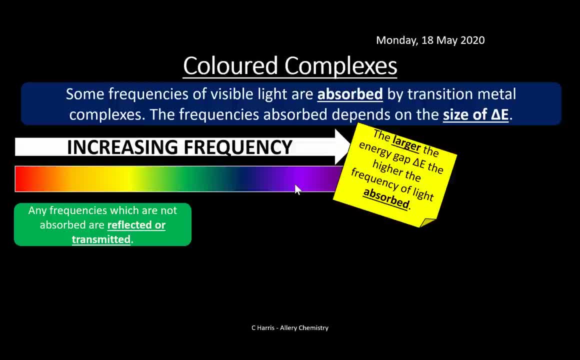 be really straightforward, but a lot of people don't study physics, so i'm going to go through this and break this down a little bit more. so any frequencies which are not absorbed are reflected or transmitted. okay, so only one of them: frequencies out of that band there is absorbed. 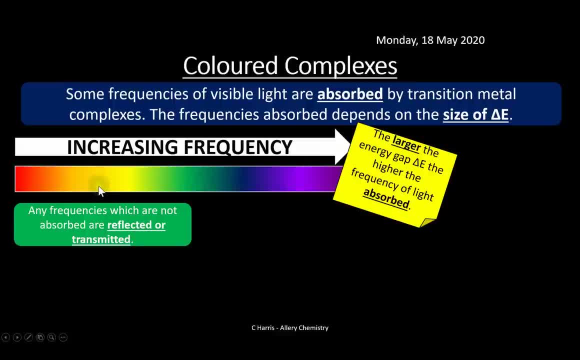 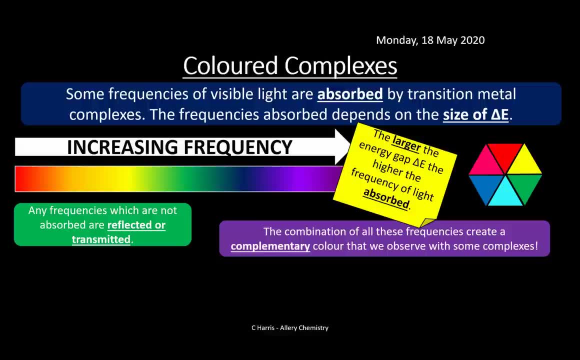 the other ones? um, the other ones are actually reflected or transmitted. okay, so the combination of all of these frequencies creates a complementary color that we observe, that we observe with some complexes. we're going to look at that later. uh, later on in the video, when we look at the complementary colors a little bit more detail. okay, so, for example, here's an. 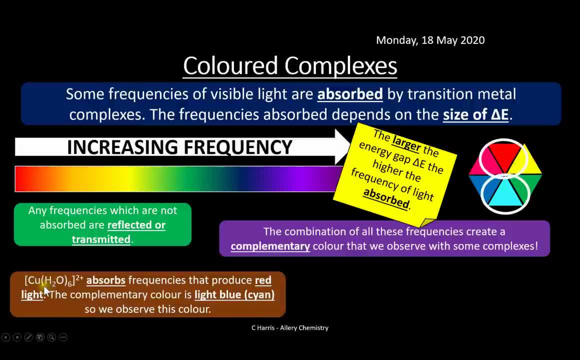 example, which is copper with six hexa aqua copper complex. trying to say that one quick. and this absorbs frequencies that produce red light, so it absorbs red. okay, so that's the color. it absorbs all the other colors in the spectrum, so it absorbs this one. so a mixture of all these colors are not. 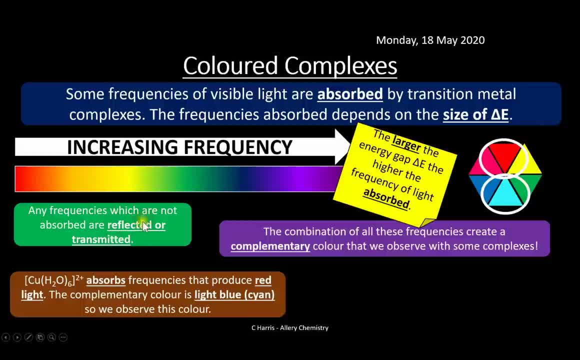 absorbed are reflected or transmitted back, depending on the type of complex um and the color. if we mix all them colors together, we get cyan, so that's the complementary color that we see, so it absorbs red, but we see cyan, so we see it as a cyan color and indeed if you look at copper um, so you might have. 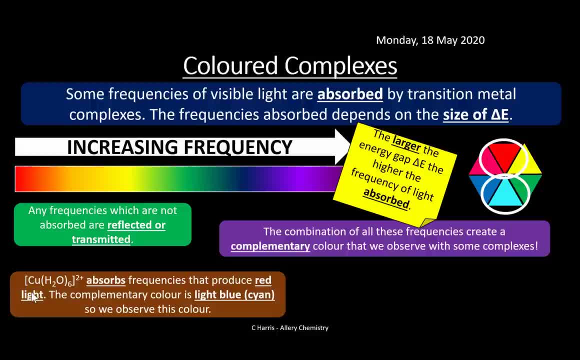 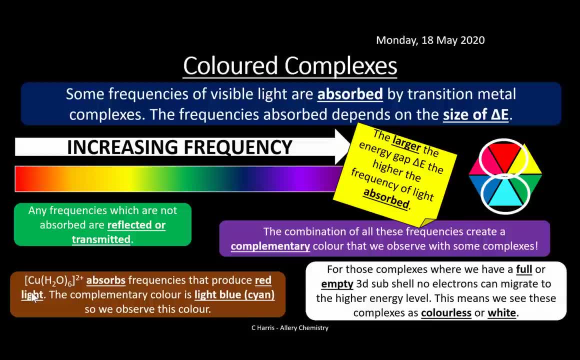 done a copper sulfate crystals, for example, um in in one of your lessons, um, then copper is a pale blue color. so that's what we see. so it's cyan, okay. so for those complexes where we have a full or empty 3d subshell, then no electrons. remember i said this before: no electrons can. 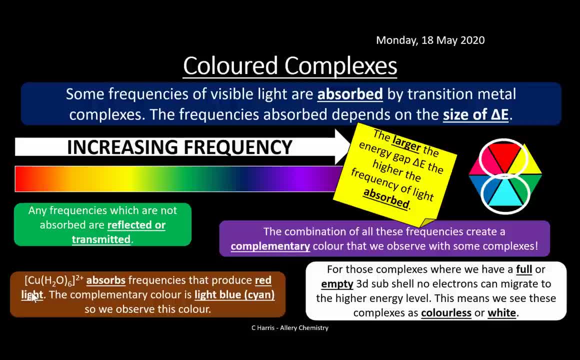 actually migrate to the higher energy level. so your things like zinc and scandium, uh complexes. so when they um, dissolve them water, excuse me um. and when they're dissolved in water and the six water ligands surround them, then they actually form colorless or white, um, white. 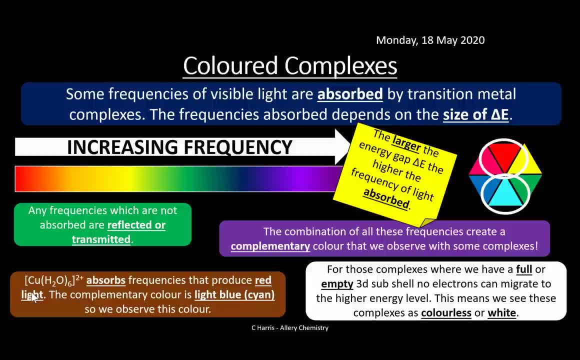 compounds or colorless solutions. they don't have any color um associated with them because there's space for electrons to migrate, or no electrons at all- to go from that lower uh d orbital to the higher d orbital um. you know the the orbitals in there, from d um, the orbital splitting. 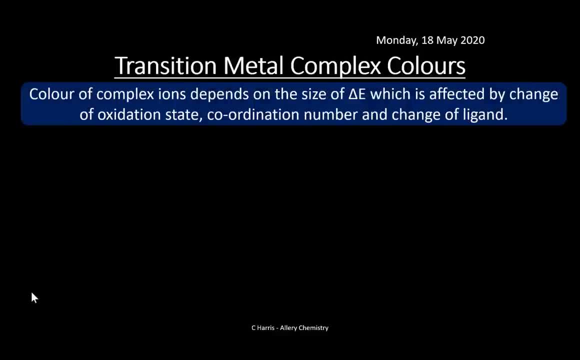 okay, so the color of complex ions depends on the size of delta e, which is affected by change of oxidation state, coordination number and the change of ligand. okay, so the delta e, remember, is changed by all of them different. the size of delta is changed, is is determined by them different factors. okay, so let's have a look. 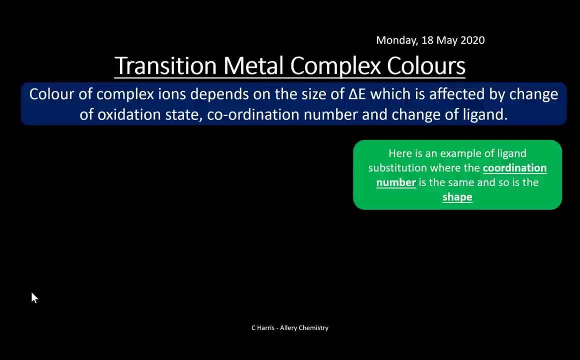 at an example of ligand substitution where the coordination number. you'll see more ligand substitution in the next topic. they are very similar, these topics, by the way, and so where the coordination number is the same, and so is the shape. so let's have a look. so we've got cobalt here. 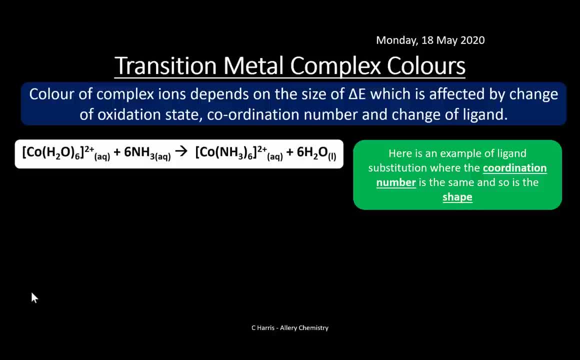 so we've got cobalt with six water ligands surrounding it. okay, um, and it's going to. we're going to react it with ammonia. so we're keeping the shape the same, but we're changing the ligand. so you can see here, for example, hexa aqua cobalt complex is pink and 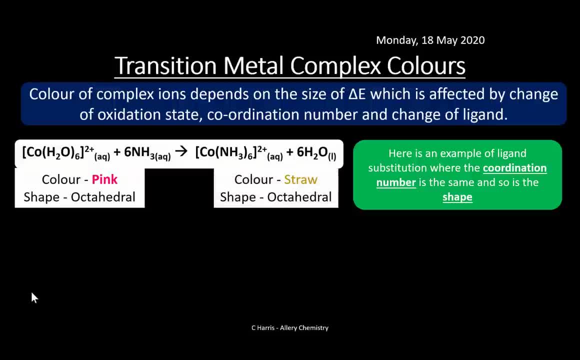 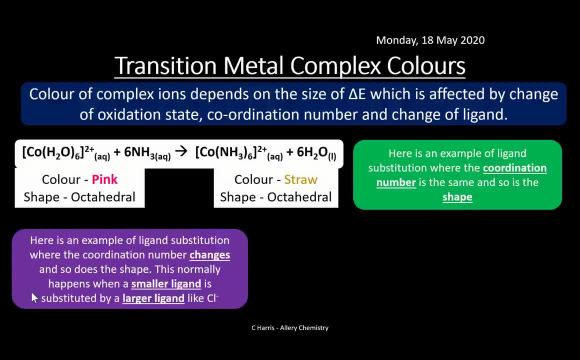 it's octahedral, but with ammonia it's straw and octahedral. so you can see the ligand has an impact on the color because the type of ligand impacts delta e, and so here's an example of ligand substitution where the coordination number does change, so obviously the shape will change as a. 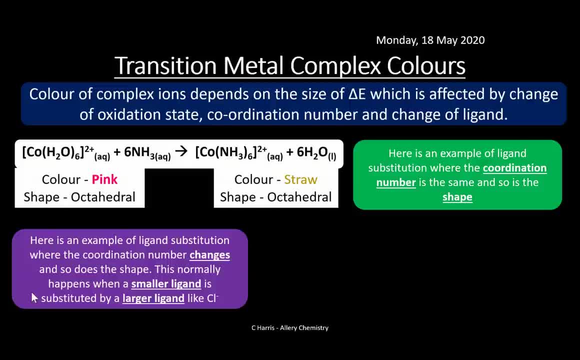 consequence, um, and this normally happens when we're taking a smaller ligand and substituting for bigger ligands, such as such as your chloride ion. so you can see here that we've got our copper hexa aqua complex, which is octahedral and pale blue. 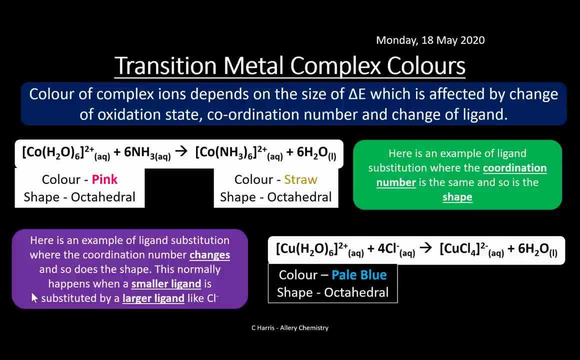 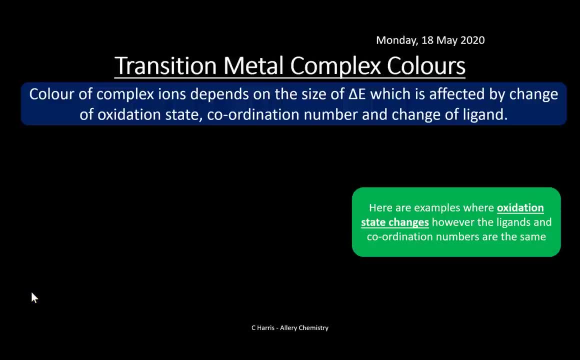 but then once we substitute the six water ligands for bigger ligands- so that's chloride ligands, but also we're changing the shape- that will also have an impact on color as well. so obviously this is yellow and the shape is tetrahedral. okay, so let's have a look at an example where the oxidation 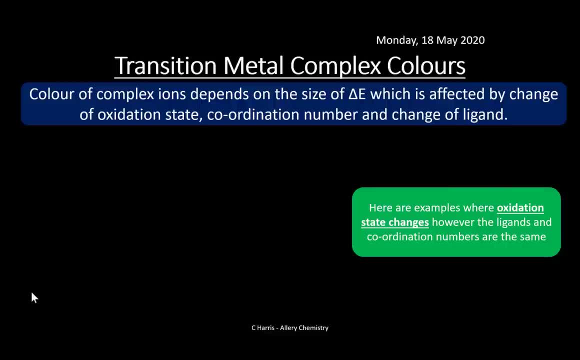 state is changing. so remember there's three ways. so we've looked at the coordination number changes the ligand. so this is where we're looking at oxidation number. so you can see, here we've got iron uh going to iron three, plus the ligands are the same, the shape is the same, so one's octahedral. 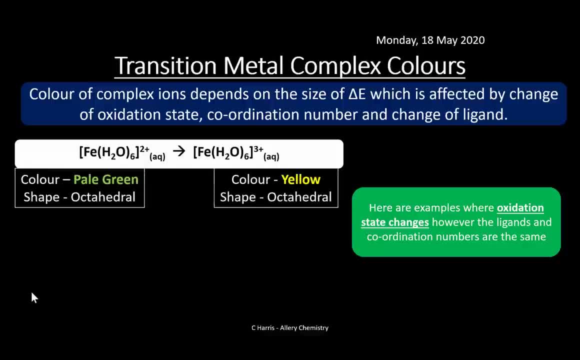 and pale, pale green. the other one is also octahedral, with the same ligand, but it's yellow. so the oxidation state of the transition metal has clearly had an impact on the color and obviously hence delta e as well. here's another one. this is vanadium. uh, again same, uh, same system: vanadium. 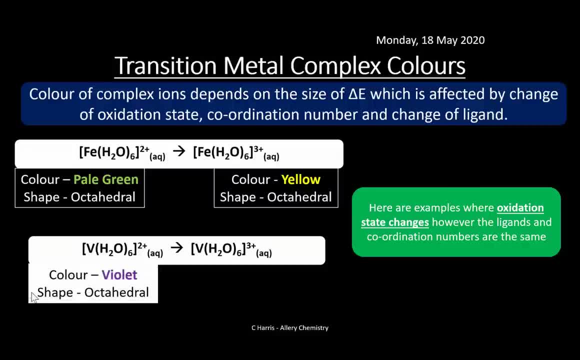 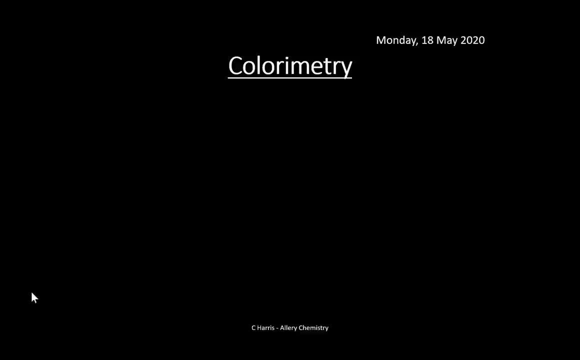 two plus to vanadium, three plus um. the color here is violet and octahedral. the color here is green and octahedral. so what's impacted, that is, the um, is the type of- uh sorry, is the oxidation state of the transition metal in the middle. okay, so we're going to look at how do we actually um measure. 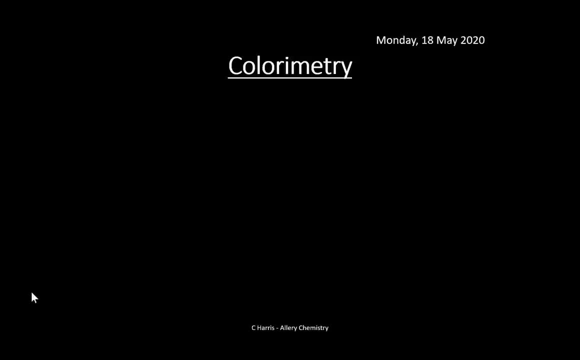 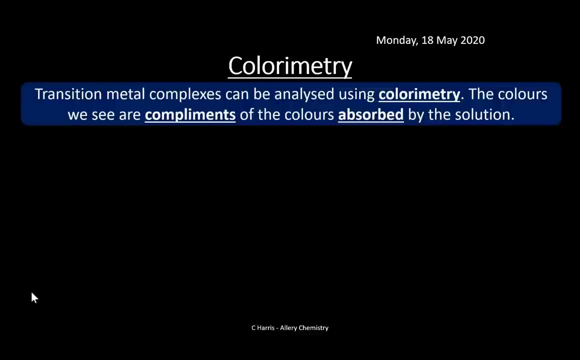 these, or can we measure the um concentration of a substance, of these colored substances? and we can. we can use something called colorimetry, which is lovely. um, so your transition metal complexes, these can be analyzed using colorimetry, and the colors um we see are um complements of the colors absorbed by the solution. remember so if it. 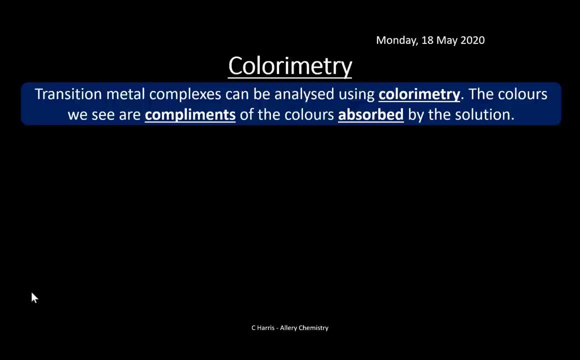 absorbs red, and then we see the color. that's the combination of all the other colors in white light. okay, so that's what's transmitted or reflected. so remember, just as a bit of a recap, that white light, um, obviously, white light is made up of the colors that we see above, um, so when it hits the transition, 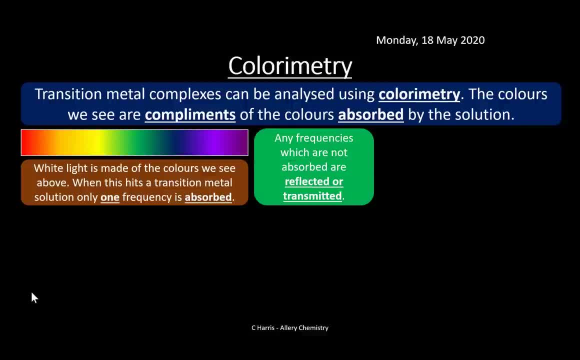 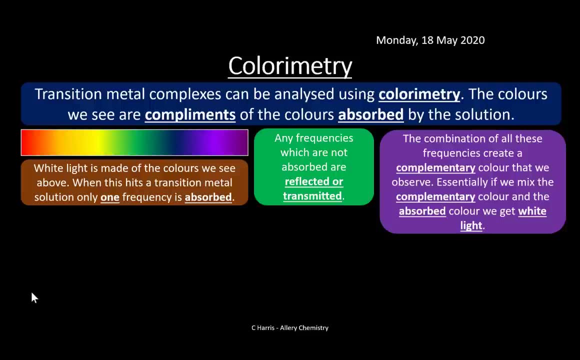 metal, only one of the frequencies is absorbed. so just remember and so remember. all the rest are reflected or transmitted. so we've seen that already and obviously the combination of these creates that complementary color and that's the color, that um, that we see. so if like say, look, using that color, 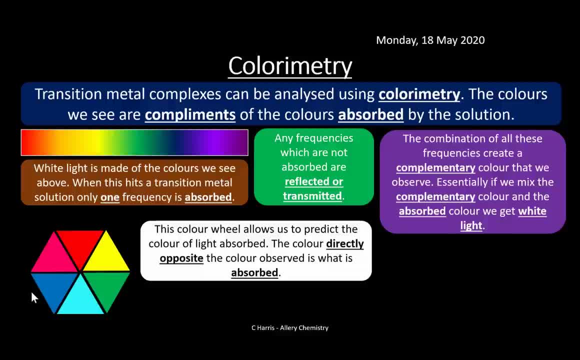 wheel, like we've seen before, um. it just allows us to predict the color absorbed, and the color directly opposite is the one which has been absorbed. so, for example, if we look at um, a green color is observed. this would mean that magenta is actually being absorbed. so if we look at the 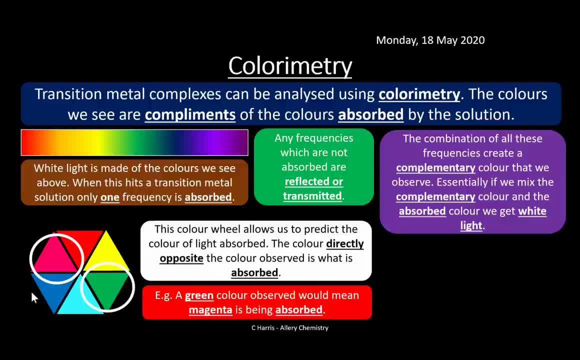 color that's being absorbed, so the magenta of that spectrum is being absorbed. then all the other colors mixed together would be the one that we see. so, for example, if we look at this, there's your magenta color that's absorbed, so it's a combination of that, that color and all of these colors here. if 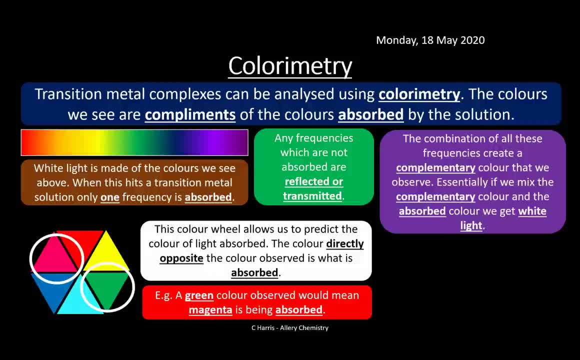 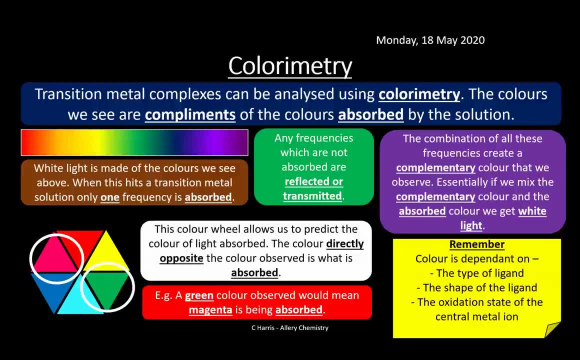 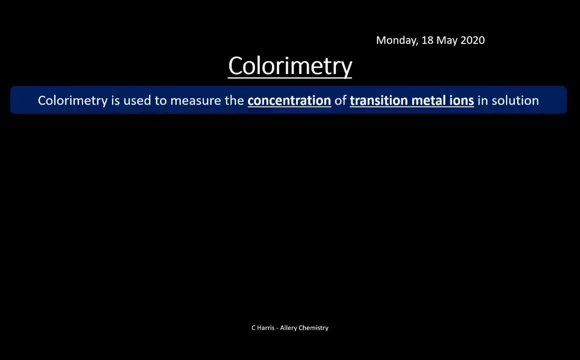 you mix them all together that we get green, okay, so that's, that's the color that we observe. so, just as a reminder, remember it's these things which determine the color here. okay, so let's have a look at, um, let's have a look at how we can actually, like i say, measure the concentration of the transition. 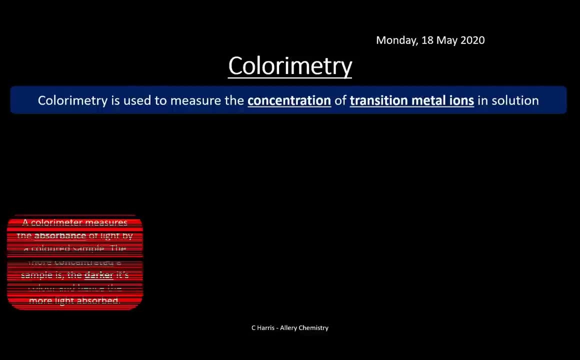 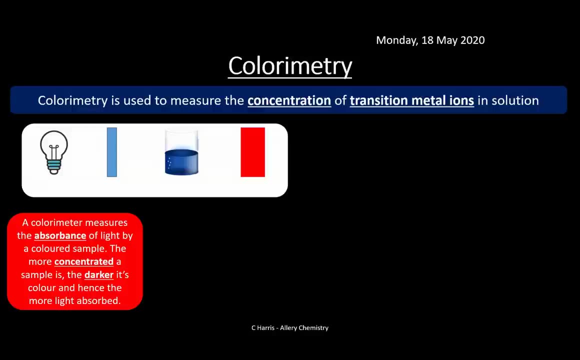 metal ions in solution, and we can do that using an instrument called colorimetry, which is, like i say, which is um, a machine that basically measures absorbance of light. um, so, um, basically, the idea is that the more concentrated your solution is, that you're testing the um the the darker it is. 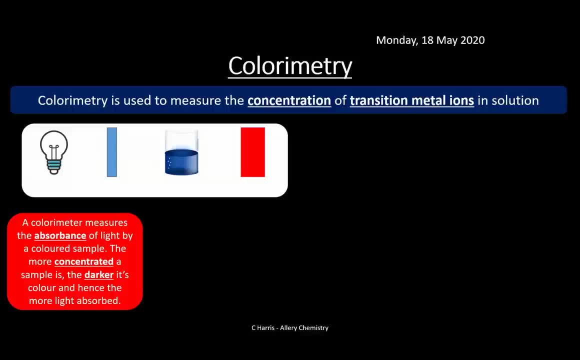 and therefore the more light that is absorbed. and these machines basically measure absorptivity of your um, of your substance. okay, so more light is absorbed if it's darker. so the colorimeter, remember it, must be set to zero. and what we do um, we basically calibrate it um and we we measure the. 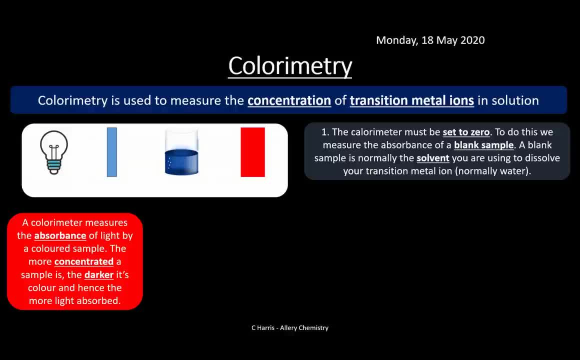 absorbance of a blank sample. okay, so a blank sample is normally a solvent we're dissolving in, so that solvent could be water, for example. so we're shining the light through the sample of the solvent that we're using, um. so, for example, water, and we measure the absorptivity. clearly it's. 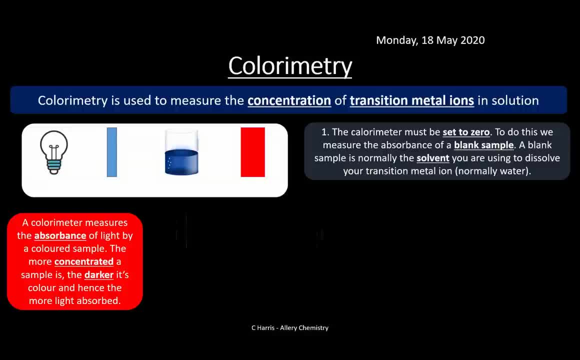 colorless. so there's not going to be much absorptivity at all, not much absorption of light. so white light is is filtered into a narrow range of frequencies. okay, so we call it monochromatic light. um is produced. okay, so you've got your white light here, um, and obviously that goes through, um hits your filter and is narrowed down. 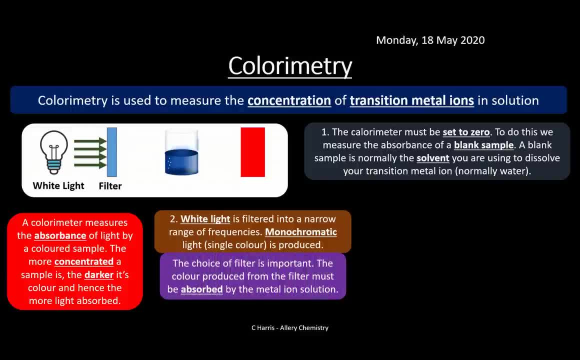 and so the choice of filter is important. what we need to do is the color produced from the filter must be absorbed by the metal ion solution, okay, so whatever color is being used, that must be removed. so that's why we're showing just a similar example of a UV light. that's exactly what we're. 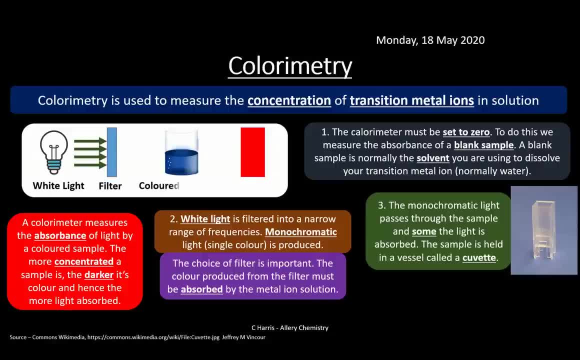 using here, um, for example. so it's a light which we call an arduino, but we're using the blue light to make it, um, dim, conversely. so what we're doing is we're going to be using the arduino to make that dim versus dim. so that's going to be a really interesting example of a. you might have seen these, you might have got one of these at school or college, um. but you put your sample into something called a cuvette and the cuvette um is basically the um where you put your sample in the cuvette. now, the cuvette's got an interesting design. it's obviously square, but also it has two frosted sides and two colorless sides or clear sides. what you want to do is shine the light or point the colorless side where the light's going through. the frosted sides are there, so this: 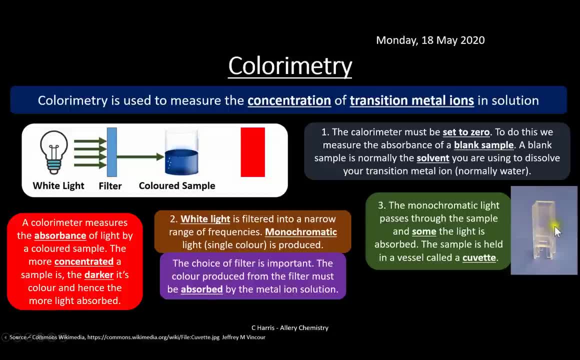 is where you can pick it up, because what you don't want is to pick it up on the on the colorless side, because you get fingerprints all over that and of course they- obviously the oils in your skin- can be- uh, impact the absorptivity as well. so you want that. you want the sides of this cuvette to be. 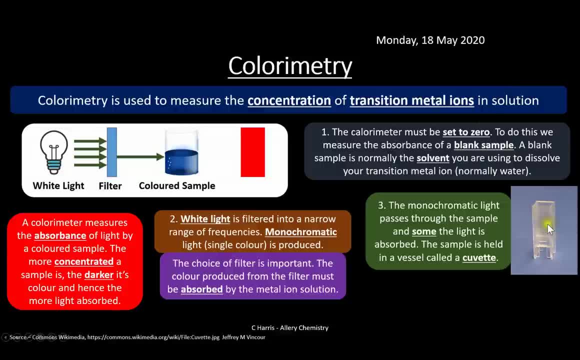 completely colorless and you want this to be obviously frosted. okay, so that's where you hold your sample and effectively- um, obviously the light is. then goes to the filter. it goes, this monochromatic light here goes through the sample. obviously, some of the colors absorbed the color. 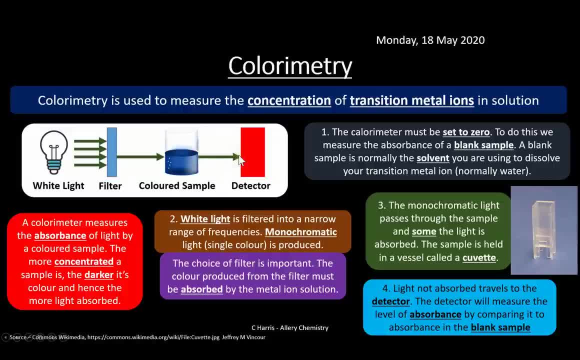 that goes through the filter was absorbed, and then all the rest of the colors is then reflected out, um, out on the side and hitting the detector and basically, um, the detector is, um, is measuring how much of this monochromatic light has been absorbed by the color here and how much is. 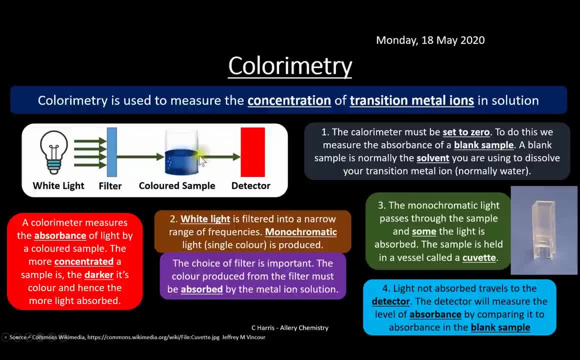 actually coming out to the other side and clearly, the more concentrated this is, the less light's going to come out here. okay, and we do that by measuring against the blank samples. remember this is dissolved in a solvent. this could be water, and we have the value of our blank sample already, so we just minus the two so the the detector will. 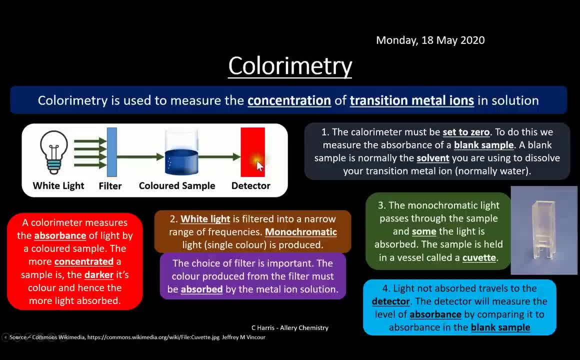 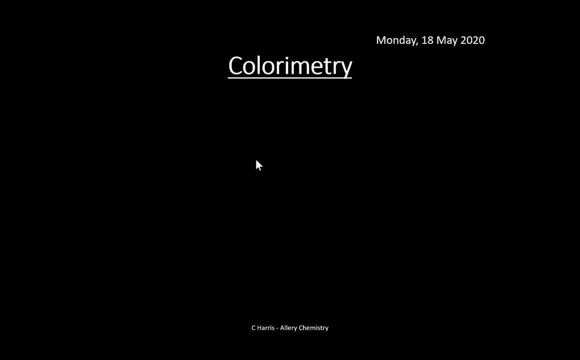 know if there was any absorptivity, because the solvent it will take that into account when it reads it. okay, so, um, we really use the data from colorimetry machines, um, to actually measure the concentration, but what we've got to do is is draw a calibration graph first before we actually do. 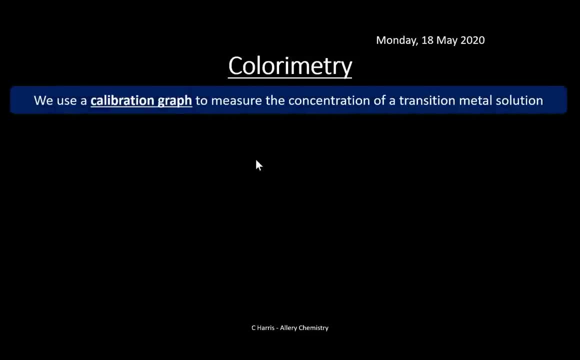 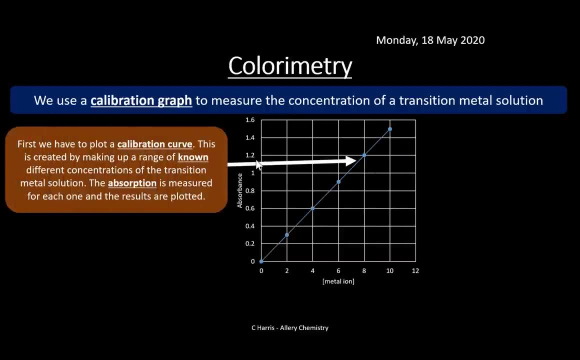 that. so a calibration graph is used to measure the concentration of your transition metal solution. so, um, you can see, we've got a calibration graph here and so we plot this and it's basically created by making up a range of known different concentrations of this, of the transition metal solution and the absorption. 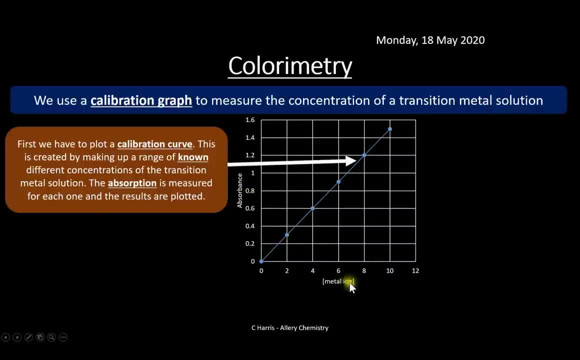 effectively here. so this is the absorption. you've got a graph of absorbance against the concentration of metalline. basically it's plotted for each one. so we, we make up a range of different solutions at no point, though, so we plot the graph Sahib here. so it's basically a process is created for each one. so we, we make up a range of different solutions at no point on which. Why does revenues go away? That's the question: How do you solve up those concentrations? 그거 våra nad zelente 있는데. Two79 therapy. 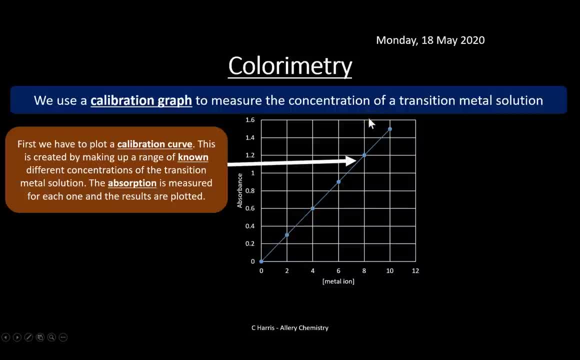 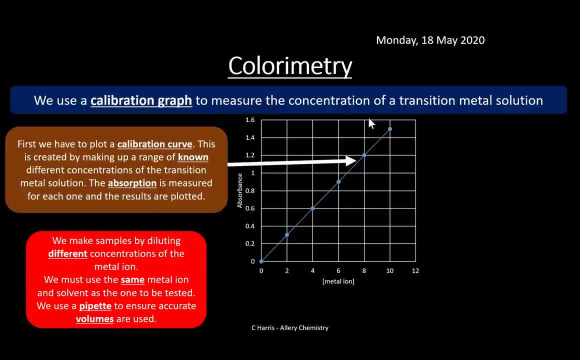 concentrations. we just plot them on this graph. so we've got a reference now, and so then what we do is then: obviously we make the samples by diluting different concentrations of the metal line. okay, so we dissolve that into the solution and we must use the same met line tested. that's really. 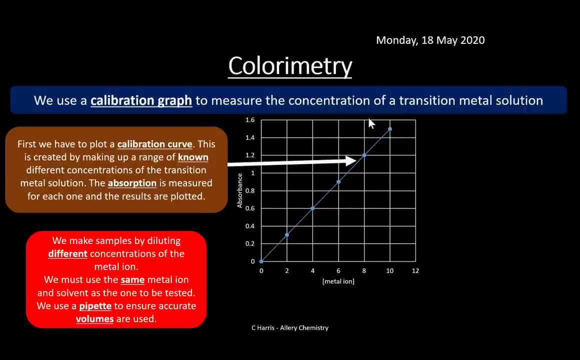 important and we use a pipette to measure it accurately, to measure the volumes accurately, and obviously we then put them into the colorimetry machine and then what we then do is then test the sample we want to know the concentration of by measuring the absorbent. so we've got the sample. 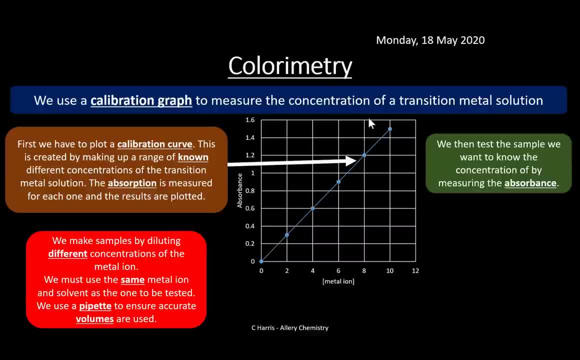 we're going to measure the absorbance and then we're going to use the graph to measure the concentration. so, for example, if our sample under test has an absorbance of 0.7, then we're going to get a concentration of somewhere around four and a half. so we're using that calibration graph. 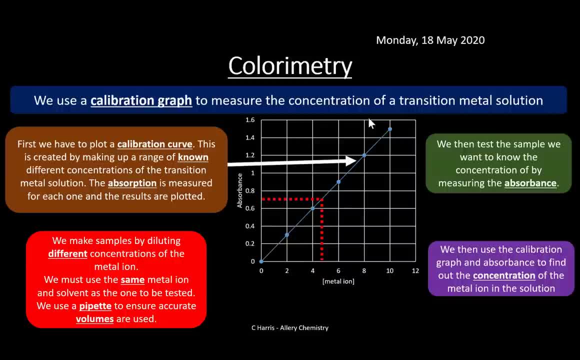 of. obviously, the, the calibration chemicals is the same as what we're going to be testing, okay, but we use the graph to to measure the concentration. so it's, it's fairly straightforward. um, you know it's, uh, it's, it's about plotting results of known samples and 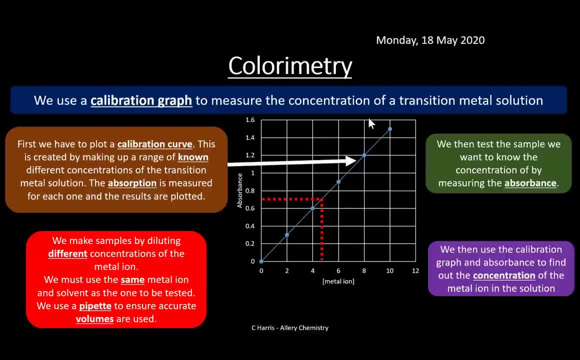 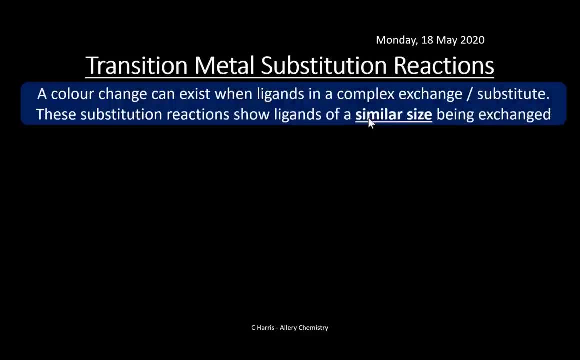 then using it to work out the concentration of your unknown one. okay, so let's look at some reactions of uh transition metals. so we're going to look at some substitution reactions and basically a color change can exist when ligands in a complex exchange or substitute. okay, and so. 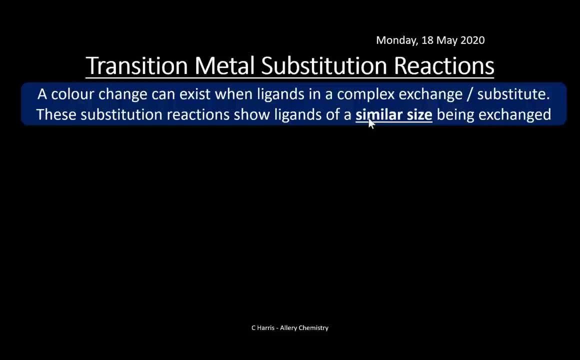 these substitution reactions show ligands of a similar size being exchanged in the example here. okay, so let's have a look at the first one. so we're going to look at a cobalt example here. so we've got cobalt with six waters. notice the difference here: we've got cobalts with six. 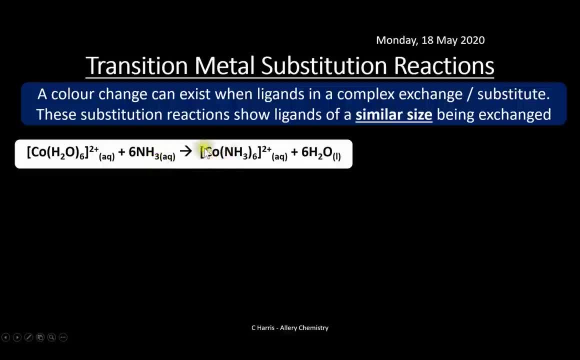 waters. we're going to react that with six ammonia ligands and what we're going to form is our ammonia, hexa, ammonia complex here. okay, still the same charge, because ammonia and water all don't have a charge on their own and obviously the six waters have been displaced. so the color changes here this: 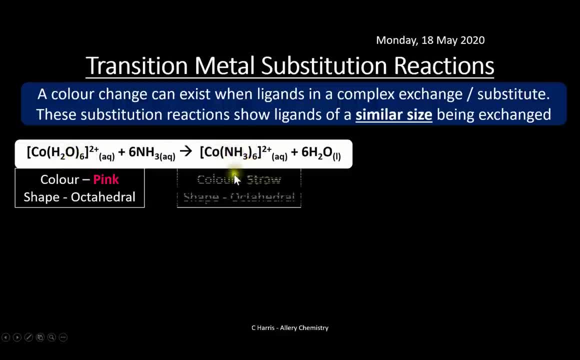 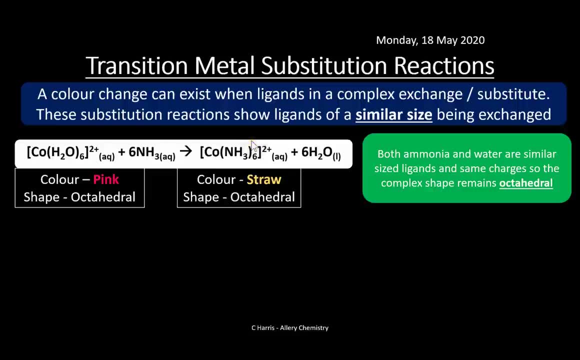 is a lovely pink color and this is a straw color and this is a light pink color and this is a light color cobalt. with your six, they go six ammonia ligands, um, around the side. so both ammonia and water are similar size ligands, and so the charges, uh on the complex remains, um, remains the same. 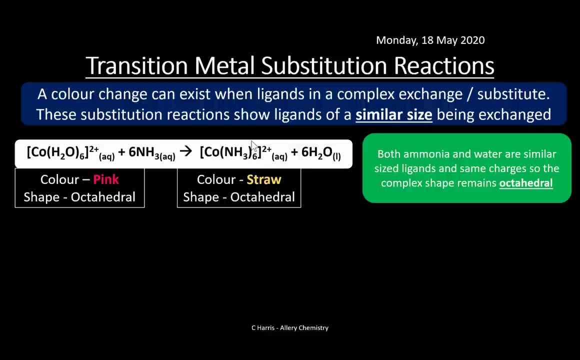 but also the. the shape remains the same as well. they're both octahedral, so the color change, like we've seen before coming from this is because of the ligands changing. so here's another example of a metal, a transition metal, substitution reaction. so here we have six water ligands. okay. 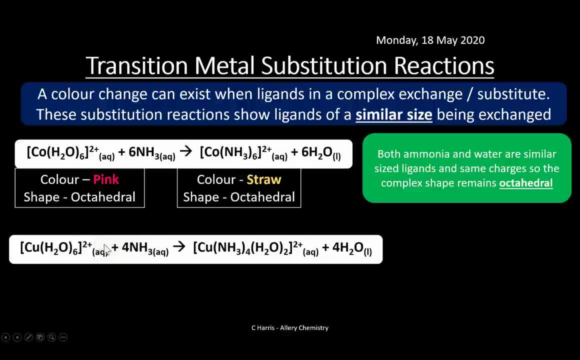 uh, we're going to react it with ammonia, and this is slightly different in the fact that you actually get a partial substitution with copper. so you need to be aware of this. so, unlike cobalt, where you get a full substitution here. so basically all the waters are substituted for the ammonia, here only. 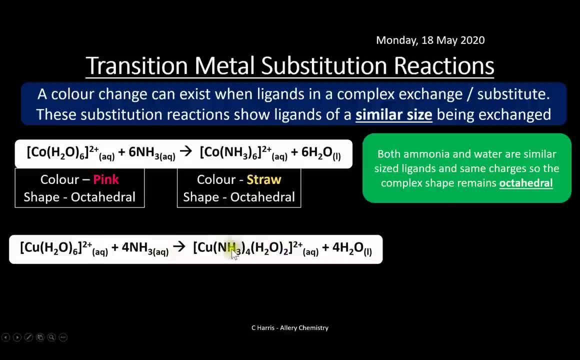 four of them are. so the axial, uh water ligands remain the same, so you've only got a partial substitution here. four of the ammonias add into the complex there and we've got two water ligands left. so the colors: this is a nice blue color, uh, on this. 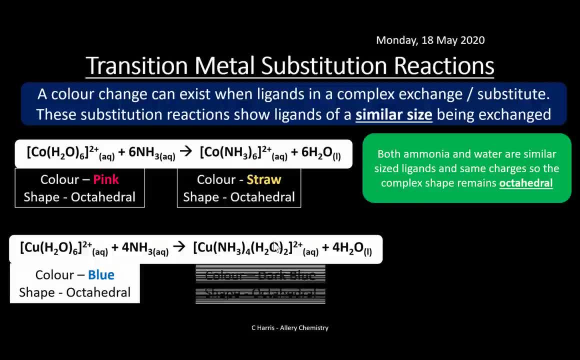 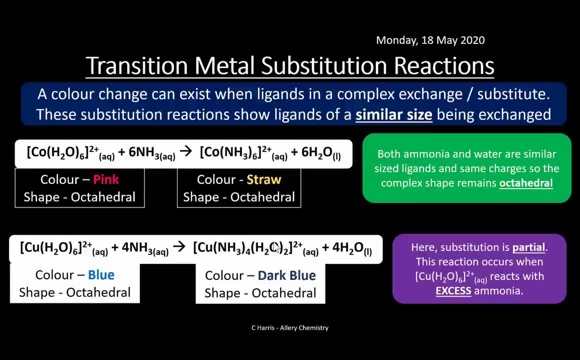 side. so that's your, obviously your copper. two plus and we get a nice royal blue, really dark blue. on this side, the shape remains the same, um, but um, here it's a. we get a partial substitution, uh, instead, so, um, this is all these examples. here we're reacting it with excess ammonia. 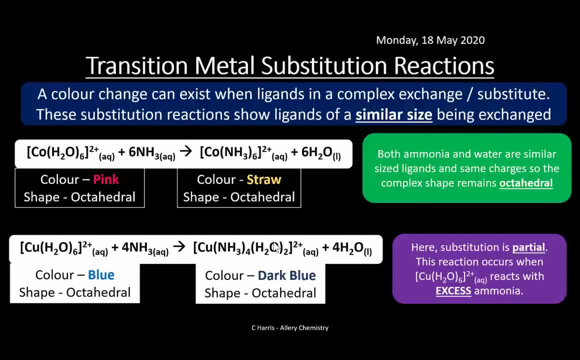 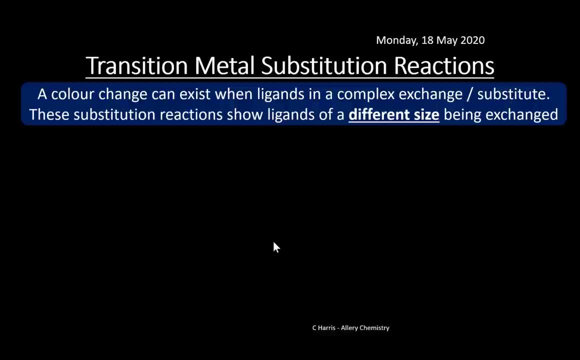 okay, so there's a plenty supply of ammonia for these reactions to to work. okay, so we're going to do the same, but this time we're going to look at um- ligands of a different size being exchanged- and and um. basically, you need to be aware of these reactions that i'm going to go through here, so remember your. 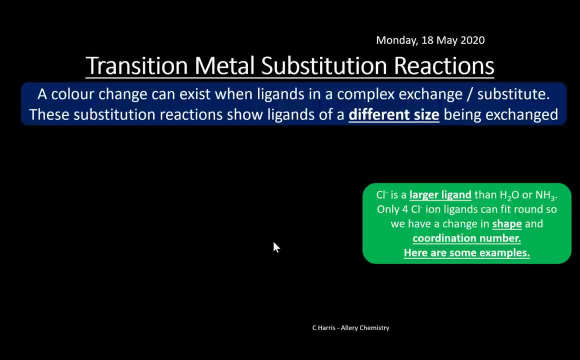 chloride ligand is bigger than water or ammonia, so we can only fit four of them around that central metal line. so here the coordination number is changing and hence the shape is changing as well. so let's have a look at a cobalt example again, but this time we're going to be exchanging it. 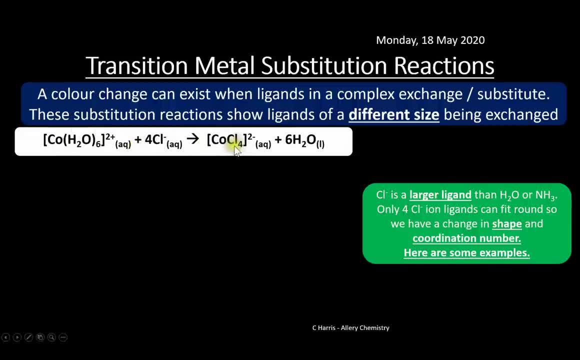 with chloride ligands and effectively, what happens is all the water ligands are displaced, but we only have four chloride ligands here and obviously six waters. so this is a pink color here, um, and this is a blue color which is your cobalt, um, cobalt chloride, cocl4 um. octahedral, tetrahedral. 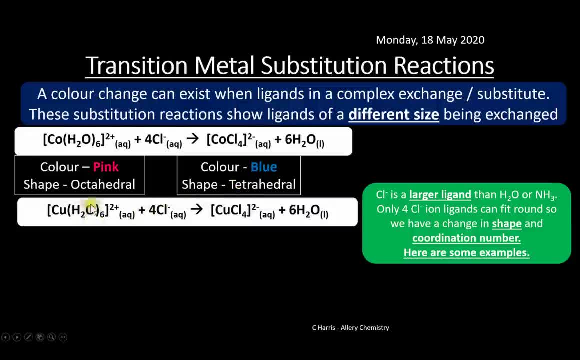 okay, here's another example. this is copper um. this time we've got our six water ligands, um, and a chloride ligand, and you can see here that, because it's bigger, we only have four of them around there exactly the same. so we've got blue and that's going to yellow. 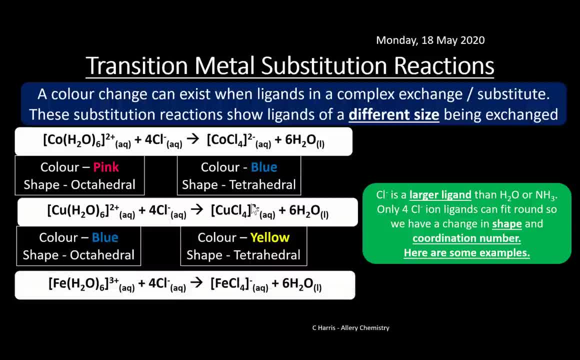 and just for another example here, this is iron three plus, again, reaction to chloride ligands, and we get a yellow and a yellow shape here, yellow color here, so you can see both of these are yellowish in color, um, but the shape has actually changed here. so you can see, all this is all these. 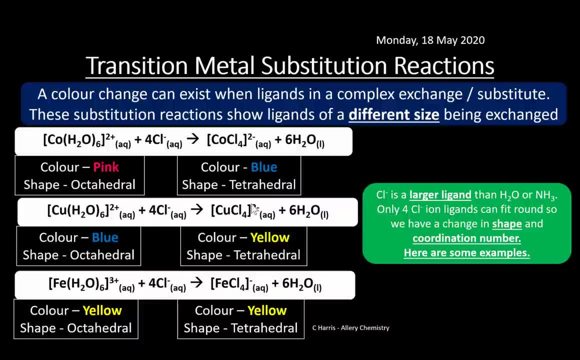 reactions are is we're just using a bigger ligand. we can't fit as many of them around, so it's just showing the reactions. nothing new here, it's just the reactions. um, the reactions are new, obviously, but the actual principles in terms of the size of the ligand you've seen earlier on in the video. 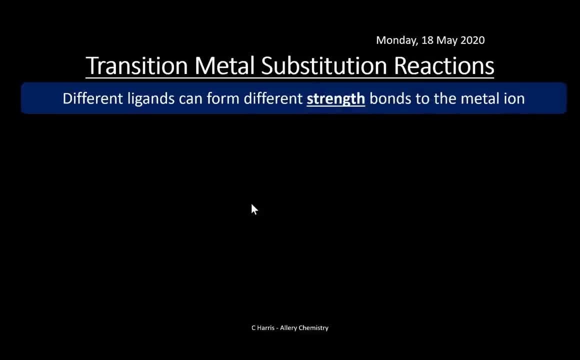 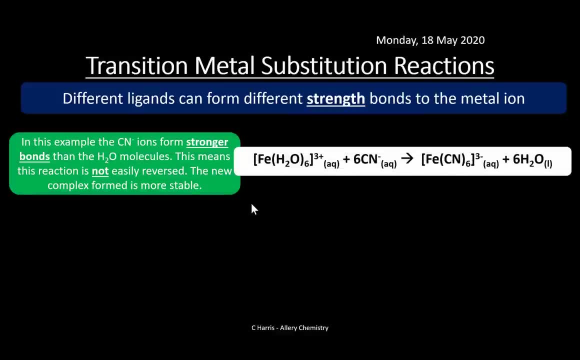 so different ligands can form different strength bonds to the metal line, um, as we'd obviously, as we'd seen before with hemoglobin. so you can see in this example um, here the cyanide ligands, these form stronger bonds than the water molecules that were originally attached to the iron, and so this means this. 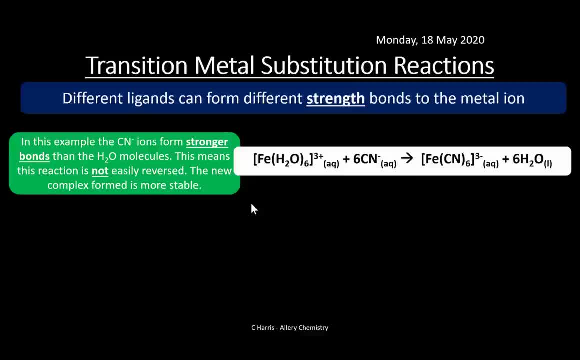 reaction is not easily reversed, and so the new complex that's formed is actually more stable. this complex in particular- now this is a bit of a bit of kind of interesting fact- um, the in your salt. if you look at the package of salt, salt has an anti, anti-caking agent in there. basically, it stops the salt from clumping. 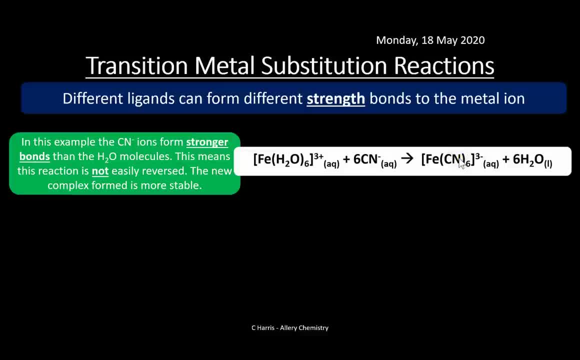 together when it comes into contact with, uh, with water. so you can see here that, um, this is the actual. if you look on the back of the packet, this is the anti-caking agent. it has the cyanide ligand on it. now you might think, crikey, that's quite, that's quite drastic, because 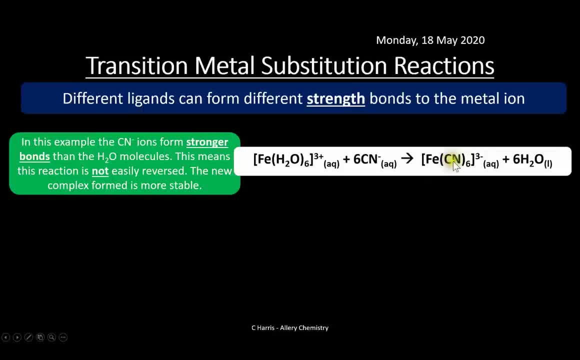 cyanide will kill you, definitely. but because this ligand bonds so well to the iron in the middle, um, it doesn't break apart when you eat it, so it just gets passed out as waste. so there you go. so have a look at the back of pack the salt and you'll see, um, your hexacyano ferrous complex in there. so obviously iron complex. 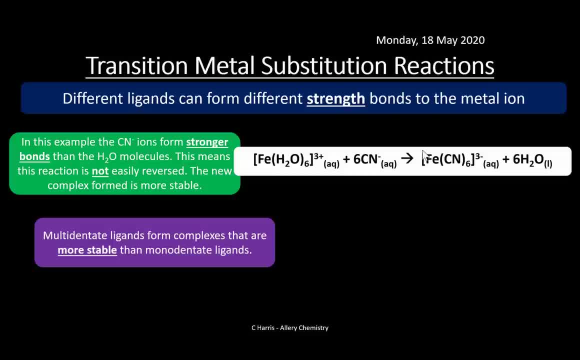 a little bit of interesting fact there- and also another thing as well- is that multi-dentate ligand- um, remember, these are your bidentate bidentate ligands as well, but your multidentate ligands are things like edta and heme. these form complex that are much more stable than monodentate ligands. 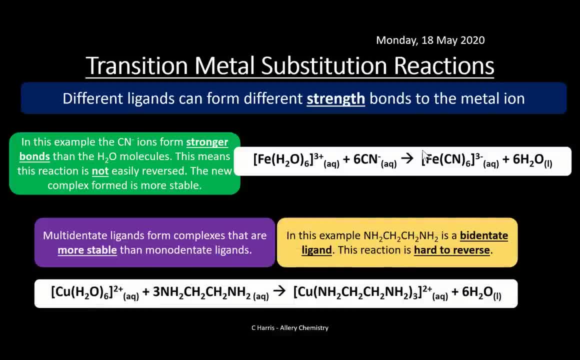 because they're more stable. um, they actually, um, obviously they, they form, uh, complexes are more stable. it's really hard to reverse these reactions. so you can see, here you've got your copper with your six waters around it. okay, around the copper ion, um, oh, the, yeah, the copper ion, the metal ion. 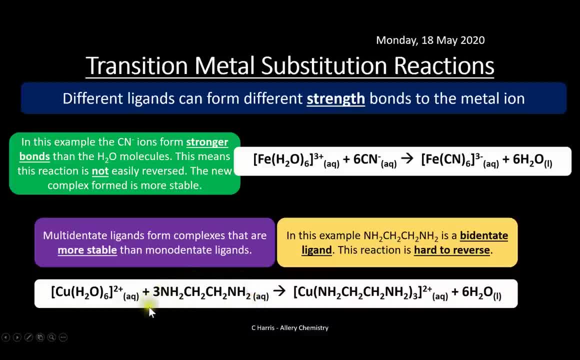 in the middle, and here we're using a bidentate ligand here in this case. so we've got three of these and what happens is all six water molecules are kicked off and they're completely substituted for bidentate bidentate ligand here. this is a lot more stable than this complex here. so this is why. 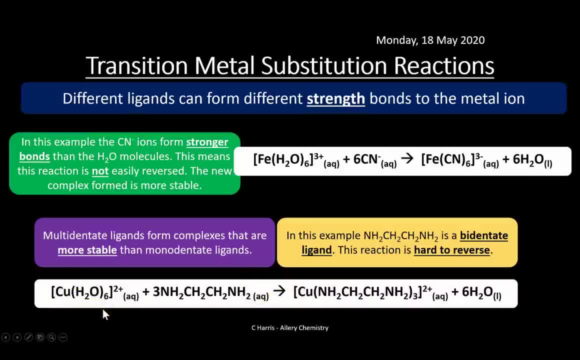 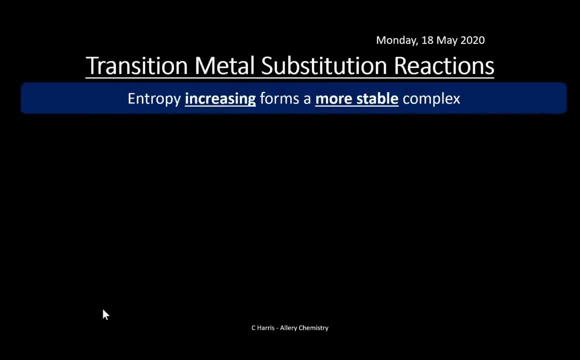 this reaction is very unlikely to go back to where it was before. okay, and so, still, looking at these substitution reactions, we're now going to bring in entropy. okay, now you, depending on, again, depending on the order that you've um looked at these, uh, entropy is a, is a is an interesting topic because 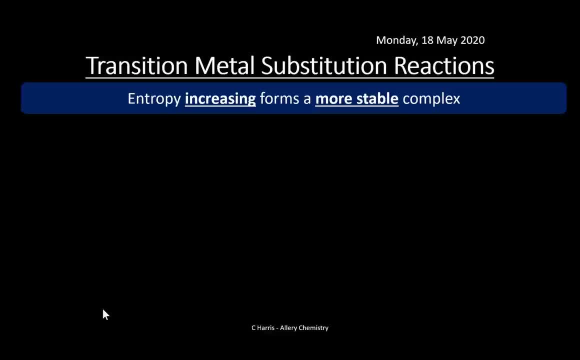 it's, it's the measure of you um order and disorder in reactions, so we can also apply it to um transition metal, substitution reactions and basically increase in entropy is forms a more stable complex. so here we're looking at the number of ways in which an atom or molecules can be arranged so in a ligand exchange reaction. 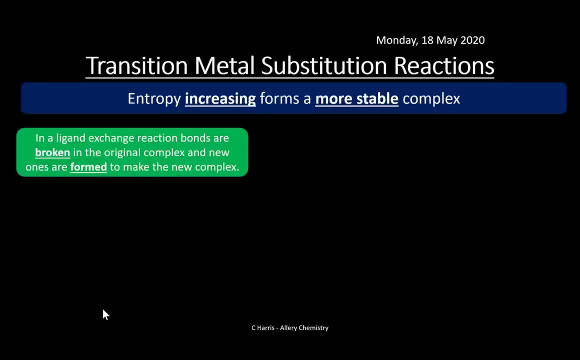 bonds are broken in the original complex, which is fair enough. we break the bonds and new ones are formed to make the new complex. so quite often the energy needed to break the bonds as similar as the energy released when the new ones are formed, so the entropy change is likely to be small. so in other words, if we're breaking the 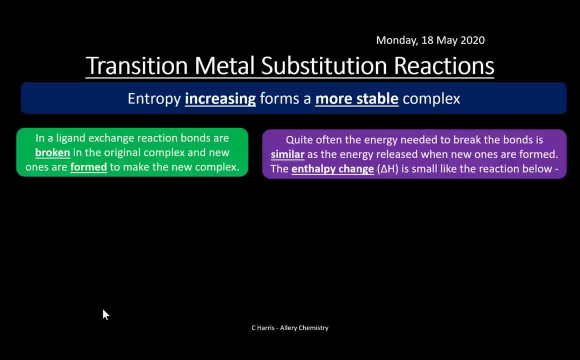 bonds between the metal ions and the ligands. the bonds that are formed in the new complex are roughly about the same, so the entropy change is is negligible. basically it doesn't have much of an impact, but nonetheless we can still get very decisive reactions here. so if we bring back that, 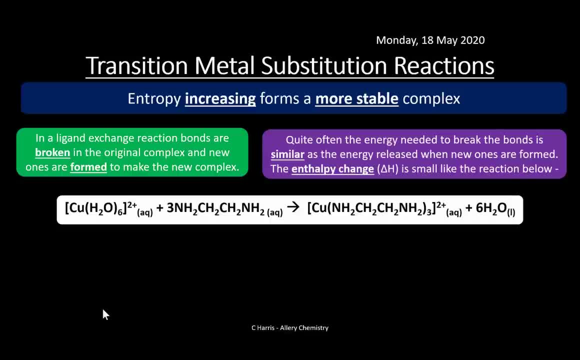 copper, hydrated copper complex. there's the hexa aqua complex. we're acting it with a bidentate ligand here. okay, so this is ethan. ethan is a bidentate ligand here and we're breaking the bonds in one, two diamines, your bidentate ligand. this forms this complex here and six water ligands now. 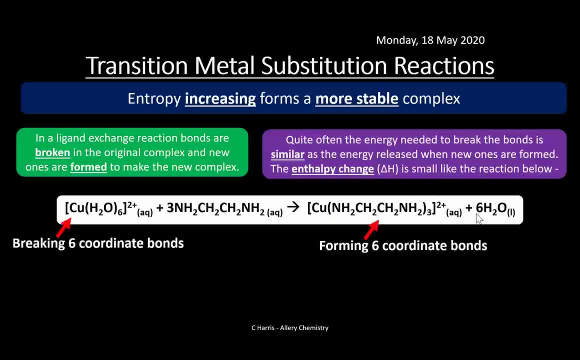 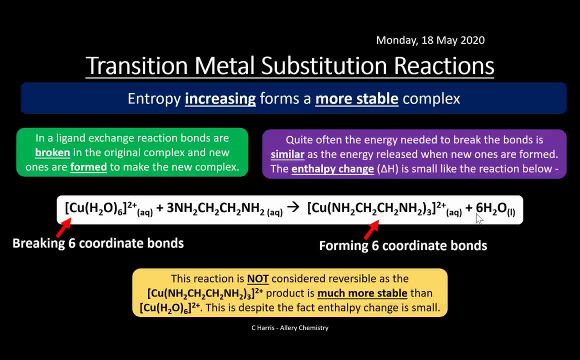 simply, all we have to do is, if we break six bonds here, we're going to form six bonds there. so the amount of end, the entropy change, is very small. but this is not considered reversible. okay, because the product this year is a lot more stable than that, despite the fact that the entropy change is. 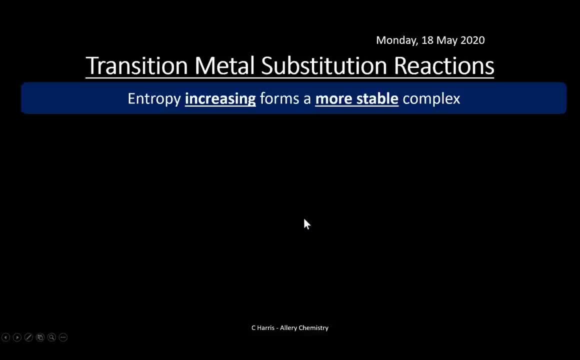 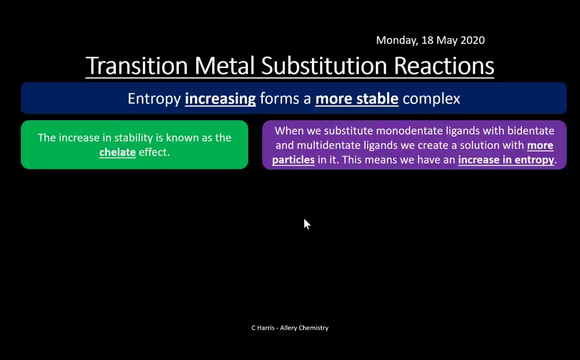 small. there's something else at play here which is obviously, which is obviously entropy. so entropy is actually led to something, a phenomenon called the chelate effect, and so the chelate effect is responsible for the stability of a complex. so when we substitute the monodentate ligands- remember that previous example- we had six water ligands around. 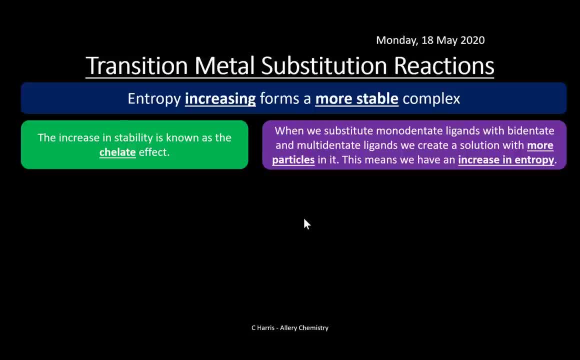 there and replacing it with our ethane one two diamine bidentate ligand. so replaced it with them. we then have a number of particles here, and so what we do is we create a solution with more particles in it, and this means you have an increase in entropy. so remember, if you've got more moles on the 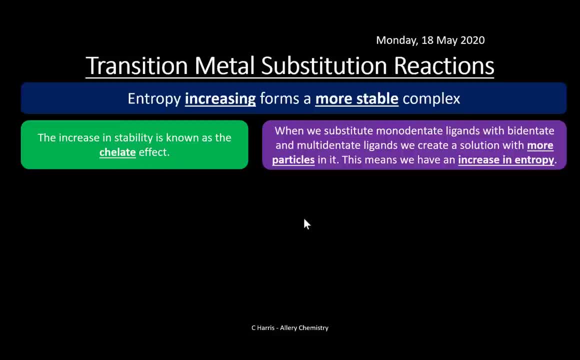 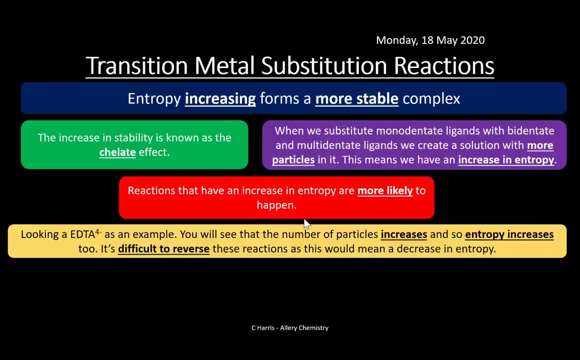 on the product side, then you have on the reactant side, then entropically that's a favorable process. so you can see reactions that have an increase in entropy are actually more likely to happen. so if we look at another example of a ligand- let's say EDTA, and then you'll see that the number of 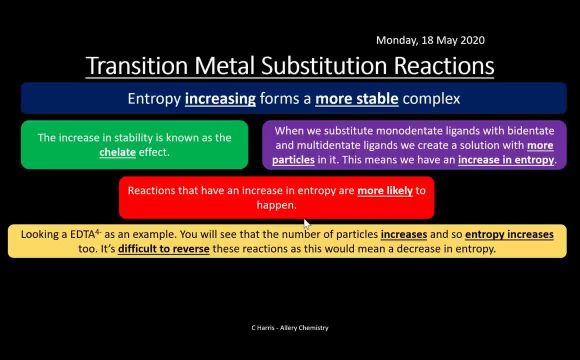 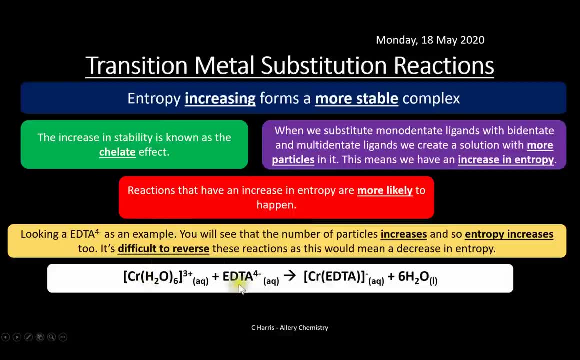 particles increases and so the entropy increases. so it's really difficult to reverse the force of a ligand, these types of reactions. so you can see, here we've got our chromium hexa aqua complex here, reacting it with our massive edta ligand here, so this is bond six times. it literally kicks all of. 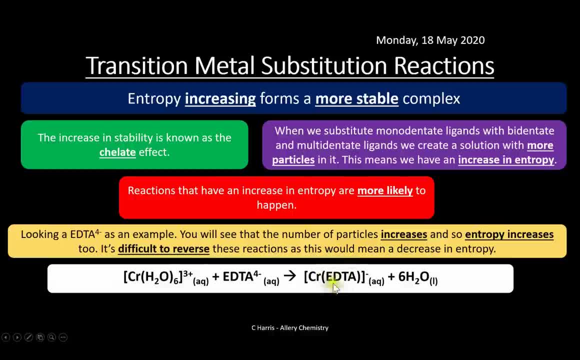 the six water ligands off the chromium and literally plonks itself firmly attached to the chromium atom here, so bonded six times, and the six water ligands are then left to float around on their own. so you can see here that we're going from two particles on the left to seven particles. 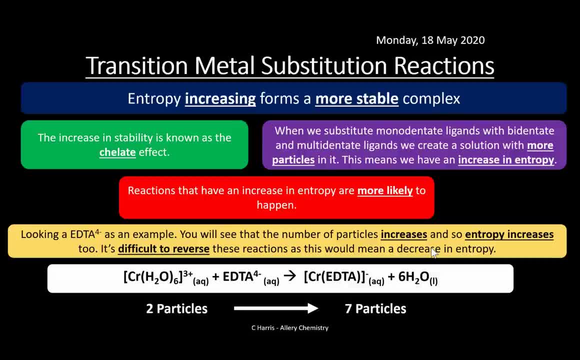 on the right hand side. so because we've got an increase in the number of particles, we have an increase in entropy. this is an entropically favorable process, going from two to seven particles. um, so that's what we're looking for as well. so make sure, if in the exam they're asking 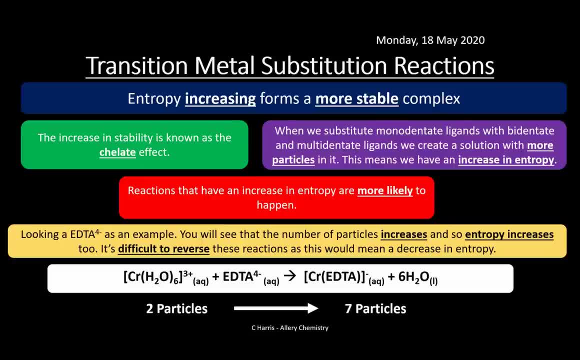 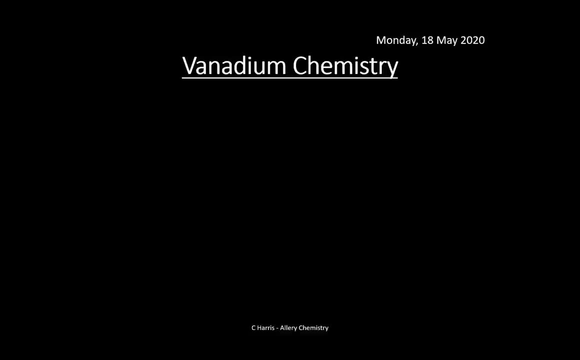 you to comment on things like entropy, um and the, obviously, the formation of your complexes there, that you um, you know, with your, your larger complexes, complex, your larger ligands bonding to the metal ion, then you're talking about entropy. okay, so, like i said before, we're now going to look at um, vanadium chemistry. so remember, i said 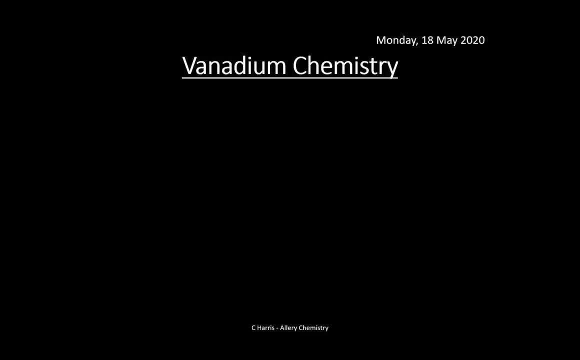 that you need to know a little bit more about vanadium chemistry. well, this is the bit that you're going to have to try and remember. there's a lot of reactions here and a lot of colors. um, you just need to try and remember them as best as you, as best as you can really. 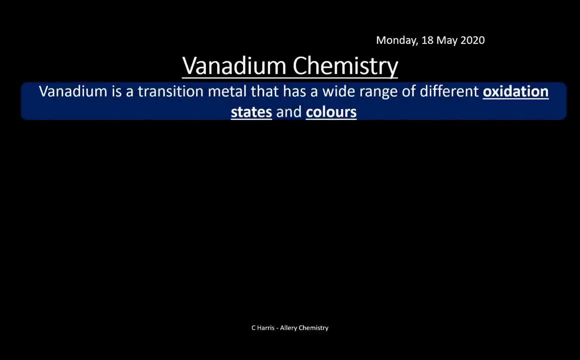 with anything like this. it's about practice and you'll just you'll become familiar with the colors over time. but vanadium is a transition metal, has a wide range- remember we'd seen it right at the start of the video where we'd seen that has a wide range of different oxidation, oxidation states. 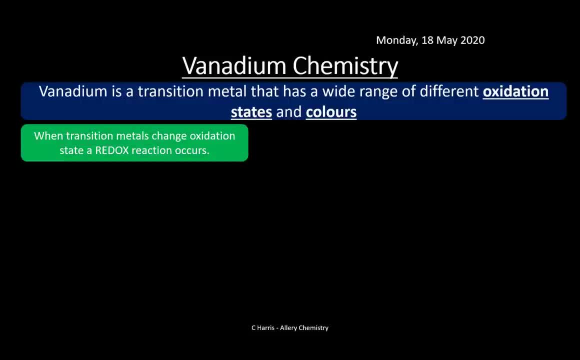 and there's a wide range of different colors we'd seen. so when transition metals change, oxidation state- okay, a redox reaction has actually happened. so we're getting reduction and we're getting oxidation, and this is what we're going to be looking at here. so we're looking at the change. 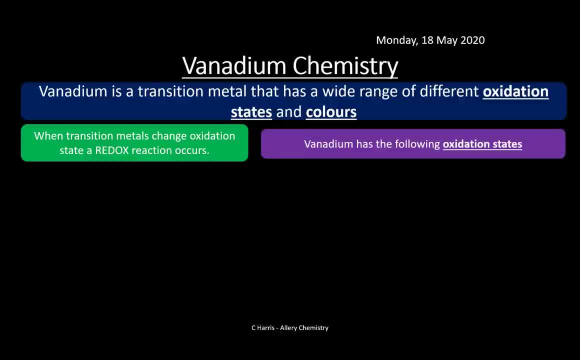 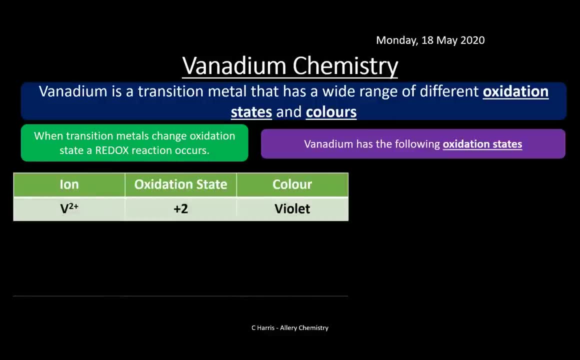 in oxidation state of vanadium and looking at their different colors. so it has the following oxidation states. so it has v2 plus, which has a plus two charge and is violet, and you need to know these colors. v3 plus is green, vo2 plus is blue and that has an oxidation state of. 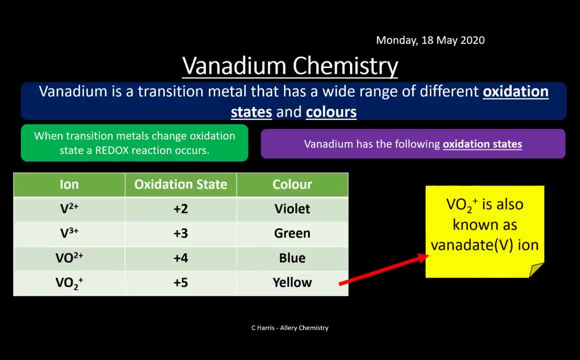 plus four. and finally, vo2 plus has a color of yellow and has an oxidation state of plus five. so you can see, here we've got different variants of vanadium, each having a different oxidation state. so make sure you're also aware that vo2 plus is also known as a vanadate five iron, so just 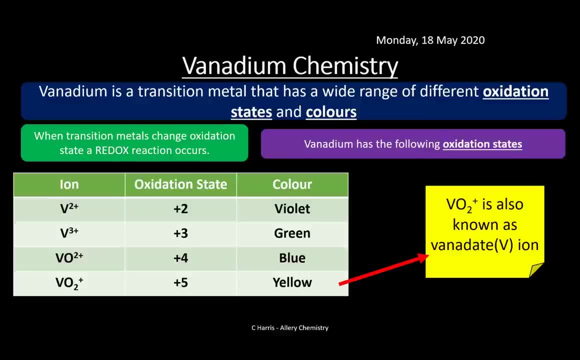 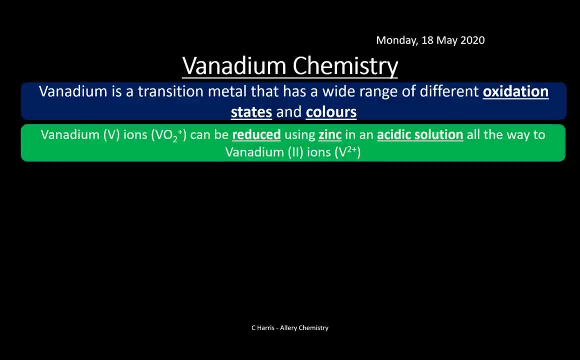 to. just as long as you're aware of that, you might see it's written somewhere. okay, so vanadium, vanadium, ions, vanadium, five ions, that's vo2 plus. these can be reduced using zinc in acidic solution all the way down to v2 plus ions. okay, you might have done this. 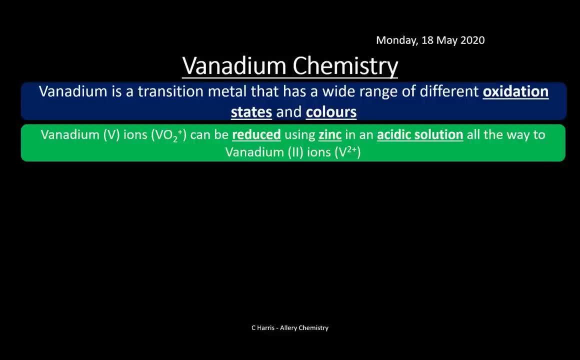 in chemistry, as in your at school or in at college, you might have actually done this reaction. it's a very straightforward reaction and basically you just put a chunk of zinc, and literally your chunks of zinc, into a, say, a conical flask and you swirl it with acidic solution and you actually get color changes. this is why i 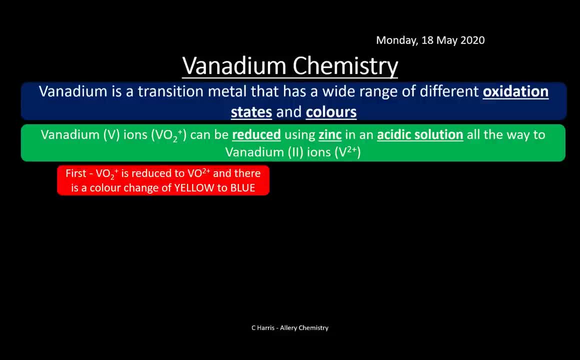 love inorganic chemistry. you get literally color change by adding a chunk of metal in there. so, first of all, the vo2 plus. we're going to look at these reactions here and you need to be aware of these reactions. it is a specific requirement from from aqa that you need to know. vanadium chemistry: 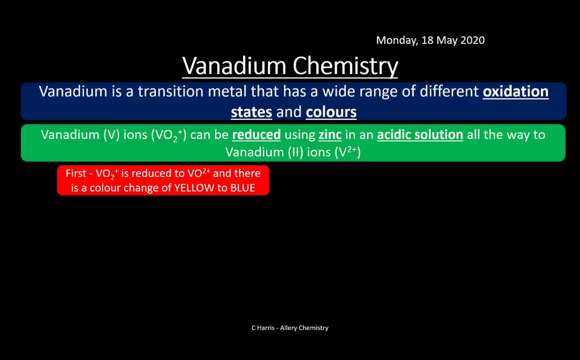 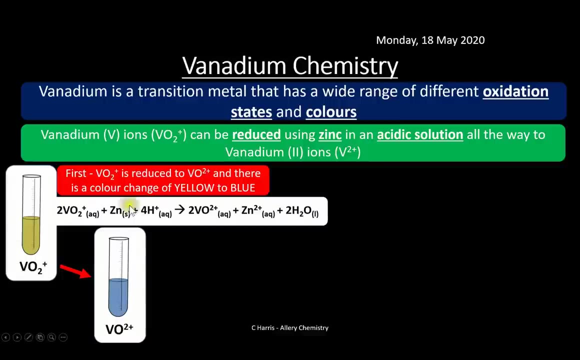 okay, so do pay attention to this bit. so, first of all, your vanadium, so your um, your vanadate ions here. so vo2 plus is reduced to vo2 plus. okay, um, and there is a color change. i've gone from yellow to blue. so let's have a look at the reactions here so you can see here that we are have our vo2 plus. 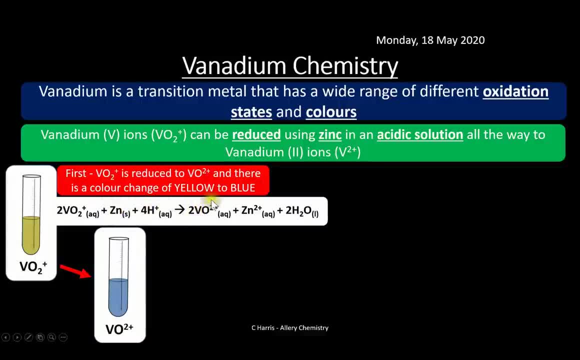 reacting it with zinc, and we've got acid in there as well, and this obviously reduces it to vo2 plus here, plus the zinc, two plus the zinc has been oxidized here, um, and then obviously water as well, and so we're going from the color change. obviously we're going from um, this yellow color, as you can see. 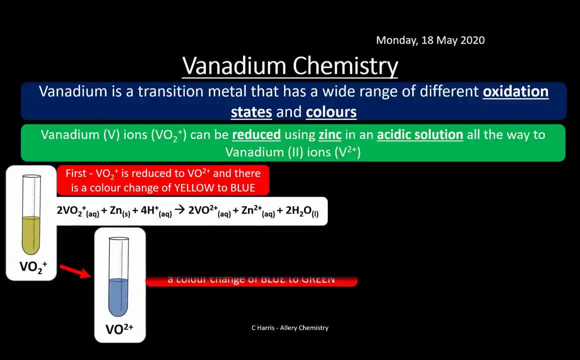 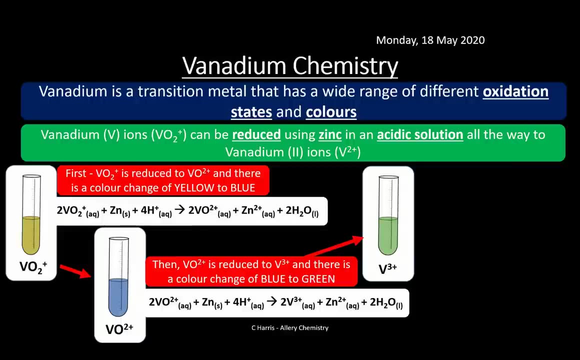 there. there it is and we're going to this blue color. okay, so this can then be um reduced further to v3 plus and there is a color change of blue to green. so you can see, there's the reaction there, the overall reaction. again, we're still using zinc to reduce it um and then finally this v3 plus. 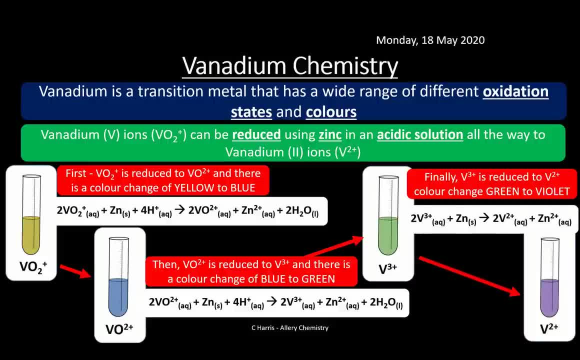 color change from green to violet. so there it is there, okay, and obviously that gets us our, our final product. so really really important that you need to know what's happening, so how it can be reduced, what you can use to reduce it and, obviously, the equations you can build them up. 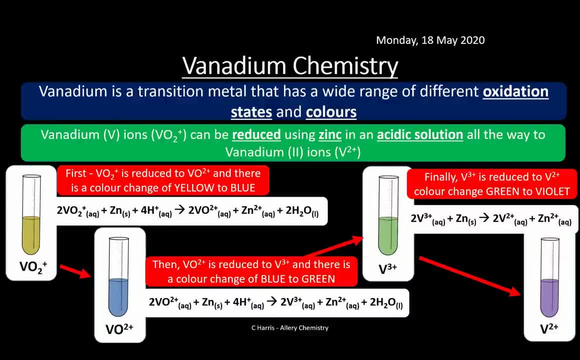 yourself. but you do need to be aware that zinc is used um to reduce um, your um, vanadium from- uh you know, from its vo2 plus to all the way down to v2 plus okay. so just be aware of that. it is a specific requirement. like i say that you do need to know about vanadium chemistry. 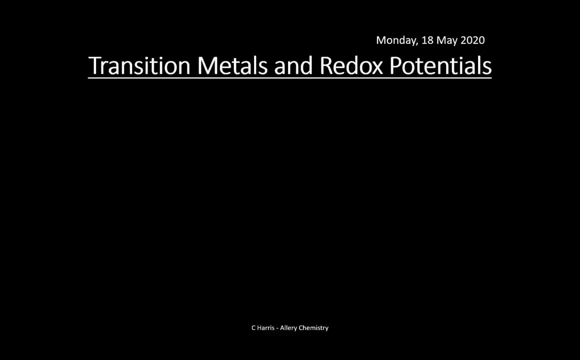 okay, so you might have seen this as well already: redox potentials. so if you've seen um and you've looked at the um topic of redox potentials, then this will be familiar with you. what i recommend. i would recommend that you do watch that video first if you've never heard of a redox potential. 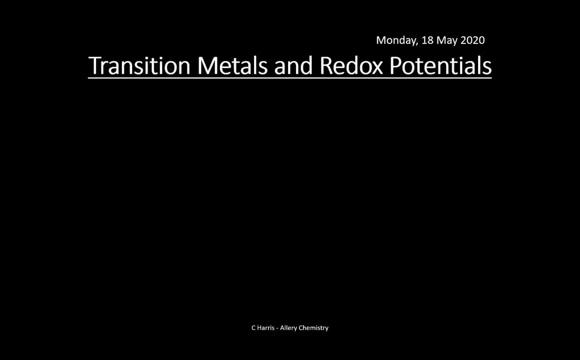 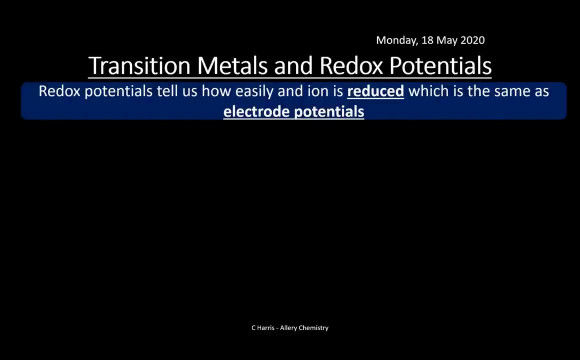 before, um, it's probably better you look at that video first, um, rather than or look at that topic first, rather than trying to work out what's going on here, because it does help if you know what redox potentials are and how they work when you're understanding this bit. so redox potentials, they basically tell. 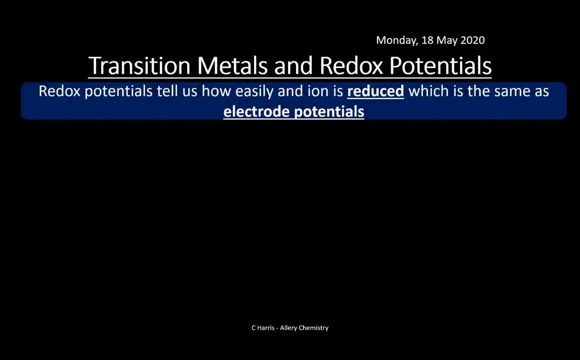 us how easily an ion is reduced, which is the same as electrode potentials. okay, so we're looking at redox potentials here. so the least stable ions- okay, have the largest redox potential and are more likely to be reduced. okay, so i'm going to say that again. so the least stable ions. 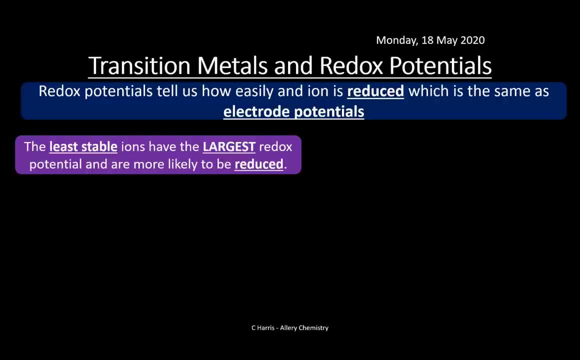 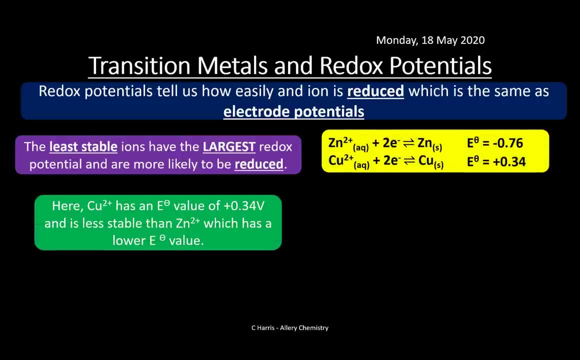 have the largest redox potential and are more likely to be reduced. okay, so let's have a look here. so we've got zinc and copper. so we've got these two different um, these two different um ions here. obviously, zinc isn't a transition element, but copper is, so we've got our electrode. 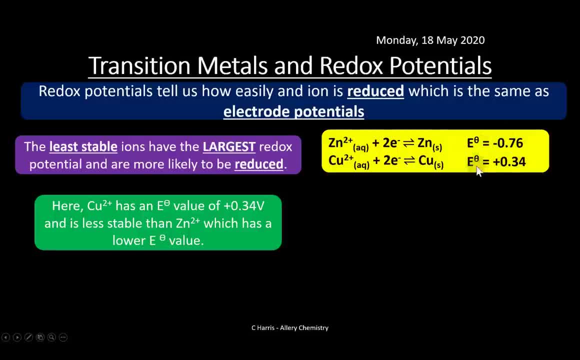 potentials here, so our redox potential, sorry, which are e naught. so here's our a naught value. so these are the same. basically, redox potentials are the same as your electrode potentials. okay, so you can see that the two plus this one here has an e naught value of plus naught point three, four volts, and 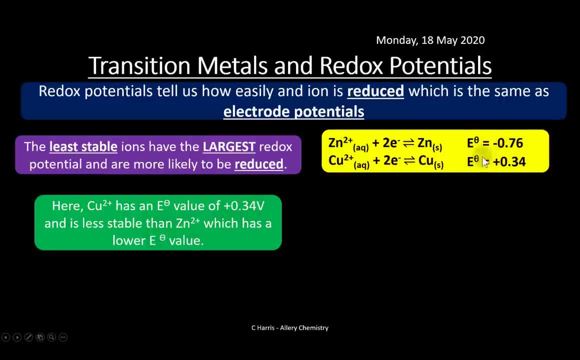 is less stable than zinc, which has a lower value. so this is less stable than that because, remember, the least stables of the largest redox potential. that's the largest redox potential, so that is the least stable. okay, so that one's more likely to be reduced. in other words, these reactions here are. 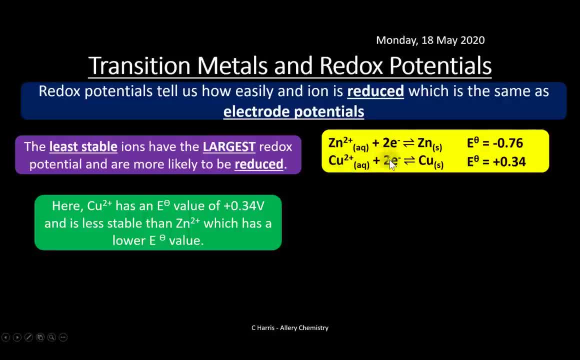 written in the reduced form already, because it's that plus electron. so remember, redox is oil rig, so oxidation is loss of electrons, reduction is the gain. so this is showing the reduced form. okay, so this one is more likely to happen. okay, it's more feasible. so remember all. 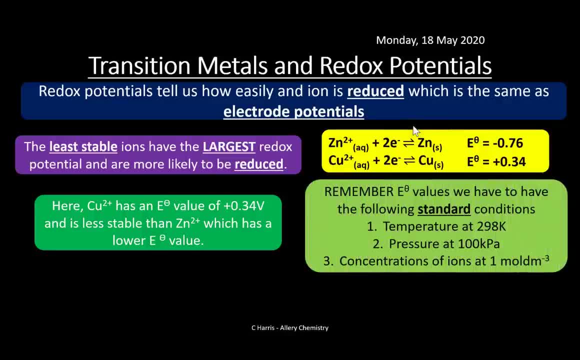 of these are done under standard conditions. so we have a standard temperature of 29298 kelvin, we've got a pressure of 100 kilopascals and concentration of ions are all at one mole per dm cubed. okay, so you can see. obviously there may be a difference in redox potential to the standard. 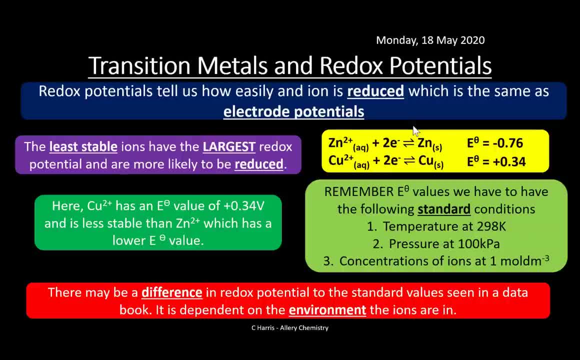 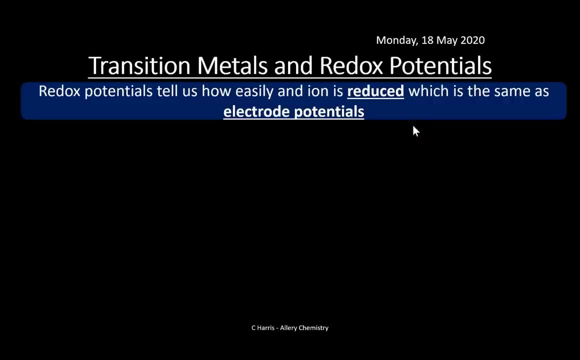 book, because the environment may be different. so we've got to ensure, when we're doing reactions like this, that we try and stick as close as we can to these standard conditions. otherwise the result you get is going to be very different to what you'd see in a in a data book. okay, so let's have 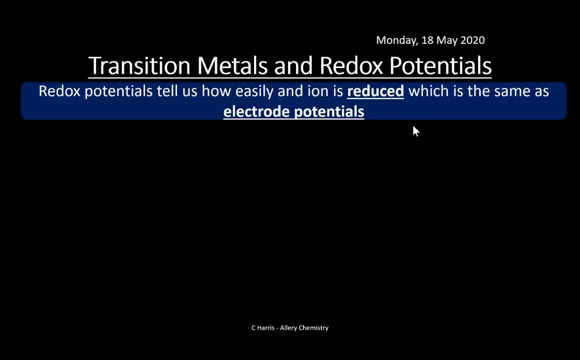 a look at, obviously, the redox potentials. we've looked at that there, so we're going to go through some different examples here, so let's have a look at ligands first. okay, so ligands- the standard potentials are always measured in aqueous solutions. very, very important, okay, always. 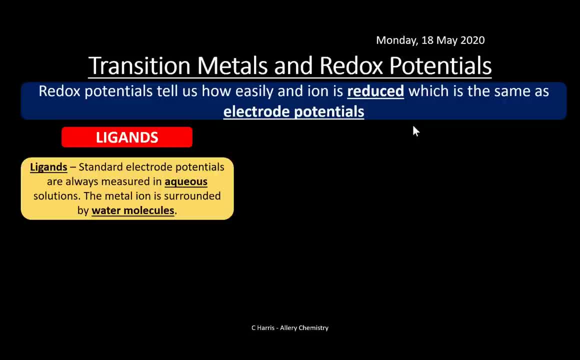 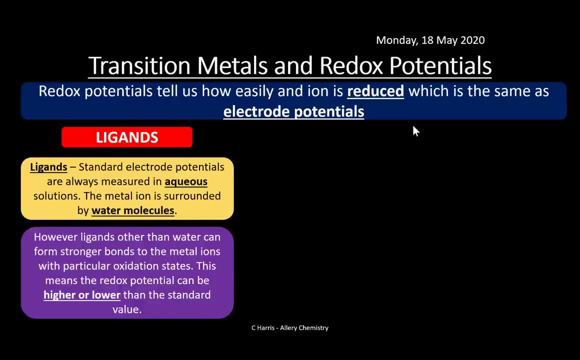 measured in aqueous solution and the metal ion is surrounded by water molecules when we're looking at this. okay, so the ligands do play a role in here, however, ligands other than water. these can form stronger bonds to the metal ions with particular oxidation states. so we'd seen that already. 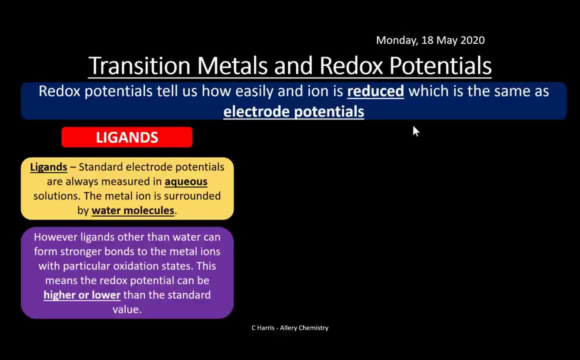 remember, such as carbon monoxide and cyanide, for example. so some of them can form stronger bonds here or lower than the standard value, because the ligand may be different. so the might ask you about what could alter. why do you have a difference in actual value against practical value? okay, so 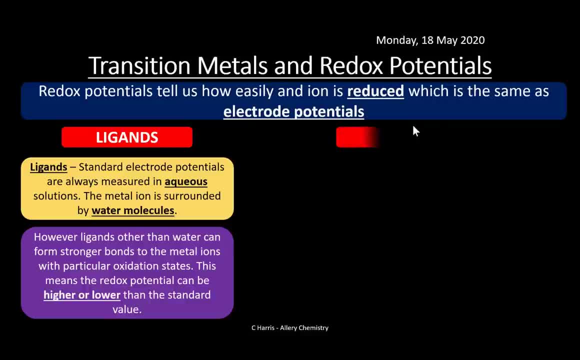 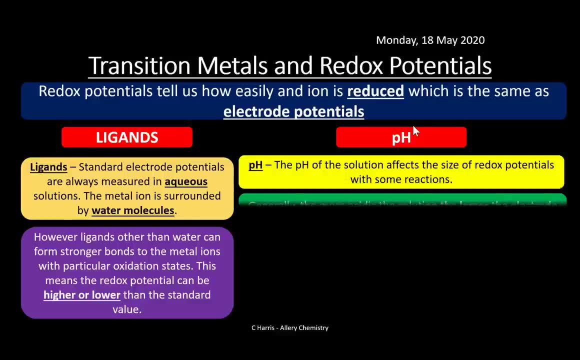 theoretical value, should I say? this could be said, and this could be one of them- which is ligand type. ph is another one, and so the ph of the solution affects the size of the redox potential as well with some of these reactions. so generally, the more acidic the solution, the larger the electrode. potential. but especially there is no octane island, being a ferrous atom, so you see kind of an geometrically different temperature and fit between polar shark structure or other anywhere in the building. my spot here, byikesYA, bright from the References in a history of берkshire University, was picked up from a 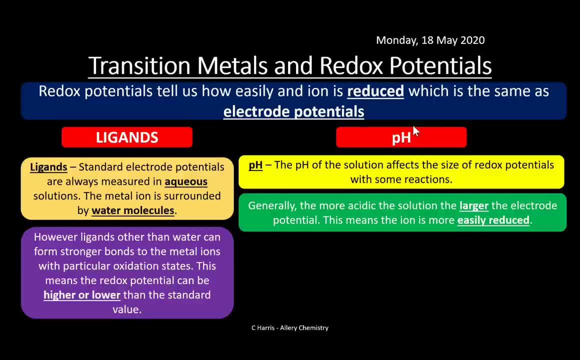 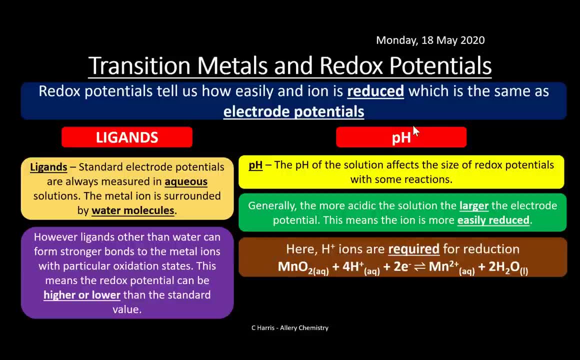 and so therefore, this means the iron is much more easily reduced. okay, so very important. so the more acidic solution, the larger electrical potential. so, for example, here h plus ions are required for reduction. so you can see it there, okay, so, um, so you need h plus ions. are here that basically? 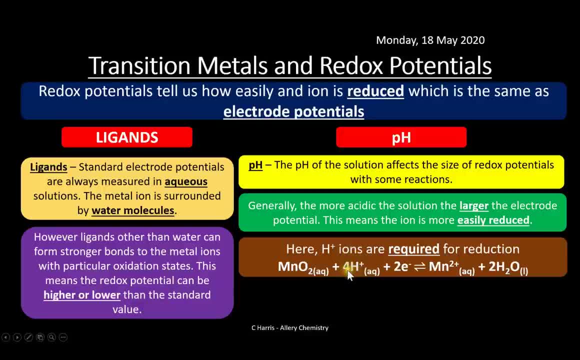 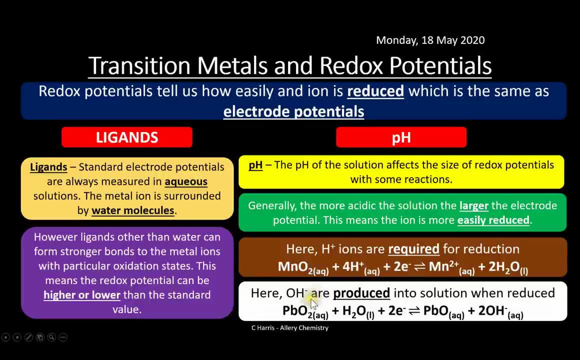 means that we're lowering the ph, we're adding an acid. so this is required to allow this reaction to actually proceed, to allow it to go. and so here, um, you can see, hydroxide ions here are produced, um into solution when they're actually and when they're actually reduced. so you can see here that 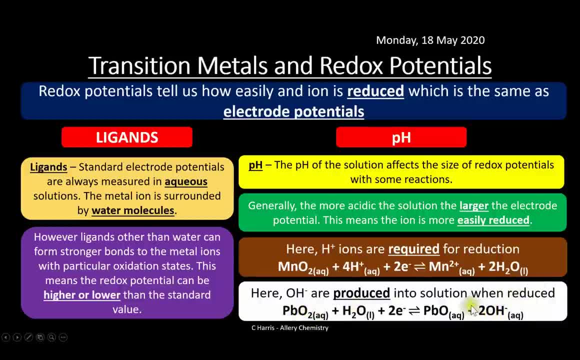 we're actually making uh hydroxide ions here, um, and this allows it obviously to go back to lead oxide as well. so this is obviously increasing the ph. so you need to be aware of um. what affects the actual um. you know, redox potentials, um, which are the same. 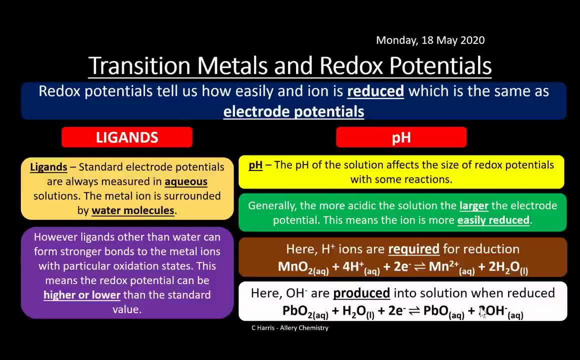 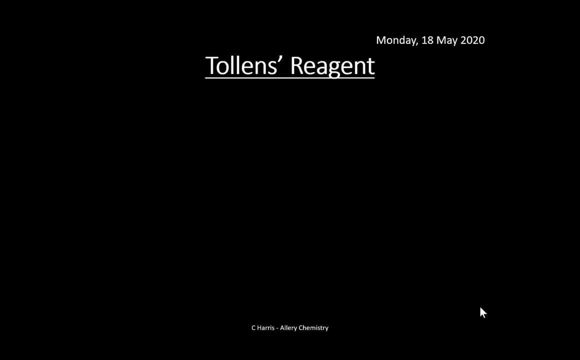 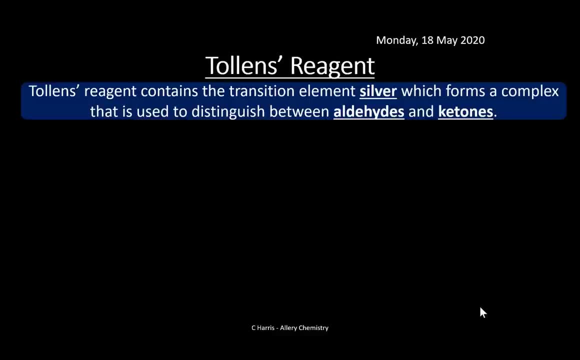 electrical potential. so we need to know the impact of that. so, for example, ligands, and obviously the ph is bomb, okay. so we're going to look at um tollens reagent. we've seen a little bit of that already because that was an example of a linear complex. so tollens reagent, remember is is used. 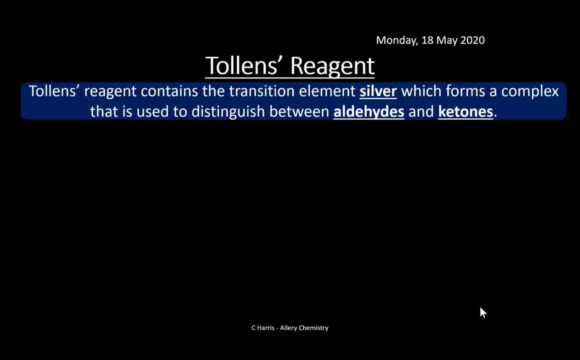 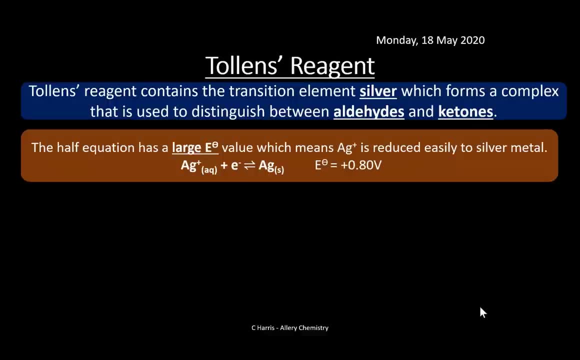 to distinguish between aldehydes and ketones, and it's also known as the and the silver mirror test. it's a really good, good test. so so we've seen that already, and now the half equation for this equation is the silver mirror test. so we've seen that already. um, now the half equation for this. 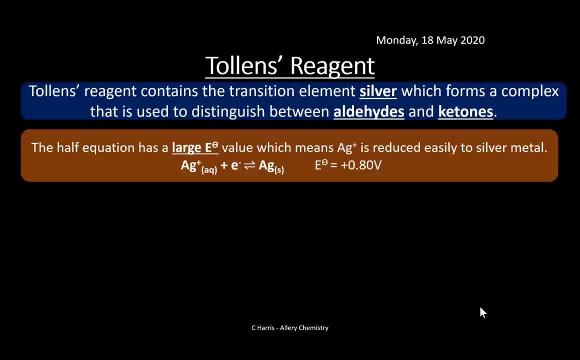 type of reaction has a very large uh redox potential, or electrode potential, okay, which means that the silver plus ion is reduced easily to silver metal. so remember, if it has a positive value, that means that this reaction is likely to proceed. okay, this is a feasible reaction. so 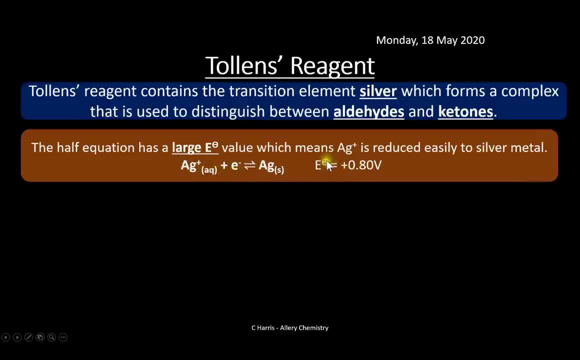 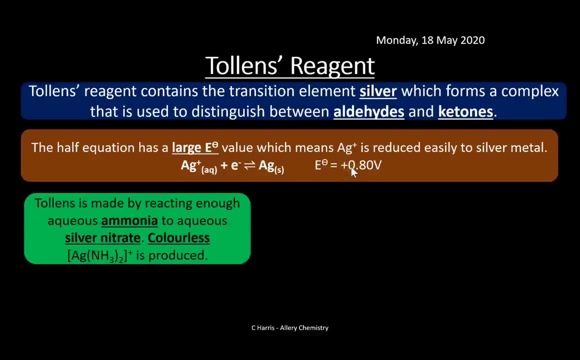 silver plus picking up that electron to form silver is is likely to proceed under standard conditions. okay, so the tollens is made by reacting enough aqueous ammonia to aqueous silver nitrate and we get this complex produced. so that's how we make the tollens reagent. 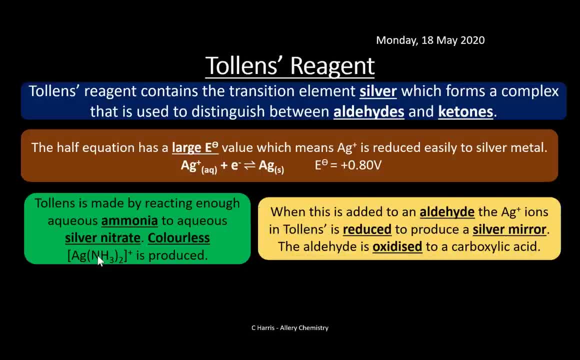 and when this is added to an aldehyde, the ag plus ions in the tollens are reduced to produce your silver precipitate here, which is obviously your, your silver mirror. so effectively your silver is being reduced because it's gone from plus one oxidation state to to zero, but it will. 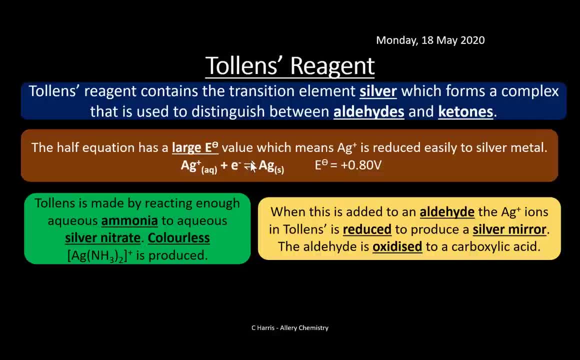 only do this if the substance it's reacting with can be oxidized, and aldehydes can be oxidized and but ketones can't be remembered. so if you add tollens reagent of ketone and there is no reaction because ketones can't be oxidized or anything, so therefore obviously your tolerance reagent will. 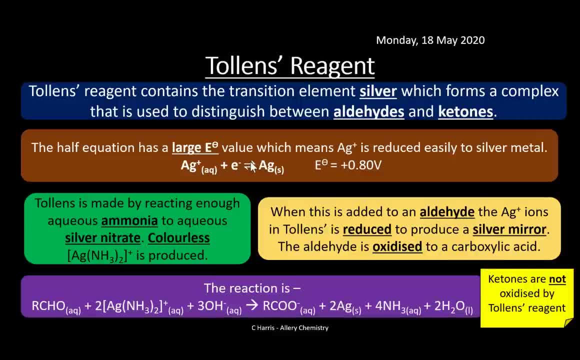 not be reduced. so the overall reaction here, um so, remember, your ketones are not oxidized, but your overall reaction is this: so you've got your aldehyde here, reactant with your tolerance, reagents dissolved in in a an alkaline solution. so we've got some ammonia, we've got an alkaline solution. here, um, and obviously then we forward the alky stressed one. you get an alkaline solution here, um, and obviously thencause the ammelium helps to be oxidized, so after a while we react. so that's actually the actin secures the collagen and um, but we're hearing the oxidation. 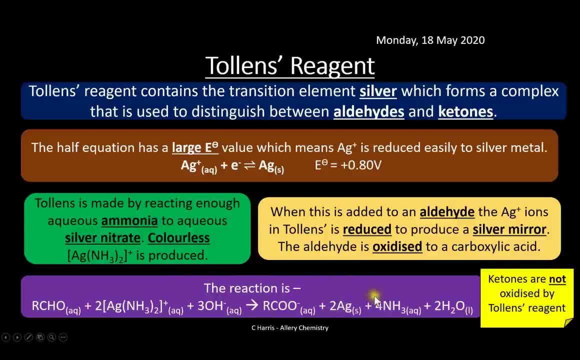 here, and obviously then we form our silver mirror here. ammonia is also produced in water, so you need to just be aware of the reactions, of why this is feasible. obviously we can see it, we know it works, but we need to just demonstrate it using these redox potentials here. okay, right, so what? 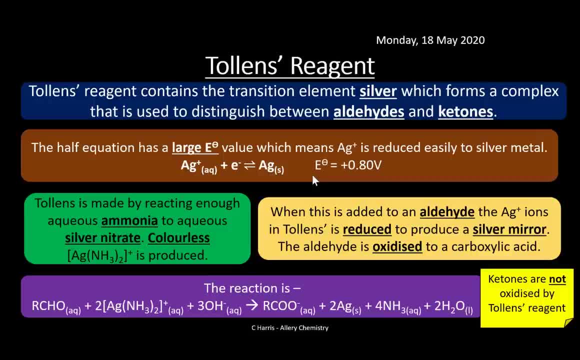 we're now going to look at our titrations, because it wouldn't be- it wouldn't be transition metals without looking at a titration. so these are slightly different titrations. the titrations you would have seen are acid-base titrations, so that's your standard one, but you can also get. 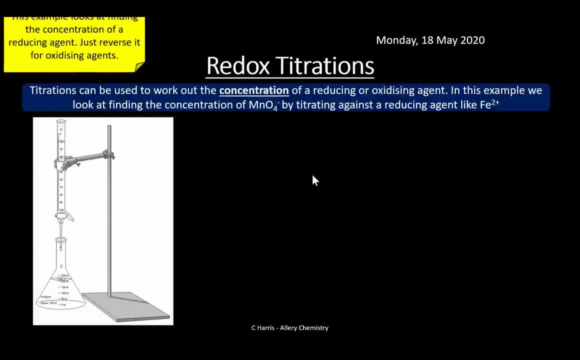 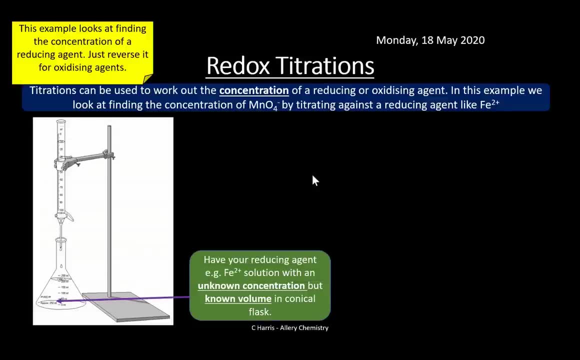 redox titrations as well. now, redox titrations are basically used to find the concentration of a reducing or oxidizing agent. so instead of trying to find the concentration of an acid or a base- so in this example we're going to look at trying to find the concentration of manganate ions, which 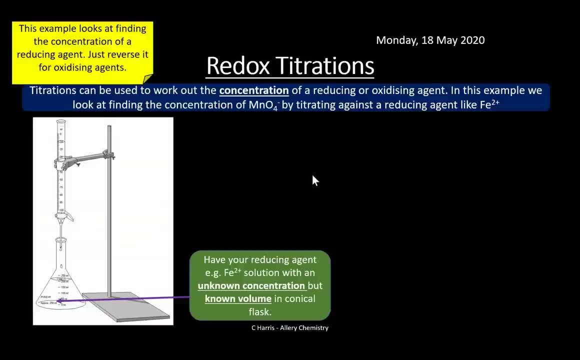 is mno4 minus. remember, it's that purpley color, nice, deep purple color, and we're going to try to titrate that against a reducing agent like fe2 plus. so fe2 plus, remember, is a green, like a pale green color. okay, so what we're going to look at is this: 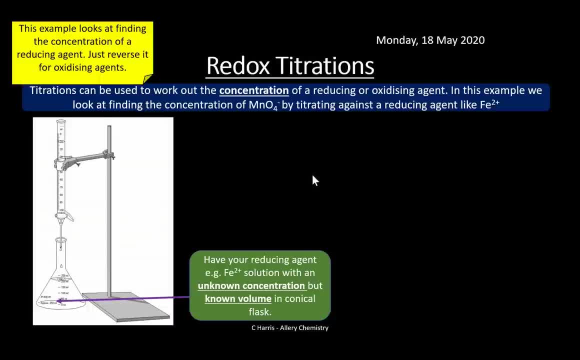 is just finding out the concentration of a reducing agent. all we have to do is just reverse it to find out what it is for oxidizing agents. okay, so it's pretty much the same. so our setup, our setup is pretty straightforward. we have our burette, as you can see on the top there, clamped into the 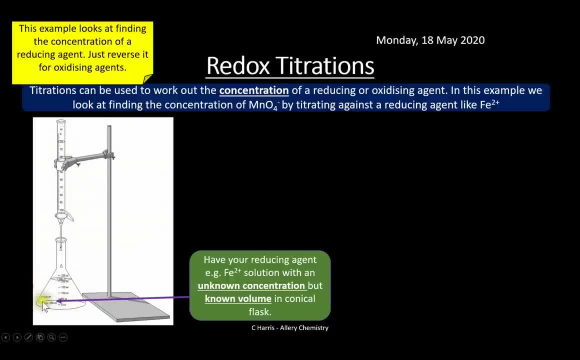 clamp stand, and then we have our conical flask and in here we have our redox titration and then here we're going to put our reducing agent in. so, for example, we're going to use fe2 plus. now we don't know the concentration of it, but we do know its volume. normally we measure this in 25 centimeters. 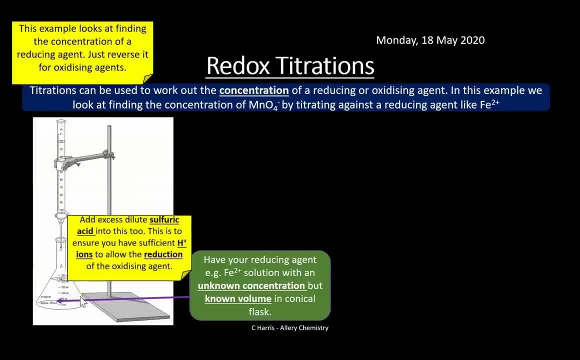 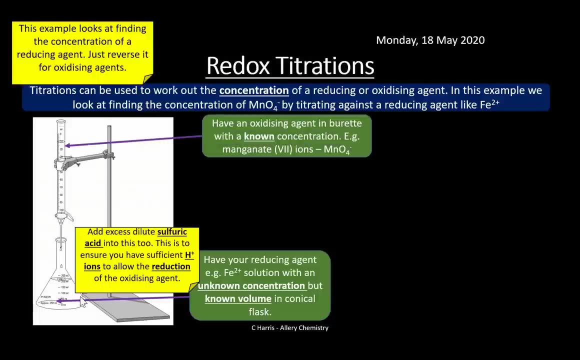 cubed, okay. so then what we need to do is add excess dilute sulfuric acid to this, and this is to ensure that we have enough hydrogen ions in there, so h plus ions, to allow this reduction process to occur. so we have our oxidizing agent in there, so we're going to put our reducing agent. 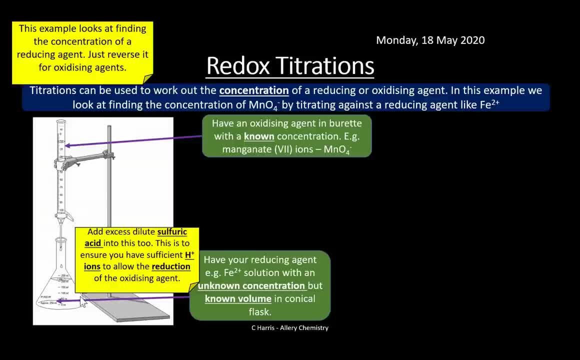 in the burette and this is known as. this has a known concentration. so we know the concentration of that which we don't know its volume. but we're going to add that to our ion 2 plus and to work out its volume. so this is obviously got the magnet ions in there, and then we add the magnet ions into. 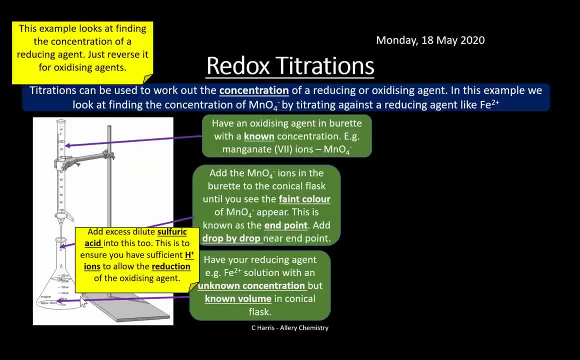 the burette into the conical flask until, we say, the faint color of manganate start to appear and this is known as the end point. so, unlike your acid-base titrations where we used an indicator to try and spot the end point, and because we're using colored compounds here, cuz. 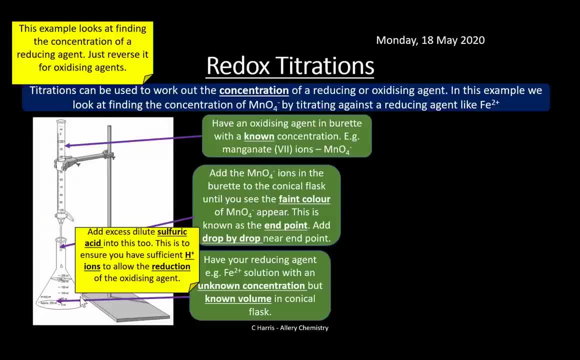 the transition metals. we don't need to add a, an indicator in here, and this will actually itself indicates effectively. we've got to remember to add it drop by drop near the end. okay, because one drop can make a big difference to the end point. okay, so we've got a really slow down when 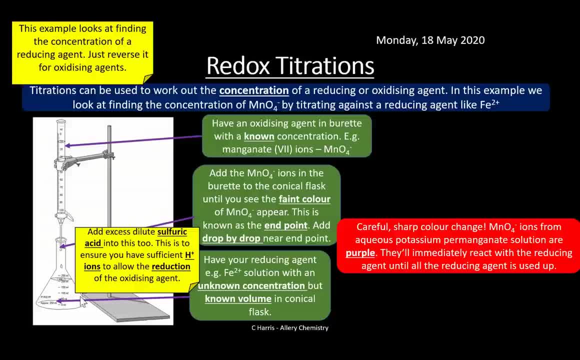 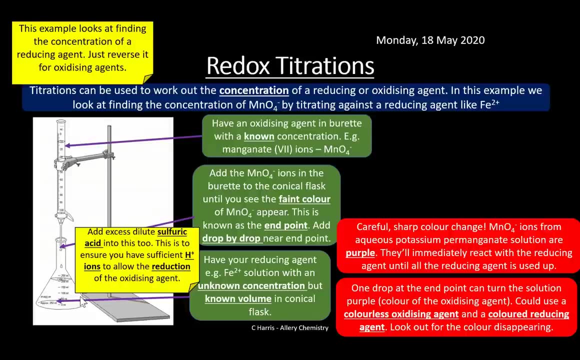 we get near the end point, so that sharp color change, we've got to be very, very careful and they'll immediately react with the reducing agent until all of its used up, and then it'll it'll go a deep purple color up straight away. okay, so, um, like say, one drop can can make a massive difference. 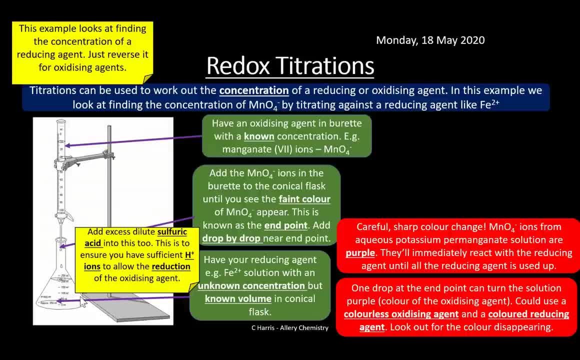 and we could use a colorless oxidizing agent as well and a colored reducing agent. all we're doing there is we're looking for the color to disappear. so in other words, we have our colored substance in the conical flask here and we have color solution in here and effectively we're adding that. 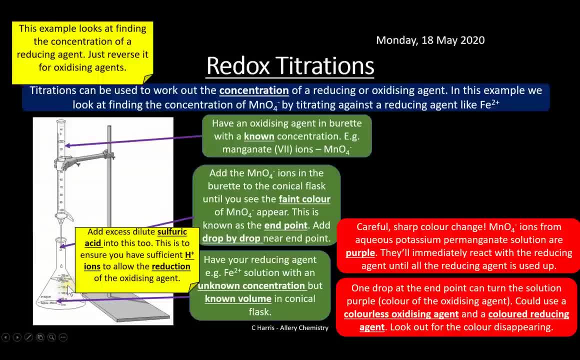 and we'll keep adding until that color disappears from there. just depends on what you're reacting it. so then, what we do: once we've added our chemical and we've reached the end point, then we need to read how much oxidizing agent was added. and remember, we all, we always read from the bottom. 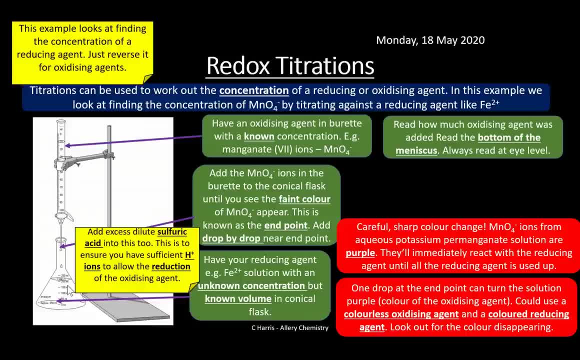 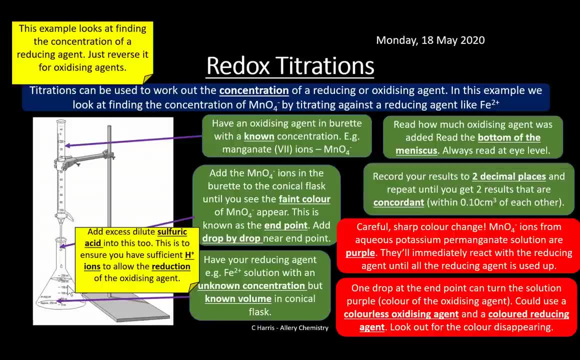 of the meniscus, that's the semicircular bubble, so it's always at the bottom of the semicircle. and then we obviously got to record our results, and we always record results to two decimal places and we repeat the results to. we get two concordant ones. so that must mean they've got to be between. 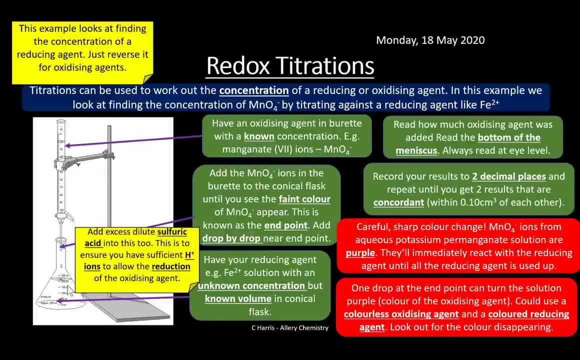 it's no point in having um running a titration and getting a result of 20, 22 and 25, because they're miles away. you know how do you know which one is going to be, you know the right value. so we've got to do it until we get at least two concordant results, in other words, within 0.10 centimeters. 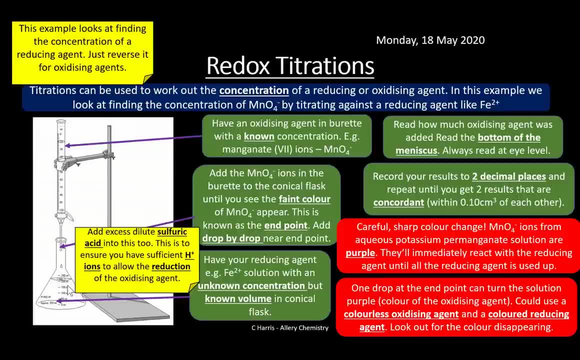 cubed. also, it's really important when you're writing down titration values, you must give it to two decimal places. even if it comes out as 20 it is, you know you've got to give it two decimal places. so that's going to be 20.00. 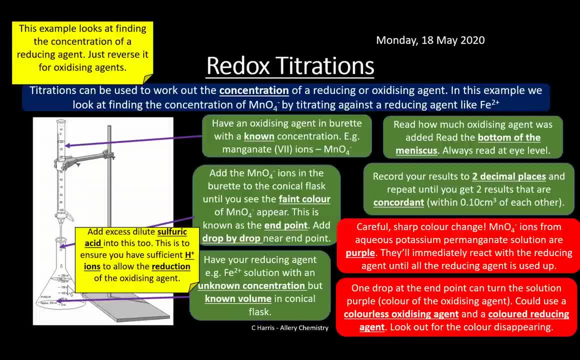 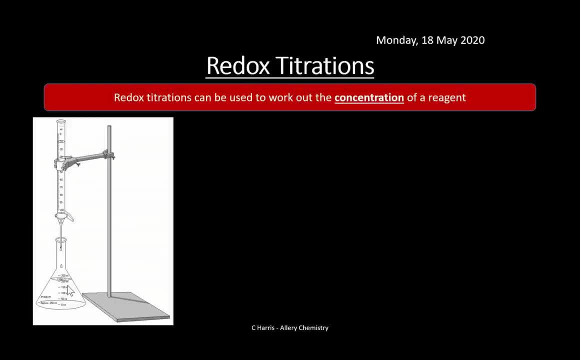 okay, really, really important. that is the standard way in which you record titration results. okay, so we're going to look at a calculation example here. so we're going to use redox titrations to work out the concentration of a reagent. so here we're going to use 18.3 centimeters cubed of 0.02- 50. 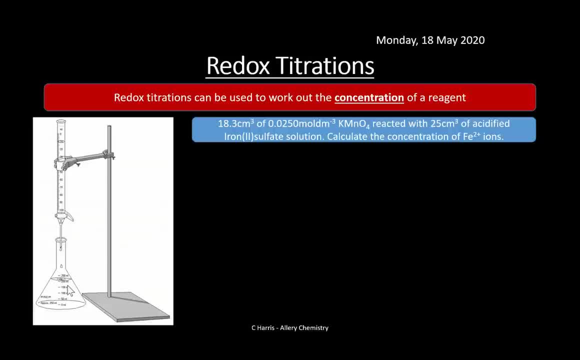 moles per decimetres cubed of potassium manganese and that's going to be reacted. we're reacting with 25 centimetres cubed of acidified iron, ответ cube it is & iito space an. we're going to calculate the concentration of i & i and so basically, just like what we mentioned before as the example, so we're. 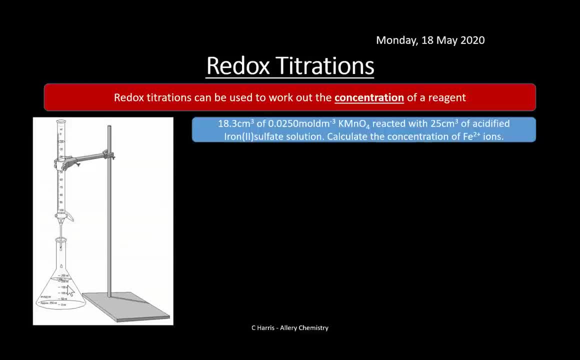 going to work through the calculation now, if you know, if you know my videos. you know i normally say, if in doubt, work out the morals. well, we are going to be working out the moles 9 minuteitty and first in this type of reaction. but before we do that, so we need to write down our equation. 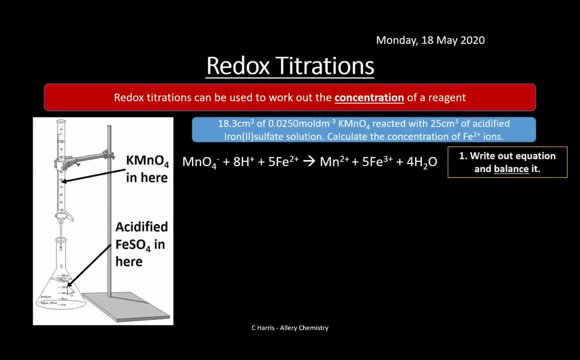 first 9 sol, inte 10 minutes. so our equation is this: okay, so balanced equation. so you're going to look at a database using this and you're going to write down on the equation first. here you can. this group is this, which is that it's the starting equation and that's going to be our answer to this powerful equation. so you're. 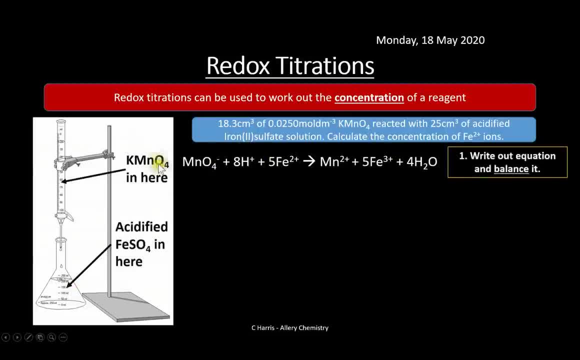 you've got manganate reacting with our iron two plus and this is our overall ionic equation. we have our potassium manganate, potassium permanganate in here in our burette and we have our acidified iron sulfate solution, which is going to produce the fe2 plus ions in the conical flask there at. 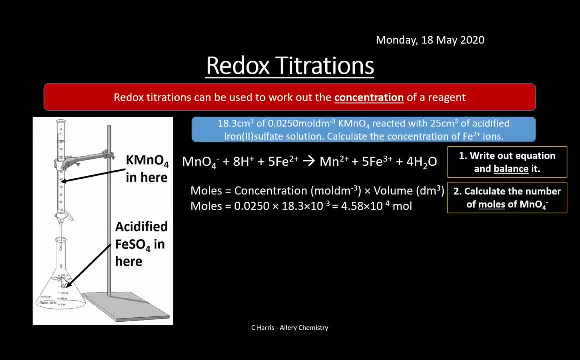 the bottom. so then we need to work out the number of moles, like i say. so the moles of manganate, dead easy moles, equals concentration times volume. so put the numbers in there and then, once we've worked- um, sorry, before before i move on, i'm jumping on too much um what i do and 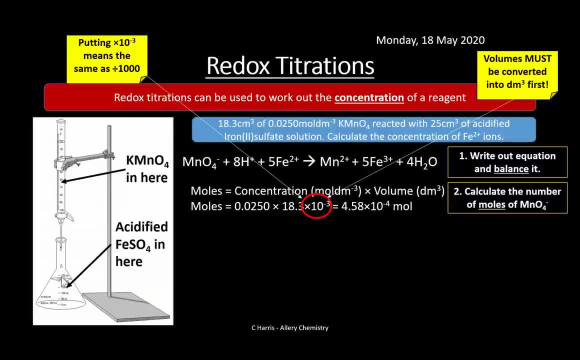 you may see this if you've seen previous videos um, where i normally put times 10 to the minus 3 at the end there, because, remember, 18.3 is in centimeters cubed. we want to get that into decimeters cubed, so we must convert it into decimeters cubed first and i just simply add: 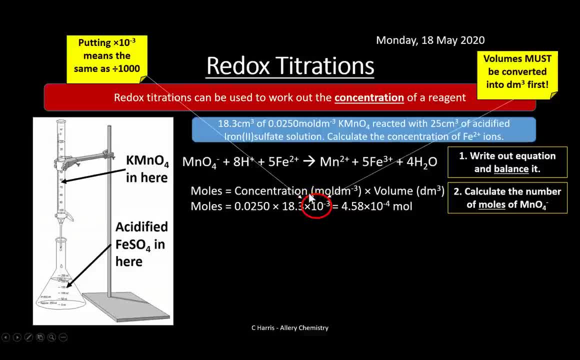 times 10 to the minus 3. on the end, it means the same as divided by a thousand. so if you're wondering where that's come from, uh, okay, so then. once we've done that, we then need to use the equation to work out the molar ratio in order. 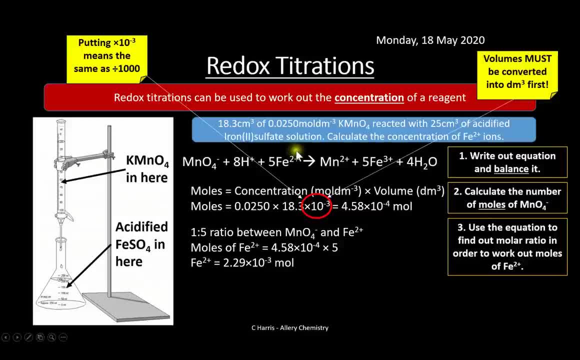 to work out the moles of fe2 plus. so you can see um that we have a one mole of mn04 minus to five moles of fe2 plus. so you can see, we do 4.58 times 10 to the minus 4, multiplied by 5 and we get the. 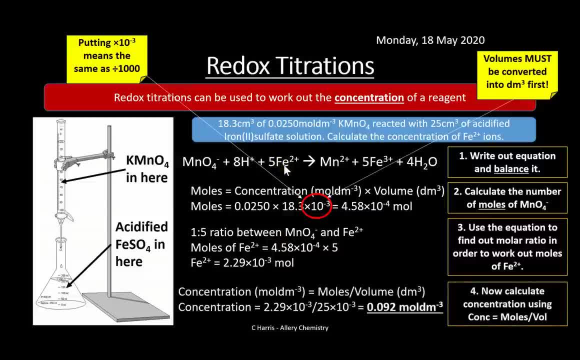 number of moles of iron. and then of course, once we've done that, we then calculate the concentration, because now we know the number of moles of iron in there and obviously that gets us 0.092 moles per decimeter cubed. so that's the number of moles of iron in there. and then, of course, once we've done, 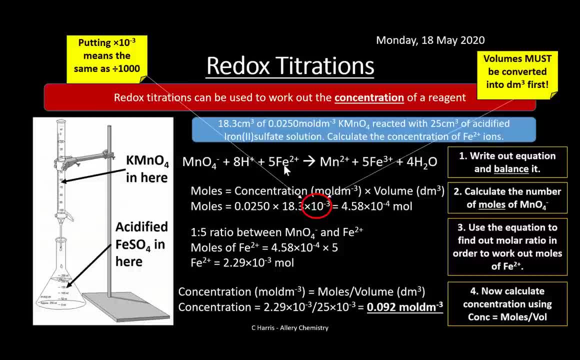 that we get the number of moles of iron in there and then, of course, once we've done that, we get the cubed. okay, so remember: concentration of moles divided by volume: make sure your volume is in decimeters cubed. that's the main thing. some people don't convert that and you're not going to get the. 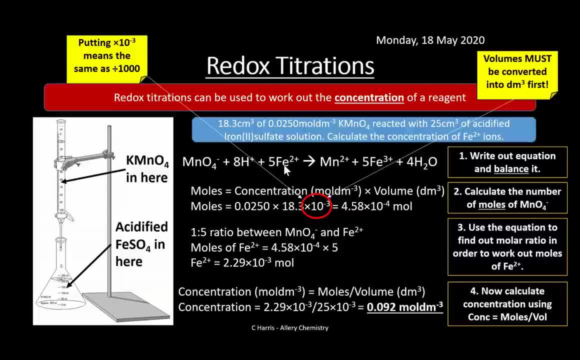 right answer. it's always going to be out by a factor of a thousand. okay, so obviously that they're all the titrations. it's very important that you need to be able to do titration calculations. i really can't emphasize that enough. you know you are going to get some form of calculation in your 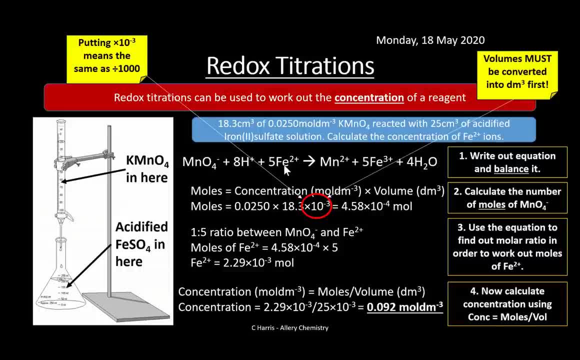 exam. it might not be a titration one. it might be other types of uh calculation relating to um- you know, redox, for example, and but you certainly will relating to say, like um, electrochemical series, for example, in this topic. but you know, titrations is fundamental in chemistry. you, you're 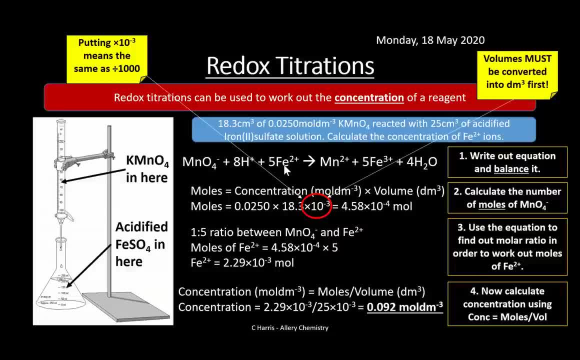 probably sick of seeing titrations, i would imagine. okay, so we're just going to move on to the final parts of this video, and the final parts is where we're going to look at, uh, catalysts. so remember one of the one of the features of a transition metal is they're good catalysts. so we're going to 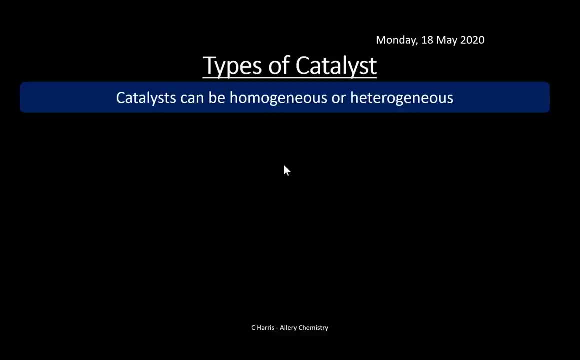 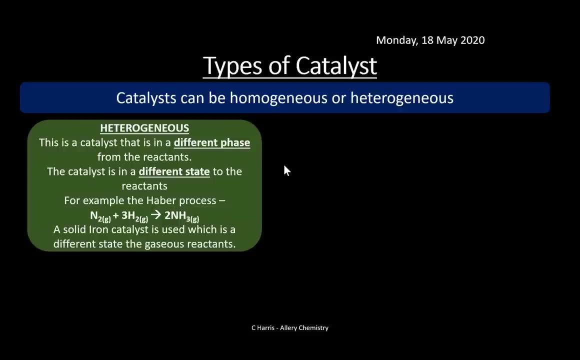 look at the different types of catalysts and they come in two types: which is homogeneous or heterogeneous? and we need to know both. so we're going to look at heterogeneous first. so this is just a catalyst that is in a different phase from its reactants. so, for example, the Haber process is 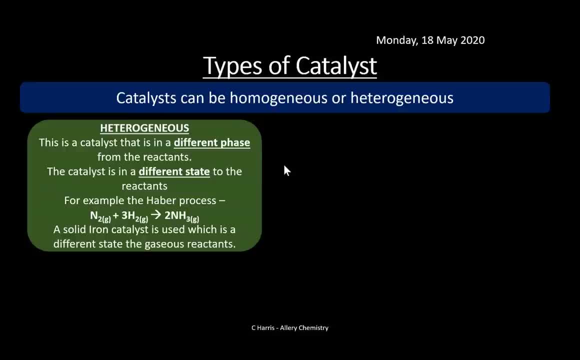 a classic example. so the Haber process is the manufacturer of ammonia and you can see there's our ammonia there, okay, so ammonia is used in fertilizer, so it's actually a really, really important reaction here. so this, these are all in gases, as you can see on there, they're all gases. 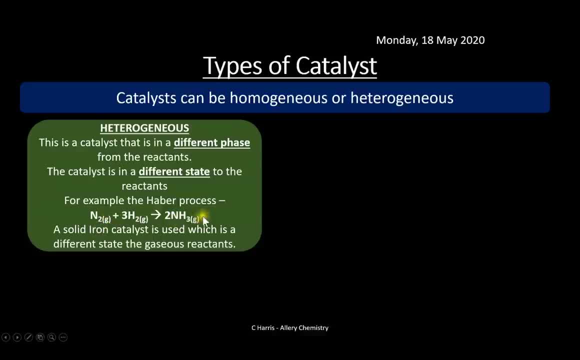 but we use a catalyst which is iron, so iron's in a different state to the gases here. so therefore it's a heterogeneous catalyst. okay, so increasing the surface area of these types of catalysts, your heterogeneous catalyst, will increase the rate of reaction. you have a larger area for reactions to. 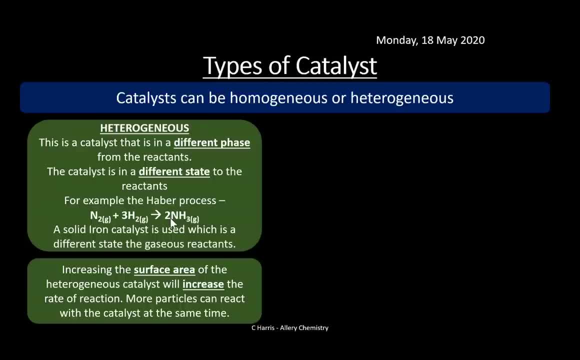 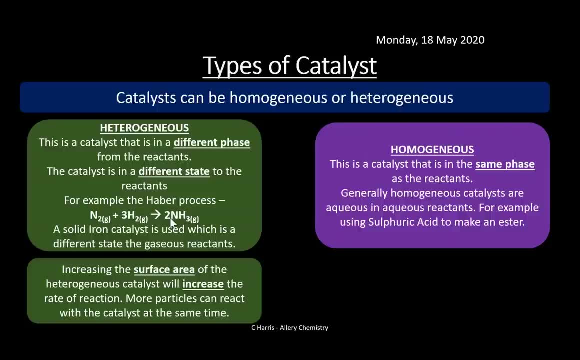 happen on. so a ground or powdered catalyst is going to be much, much better than just a solid lump catalyst- okay. so homogeneous catalyst- so these are catalysts in the same phase as the reactants. so homogeneous- okay. so these are catalysts that are normally an aqueous solution, so they're dissolved. 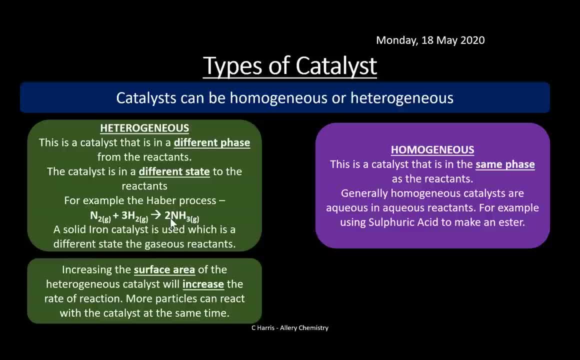 within within the solution um, so, for example, to make an ester. you might have done this in the lab again and making an ester. we use sulfuric acid as our catalyst. we add sulfuric acid in there and that helps to make our ester. and we remember you make an ester. 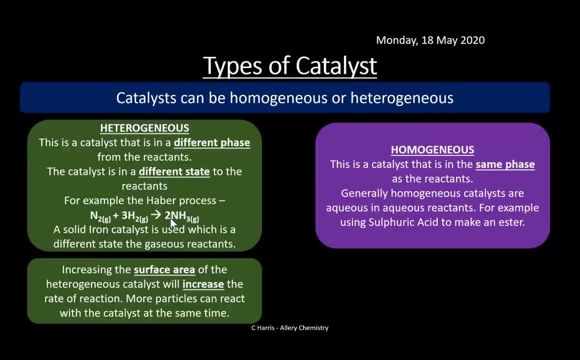 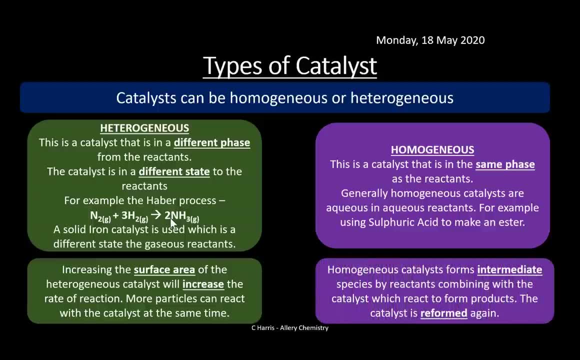 and by reacting an alcohol with a carboxylic acid. okay, so just a bit of orgasm, organic chemistry there. okay, so homogeneous catalysts, and like heterogeneous, these actually form an intermediate species. they really get involved with the reactions here and they actually, um the the reactions actually combine and react with the catalyst. but the crucial thing the most: 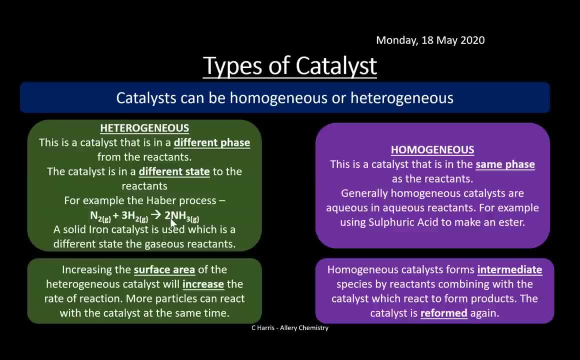 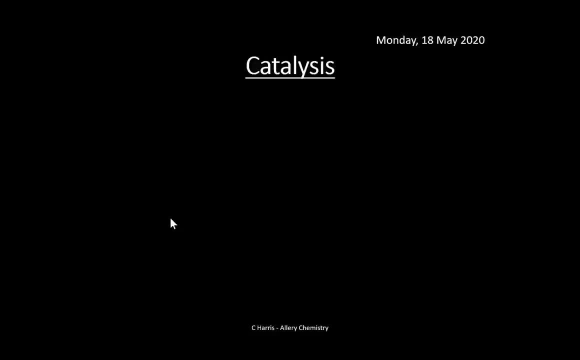 important thing with a catalyst is it's always reformed. the catalyst is never used, okay, never used up. you always reform a catalyst. that's how you can tell if it's a catalyst, okay. so um, transition metals? because they have variable oxygen levels, they're not going to be able to. 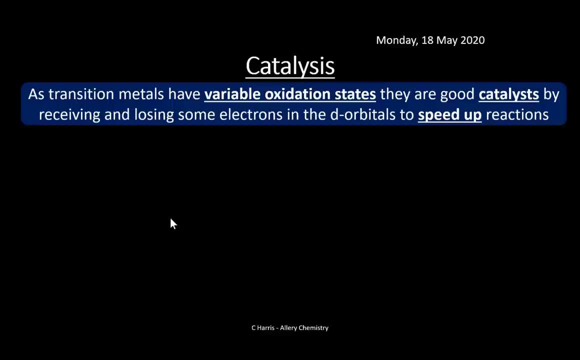 react with respect to the rate of oxidation states. they are actually really, really good catalysts, and catalysts are vital industry because it allows us to make things with lower energy, so that's better for the environment and also allows us to make it quicker as well. so we're not waiting ages and 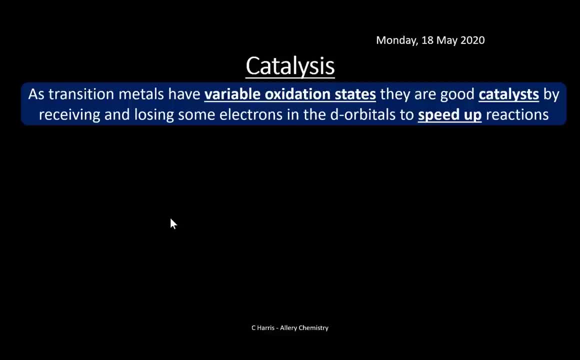 ages to produce these products. so, um, transition metals are really good at catalysts because actually they're really good at receiving and donating electrons in the d orbital, and this really allows them to be quite versatile within a reaction and hence that can speed that up. so this is why, in fact, we've got an 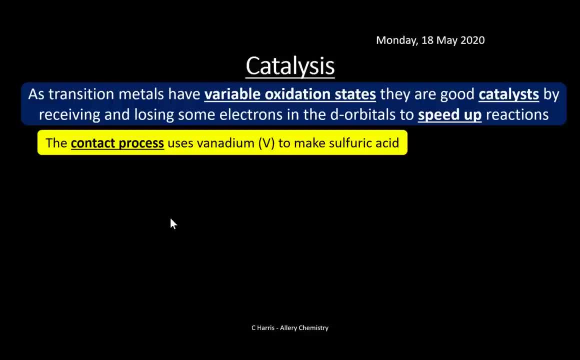 erotic reaction. that's pretty much the system of fasterście that we're really interested in. we're that up, so this is why transition metals are really good at this. so we're going to look at a specific example here, which is the contact process. okay, so the uh, the contact process. 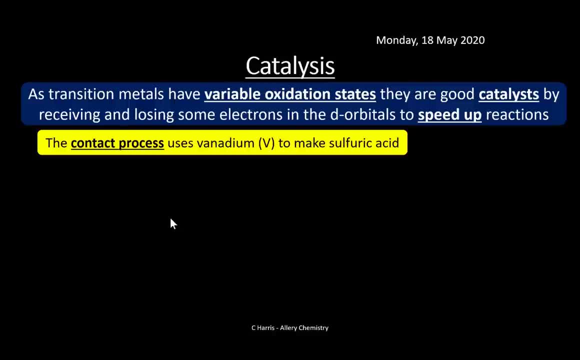 uses vanadium um, so vanadium 5, to make sulfuric acid. now, i love the contact process because i actually, years and years ago when i went to university, um, this is one of the areas that i um that i researched as part of my research project- was was the contact process of using 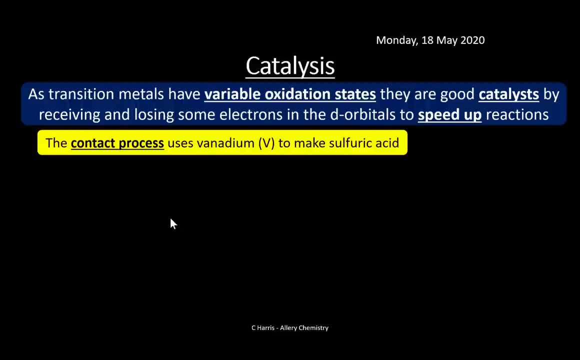 transition metals for drugs, but also um the contact process. so yeah, yeah, i think i went on a um a trip as well, to um a bp- i don't know if they still make it anymore, but uh, bp um to see how they actually do this. so this is that. so, yeah, so this has got a little bit of a connection with me. 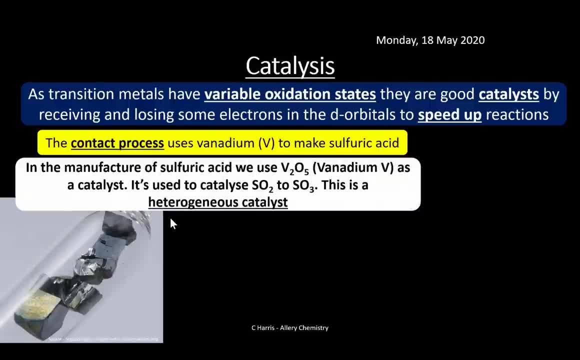 personally, but anyway. so the manufacture of sulfuric acid. sulfuric acid is a massively important bulk chemical. it's cheap, okay, compared to other fine chemicals like pharmaceuticals. sulfuric acid is made in bulk and it has to be made as cheaply as possibly can. and catalysts. 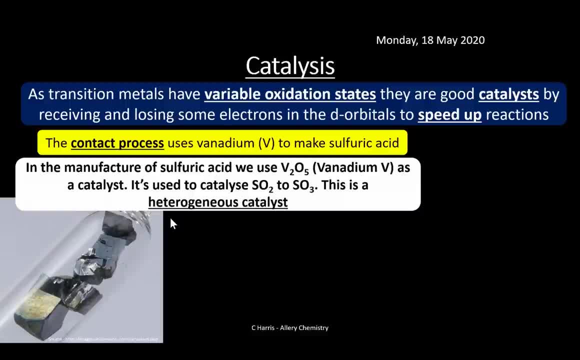 play a vital part here. so for the manufacture of sulfuric acid, we use vanadium 5 oxide, so v205 as the catalyst and it's used to catalyze so2 to so3, and this is a heterogeneous catalyst. okay, so where we obviously the catalyst is in a different phase to the reactants and products. 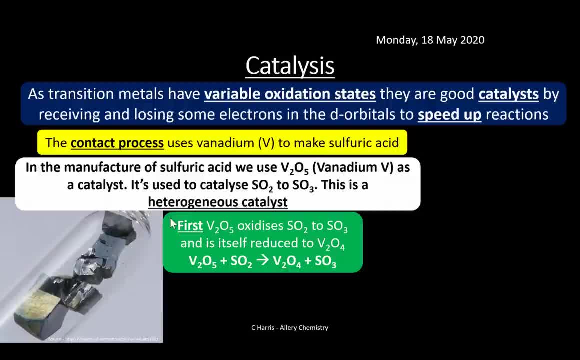 so, firstly, um, the v205 oxidizes so2 to so3 and itself is reduced to v204. so you can see here that we've produced our so3 here, fine, okay, this is our catalyst. so remember, in our second step we must be reforming this back again because it's a catalyst indeed. this is what happens. so the second step is that 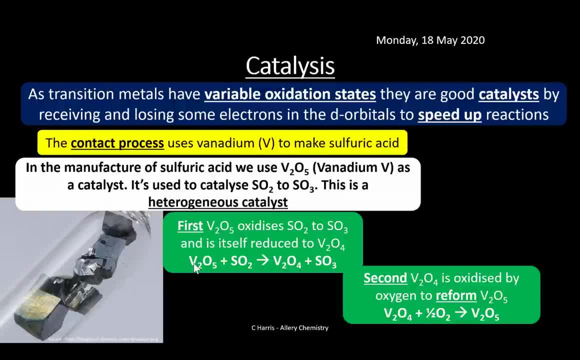 v204 is actually oxidized by oxygen, that's, that's just in the, in the atmosphere, and that reforms the layer of earth, and then it gets potentiated, okay, so what happens then is that that processes this catalyst again. okay, so remember, catalysts are vital, um, you know, for the, the, the transformation, 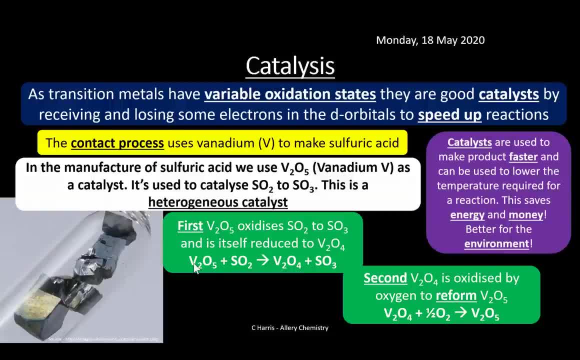 of chemicals and making them as quickly as possible and reducing the amount of energy you've acquired, which is basically what this is saying here. so it allows us to make it quicker, saves time and money and saves energy, so it's best for the environment. and the so3, by the way, is then bubbled just for. 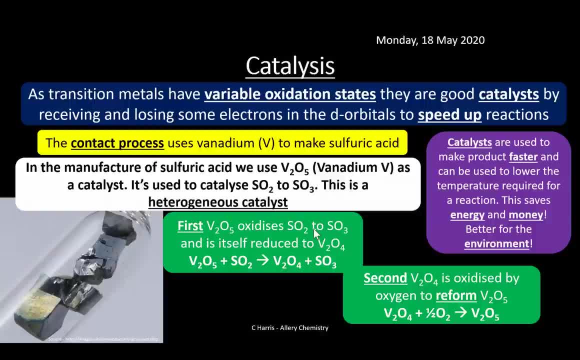 um to make h2so4, which is your, which is your acid. so so that's just showing the process which you make sulfur trioxide, which is then used to make your sulfuric acid. the catalyst only gets involved in making the sulfur trioxide in the first place. okay, so that's a specific example. you do need to. 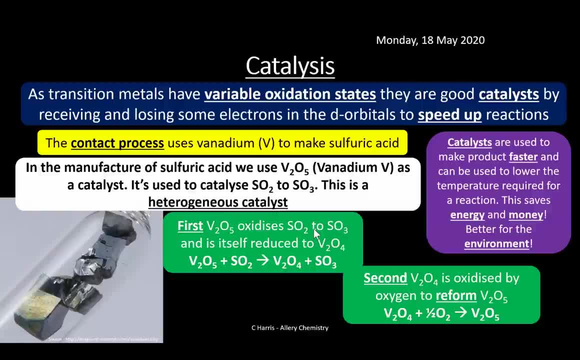 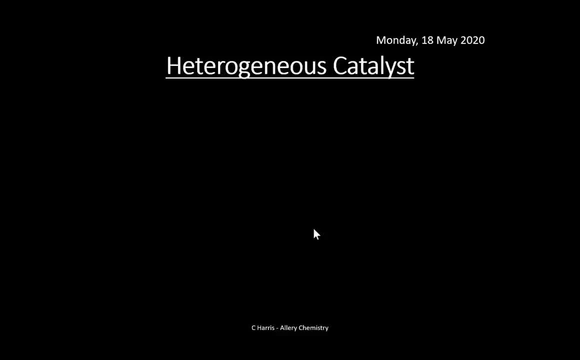 know about the contact process. you need to be aware of that. so this falls into. the vanadium member said they wanted to know a lot about vanadium chemistry. this is where it fits in within the contact process. okay, so the problem with heterogeneous catalysts is, although they're 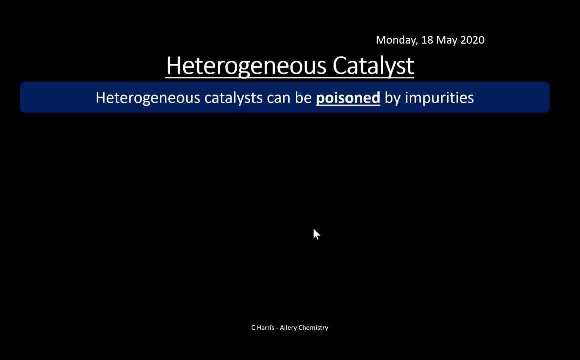 pretty good at obviously speeding up the reaction because they're solid and, in a different phase, they are liable for being poisoned by impurities. so, impurities, what these do is these bind to the surface of the catalyst. remember, these are like solid surfaces and these block active sites and 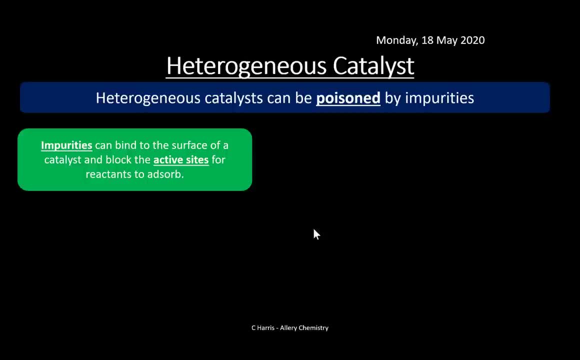 the active sites is where reactions happen. now, if we've got a solid catalyst blocked up with these catalysts, then we've got a solid catalyst, and we've got a solid catalyst and we've got a. you're not going to have many sites left to actually conduct your reaction with, and if 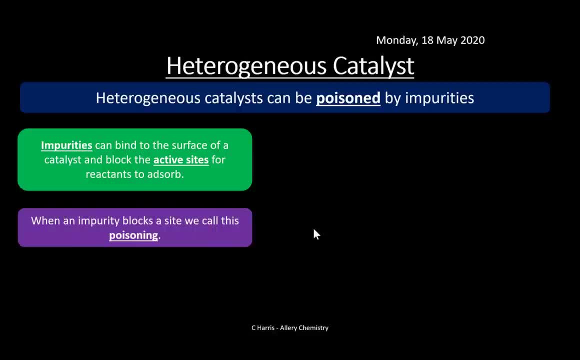 that's the case, then your catalyst is effectively useless. it doesn't really work. but when an impurity blocks a site, we call this poisoning- it's been poisoned, okay. so catalytic poisoning reduces the surface area of catalyst and this slows down the reaction overall. so, for example, if we look at the 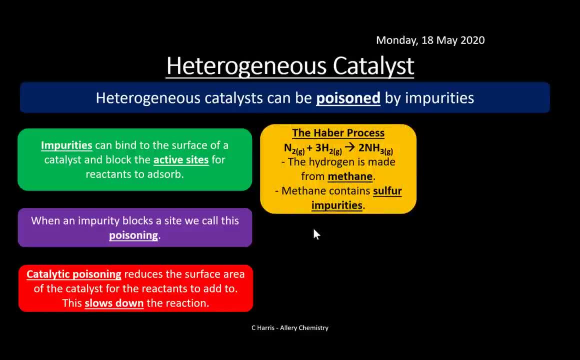 Haber process, just like we've seen before, and the hydrogen is made from methane. and the problem is, methane contains sulfur impurities. this is like any type of hydrocarbon or fuel. they generally contain sulfur inside them because these are, these are natural products and that sulfur can form you. 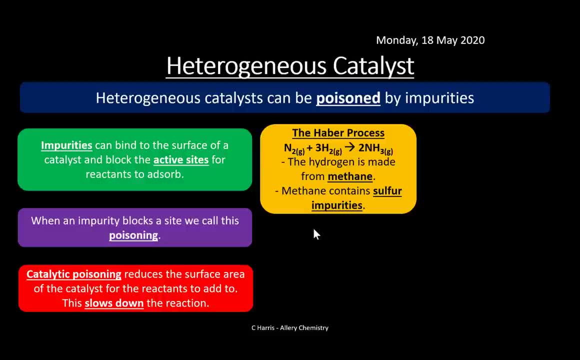 know, can have a bit of a problem. this is why, when you burn a petrol, let's say, you do get sulfur dioxide produced, because the sulfur naturally occurring in these fuels. so no different for methane as well. so so i'm going to diagram and you can see here that we've got a sulfur dioxide. 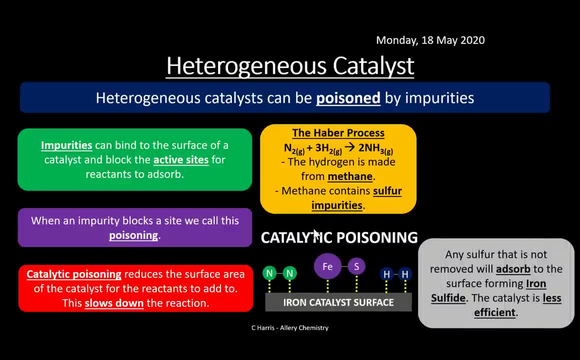 and we've got our iron catalyst surface in for the Haber process, because we use an iron catalyst here and you can see we've got nitrogen, we've got nitrogen hydrogen. this is what's supposed to be there. but then you've got this iron sulfide molecule here, because sulfur is the impurity. 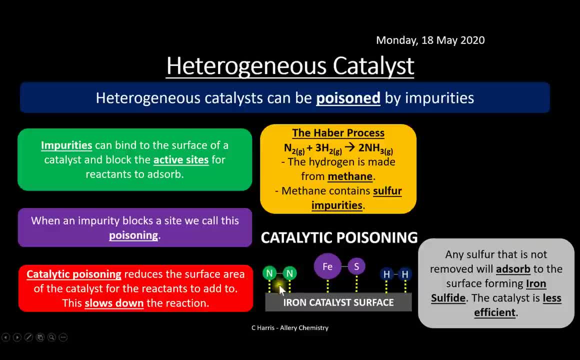 now that is blocking that site. so nitrogen hydrogen could bond here. but if you have imagine, if you had loads of these dotted around, there's not much space for the actual reaction to happen. so this is we say: this has been um, this has been poisoned the catalyst surface and we've got a. 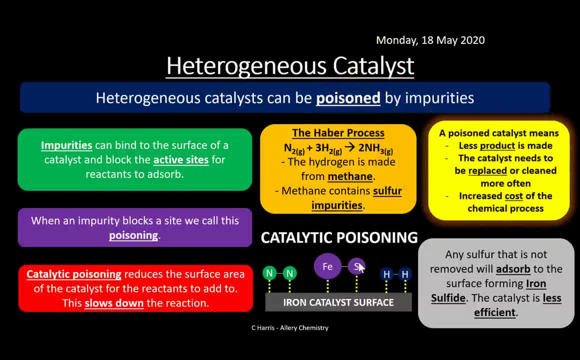 lot of this has been poisoned. it's not as efficient, and so a poison catalyst means you're not producing as much product. um, it needs to be replaced more often or cleaned. um. that increases the cost because then you need to get that out of the machine, get it cleaned, put a new one in. that means you may have. 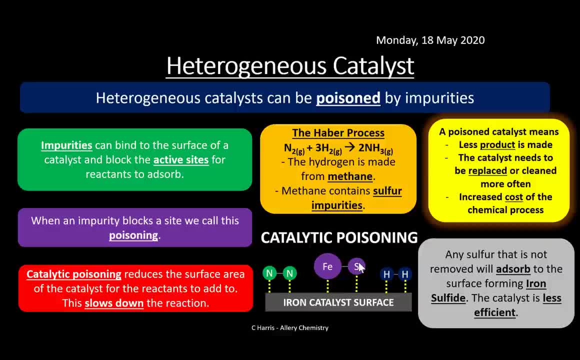 to shut down the process for a day or two days to get that changed, so that increased costs. so you've got to be very mindful of that. okay, so that's an example of a heterogeneous catalyst. you can see it's pretty straightforward: solid surface there and we have reactions adsorbent to the surface of that, allowing a reaction to. 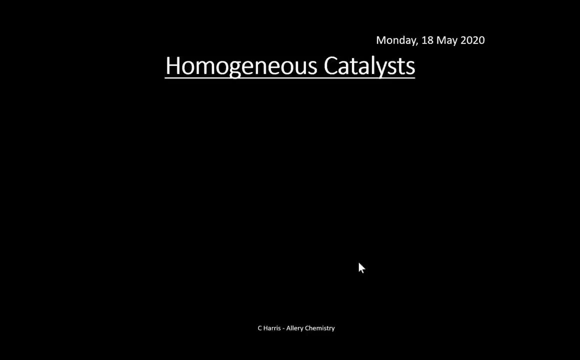 happen. so now we're going to look at homogeneous catalysts, and homogeneous catalysts have a very different approach because actually the chemicals for these catalysts actually get involved within the reaction and produce an intermediate. okay, so remember when you did your energy profile diagrams in year one. we're going to bring these back here to try and explain what a homogeneous 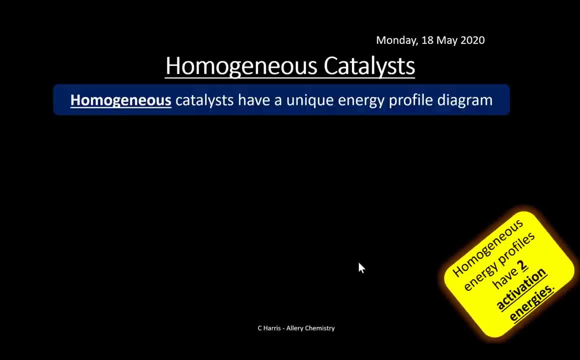 catalyst does so. homogeneous energy profile- um for these types of catalysts they have two activation energies. so here's your diagram. you might be familiar with this. so remember, you've got a reaction, reactants and products and you have a profile like that, okay, and the difference between the reactants and the um, the top of that peak there. 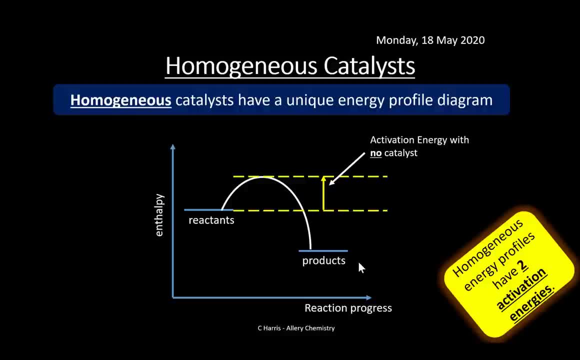 is the activation energy. that's the minimum amount of energy required for reactions, for collisions to occur and for successful collisions to occur, for a reaction to happen. so this dom here and then here the activation energy plus the carbonyl acid comes up with the activation energy. so that то is basically your score. you basically have a hematomimb關係. 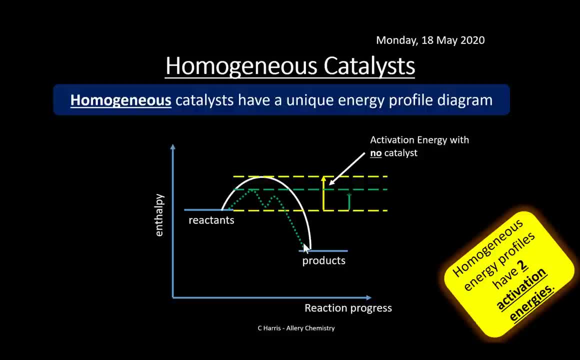 to the argon and then the casual reaction. so you notice, exercise player a little low. um, so, that's like theары k, that's�끄. we use to effectivelychet an activation energy in some kind of uh which uh Ind shields, and it calms it down. um, so, that's um, so obviously what? 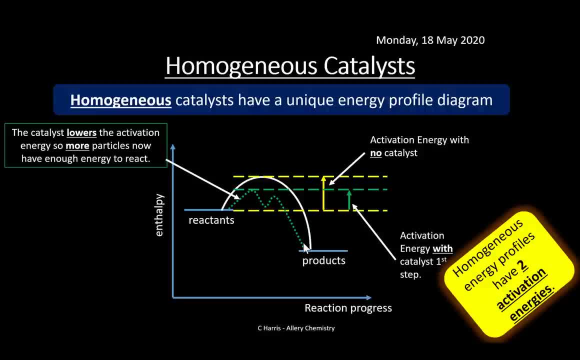 for successful collisions to occur, and so that's fine. but, as you can see, we have a second bump here. so this is the activation energy with the catalyst in the second step. so we have two activation energy lines here, and so the intermediates are formed in that dip in between. okay, so you can see that with. 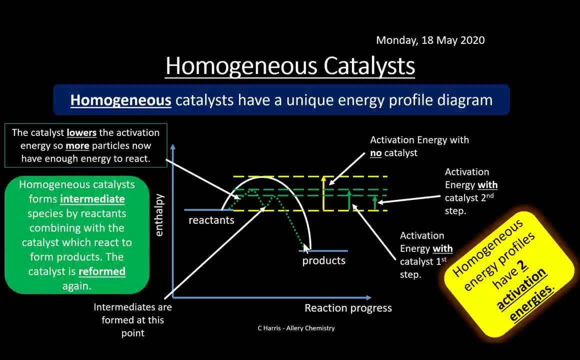 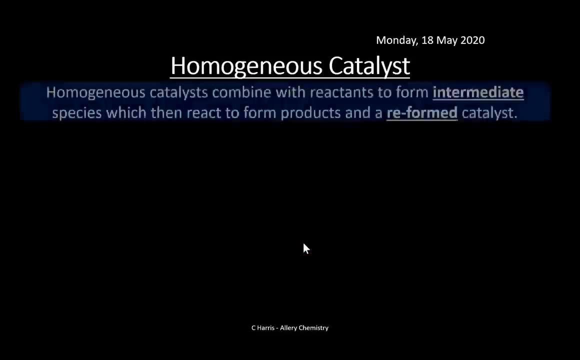 homogeneous catalysts. they form this intermediate. they actually combine with the reactants in there, get fully immersed within the reaction, but crucially, they are reformed back again at the end. so you can see we have this intermediate. let's look at a specific example here because I think it's easier. 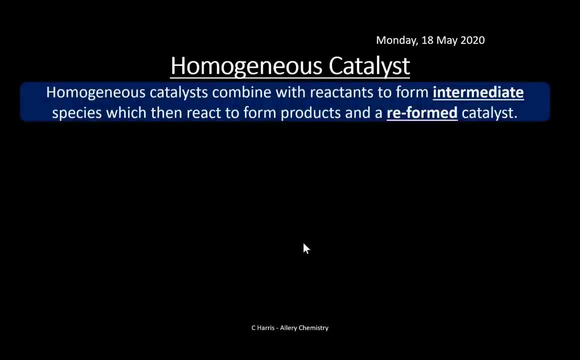 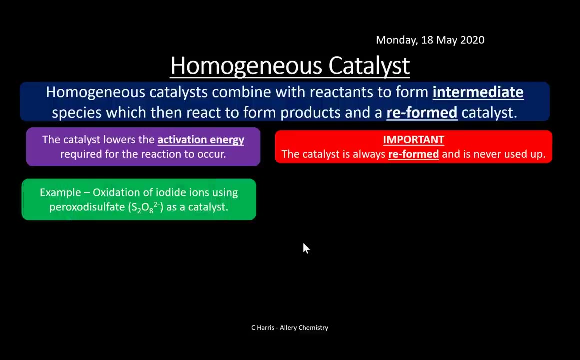 when we see it in an example form. okay, so remember, these catalysts, combined with the reactants, form an intermediate and then reformed so the catalyst reduces the activation energy required for that to happen. remember, they're always reformed at the end. so let's have a look at a specific example. so, oxidation of iodide ions using peroxyl. 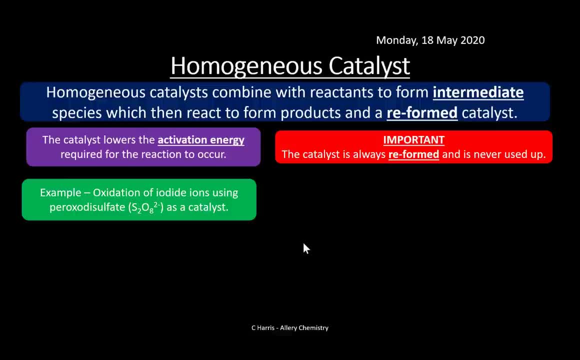 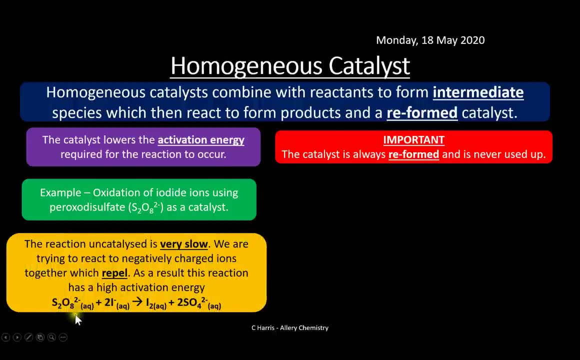 disulfate as a catalyst. okay, now the first thing you probably notice is that hang on, you're trying to react here. you're trying to react an I- with an S2O2- now, try and react these together really, really hard, because they're both negatively charged. they don't want to be. 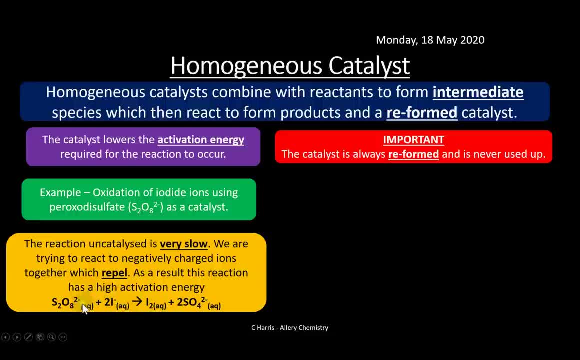 anywhere near each other. yet how on earth do we try and get these two here to react so we can produce our product, which is iodine? well, this is where a catalyst actually works here. so this is a homogeneous catalyst we're going to use here. so this is an incredibly high activation energy because obviously, the 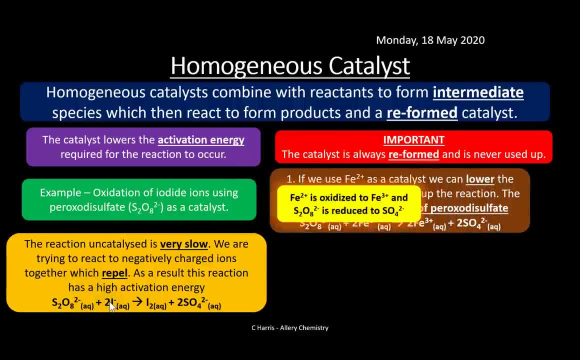 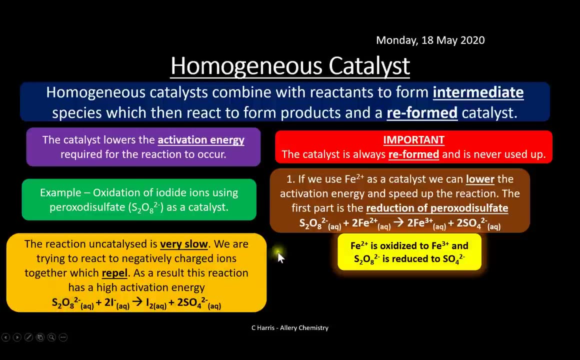 two negative charges. so let's have a look. so we're gonna use Fe2 plus solution as a catalyst. it's all in the same phase. this can lower the activation and speed up the reaction. so the first thing we need to do is actually take the disulfate, this iron here, react it with our catalyst and we form fe3 plus and then we form our so42. 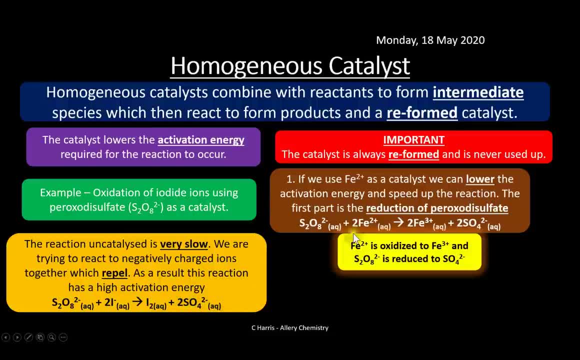 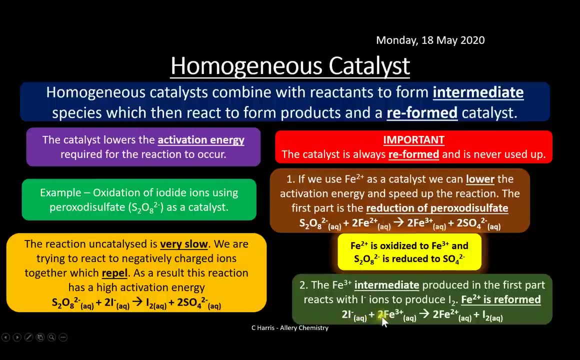 minus and look, we form one of the products immediately. okay, so this fe2 plus is oxidized to fe3 plus, and obviously this has been reduced. and so then- this is a clever bit- that fe3 plus then reacts with um, the i minus ions, and the fe3 plus then reverts back to fe2 plus. remember it. 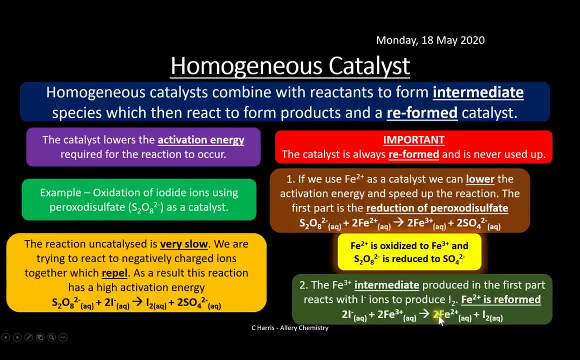 must be reformed. this was our catalyst at the start, so it must be reformed as a product to here, and obviously that then converts the i2. so what the catalyst is doing is it's actually breaking up. it's doing the first bit first, first forming the first product, and then it's forming the second. 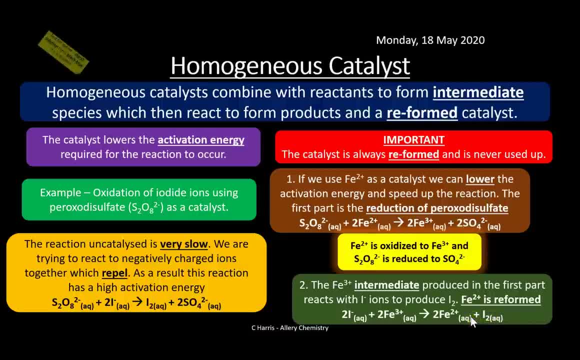 product later on. okay, um, so you can see that. the test for iodine, remember, because obviously this is, we're producing iodine, is we? if we put starch in this reaction and we get a black color if there's iodine present, we get this deep black color if iodine is present in this reaction. okay, very important, you can see we. 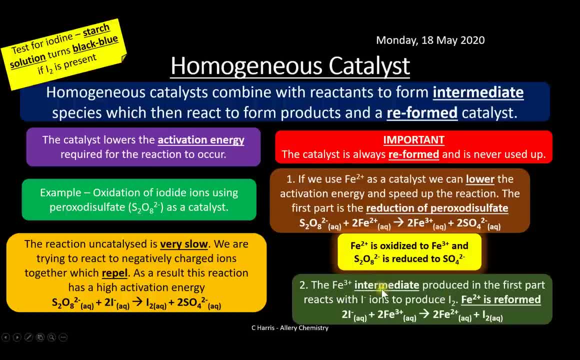 formed this intermediate. okay, so the fe3 plus intermediate. remember, on that energy profile diagram, we've got that dip in the middle because we've formed the intermediate here, but crucially, it's always reformed back again. okay, you need to know this specific example for aqa. okay, so make. 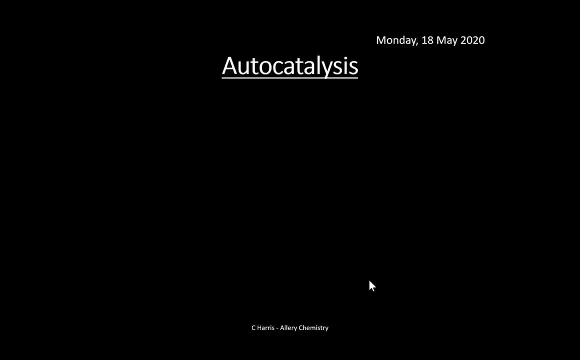 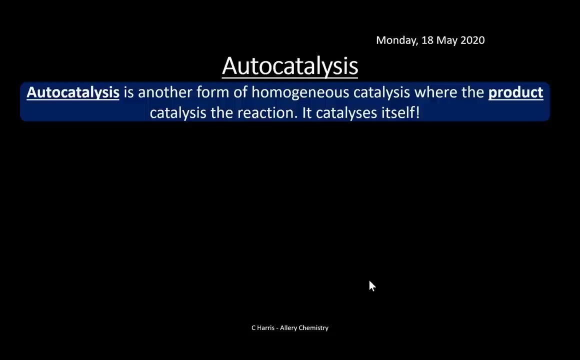 sure you're aware of it. okay, so just coming on to the the last bit now, uh, which is auto catalysis. this is so cool. auto catalysis- this is where, imagine of all reactions are like this. auto catalysis is another form of homogeneous catalysis, but the product of the reaction is acts as a catalyst. it catalyses. 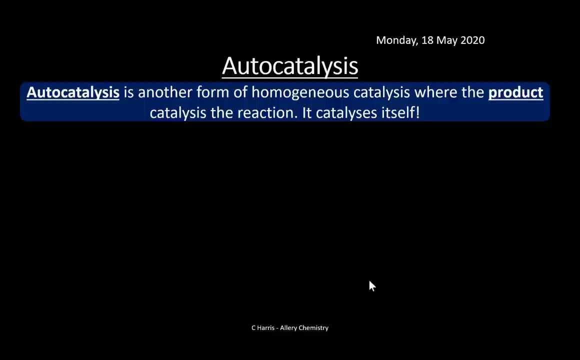 itself. this is just brilliant, this. so you do get some reactions where they do catalyze themselves. you don't even need to add anything to it to speed this reaction up. so a specific example here is where we've got manga- manganese two plus manganese two plus ions, mn two plus. 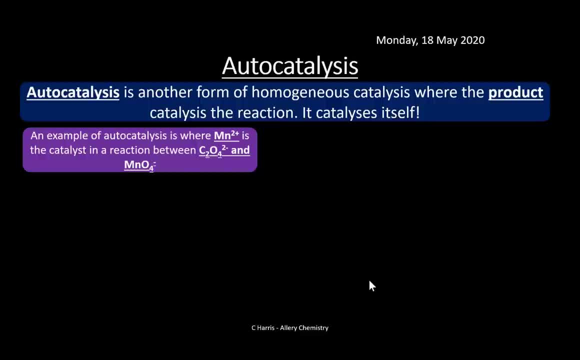 um is actually a catalyst that is being thrown out of the reaction. so we've got this one right here. uh, in a reaction between um, your c204 um and your mn04 minus ions. okay, remember again, you've got two negative ions there. they ain't going to react together because they're they're going to repel. so 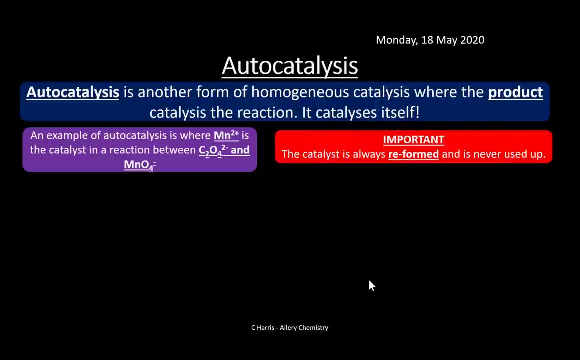 we need something to effectively- um, you know, help it, help it get along. so remember, a catalyst is always reformed. it's never used. i must emphasize that. okay, very, very important. so mn2 plus is a product and a catalyst. yep, i'm going to say that again, it is a product and a catalyst. okay, so it. 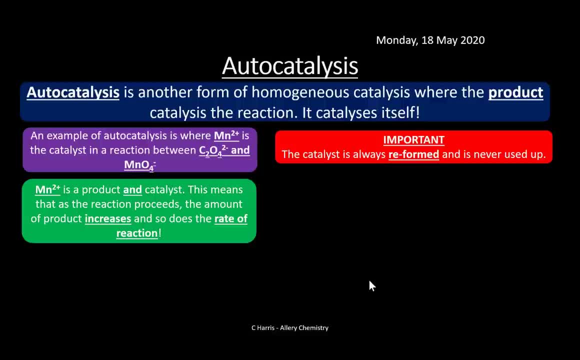 means, as the reaction proceeds, the amount of product increases and the rate of reaction increases. so initially it starts off really slow. it's a slow reaction, okay, um, and then it massive. it speeds up quite quickly, um, after that because of you producing more products, and it increasingly. 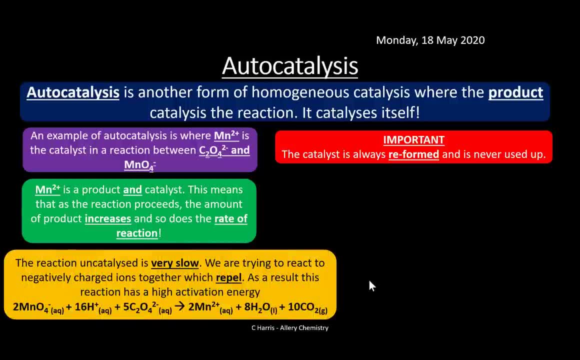 gets faster, so, uncatalyzed, this reaction is incredibly slow. remember, just like the previous example, we're trying to react to negative ions and we're trying to react to negative ions and negative ions together. that is really difficult to do. okay, they don't want to be anywhere near. 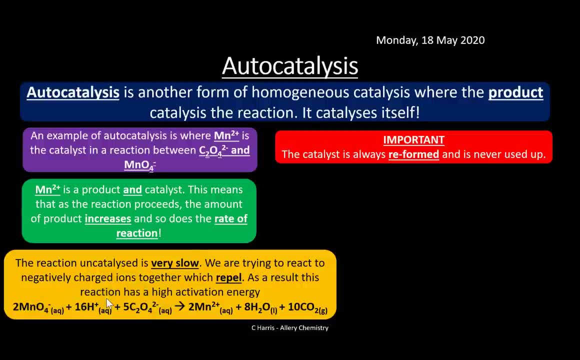 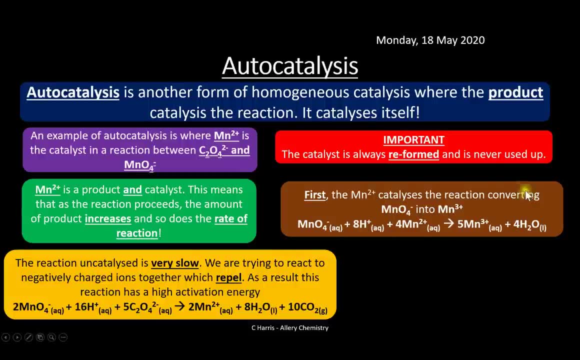 each other. they're going to repel each other, so we need this catalyst to work. so, again, it's a homogeneous, so it works in two steps. so the first step is your mn2 plus uh catalyzes the reaction and this con, this converts mn04 minus, this reagent, first into the mn3 plus, um, so uh, into mn3 plus. 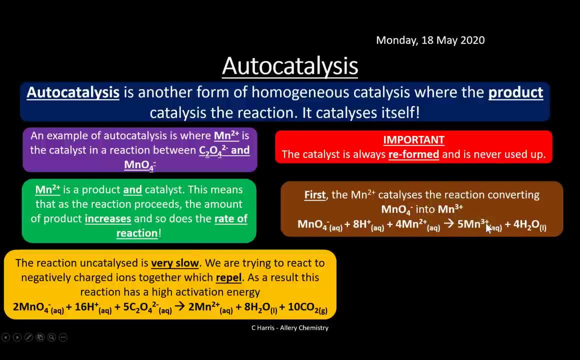 which is obviously one of our products here. this is one of the products we're producing, so that's the first, the first step there, okay, and then secondly, the mn3 plus that was formed reacts with the um c2042 minus and the mn2 plus. 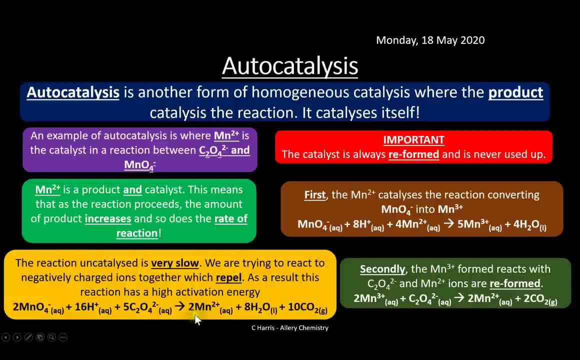 ions are actually reformed again, so we reform the mn2 plus there, it is okay. so that's one of our products, remember? that's what we want to produce, um, and obviously we're producing carbon dioxide as well here. so this is the overall reaction here, but you can see the product- one of the products is actually acting as a 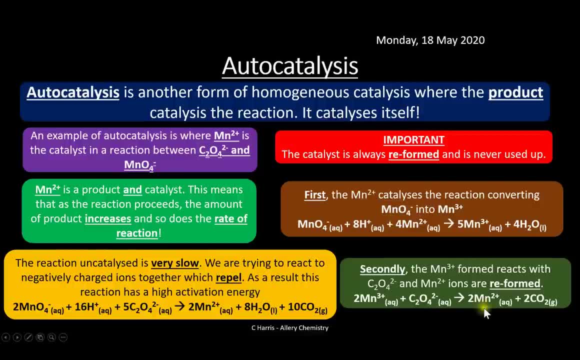 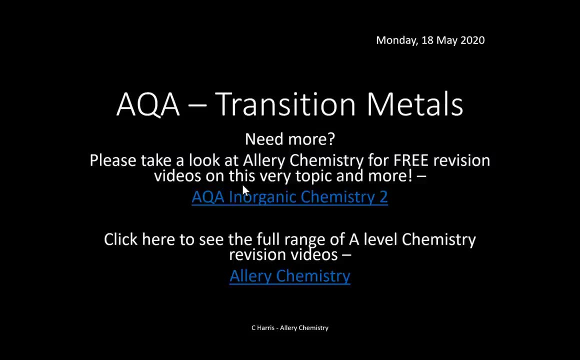 catalyst here, so it's been used up here and then reformed at the end here. okay, so it's an auto, it's auto catalysis, it's reacting itself. you need to know that specific example as well for aqa. okay, so that's it. okay, that was quite a big topic and there's a lot of stuff in there, loads of stuff. 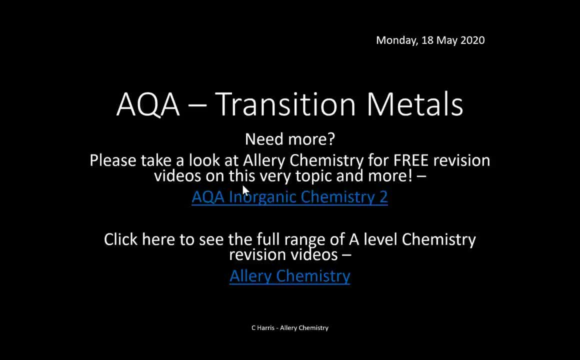 um, there is, like i say, this is not. this is obviously just one of the videos in a range, a qa videos from year one right through here through to year two, so it's fully comprehensive, as well as whiteboard tutorials and exam paper uh walkthroughs as well to improve exam technique. 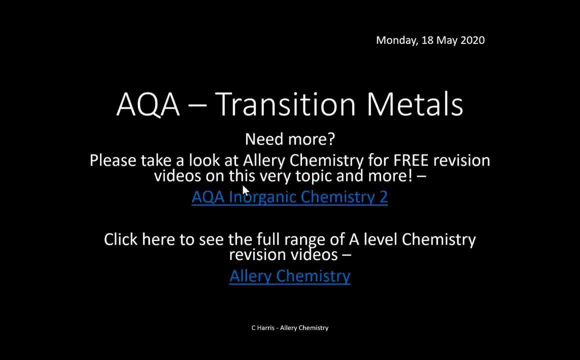 all i ask is that you hit the subscribe button. that'll be absolutely fantastic. there's no charge for these and i intend to keep it that way as well. all i need is just your support. so hit that subscribe button. that'll be absolutely fantastic. and if you do want, access your own private copy. 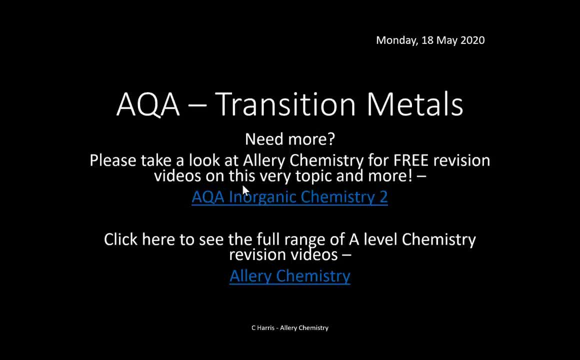 of these, then they are available to purchase great value for money. click on the link in the description box. phew right, that's it. i'm off to get a cup of tea, see ya.